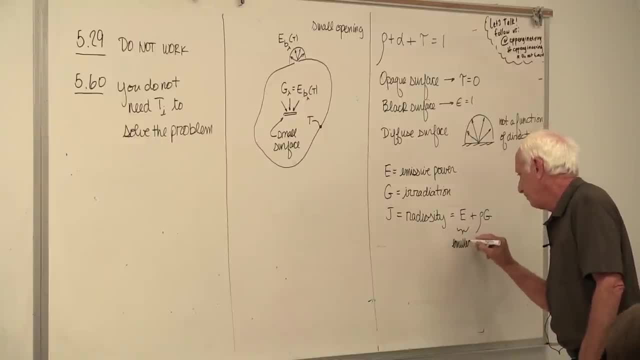 Plus there'll be some reflection from the incoming irradiation. So what leaves the surface Emitted plus reflected? Okay, now we talk about a black body. Is there a way to get something close to a black body in a laboratory environment? 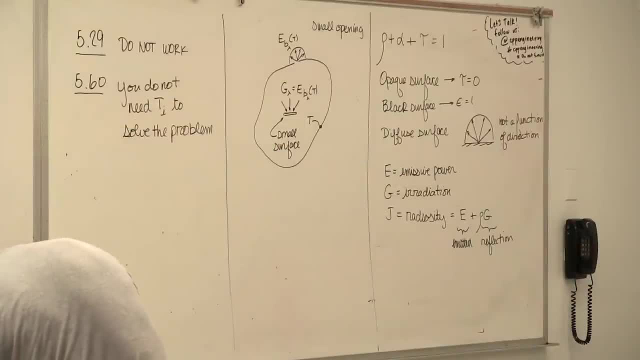 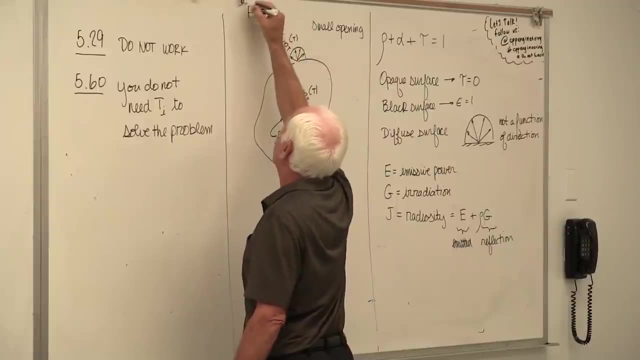 Yes, there is. It's on figure 1211.. You can look at that Figure 1211.. It's up on the board here, But in case you need to refer to it, that's where you find it. This is a. 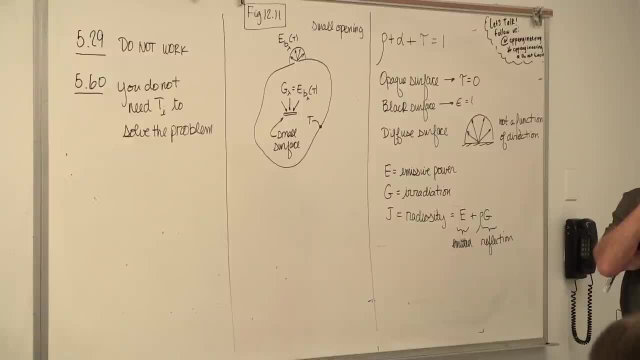 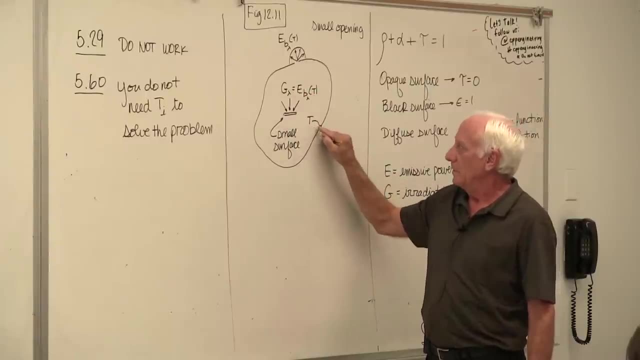 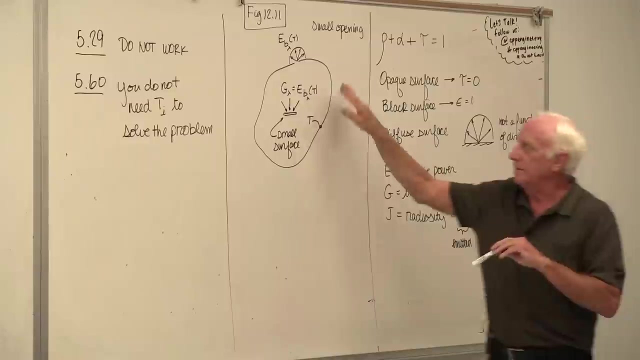 model of a large enclosure. The enclosure walls are kept at a temperature T. Forget the middle one, Just forget the middle part. There's emission from the walls in the enclosure. It bounces off the walls, It's reflected, It's absorbed, It bounces around here. 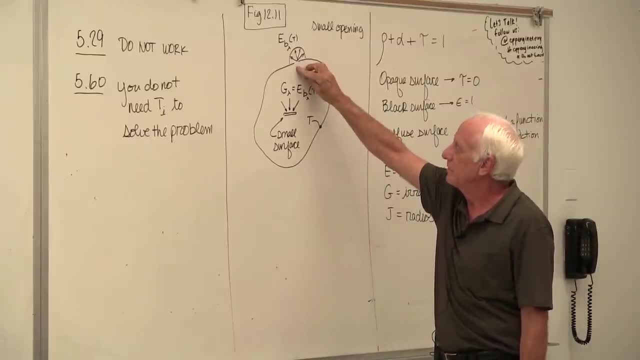 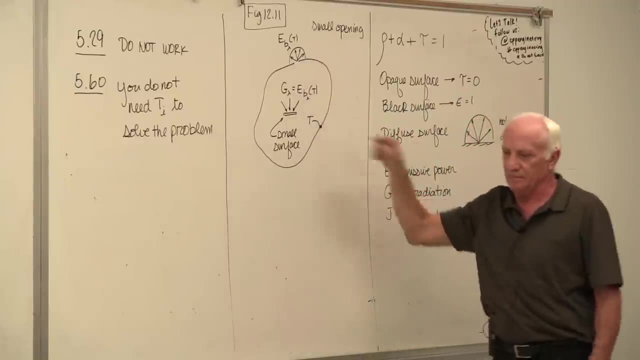 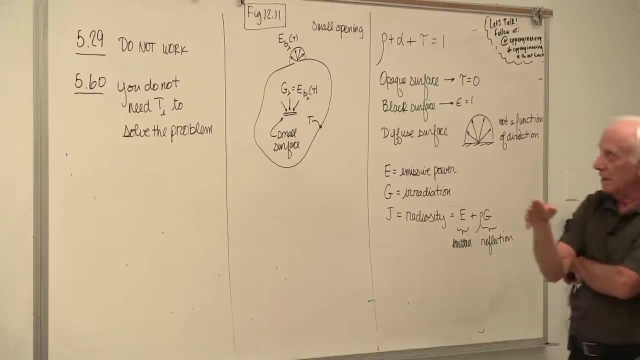 If you have a small opening in that enclosure, what leaves that small opening appears to have come from a black body at the temperature of the wall's T. That's one way you can approach a black body experiment, maybe in a physics lab A large object. 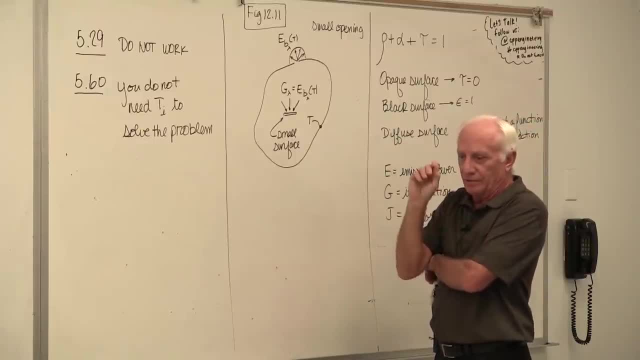 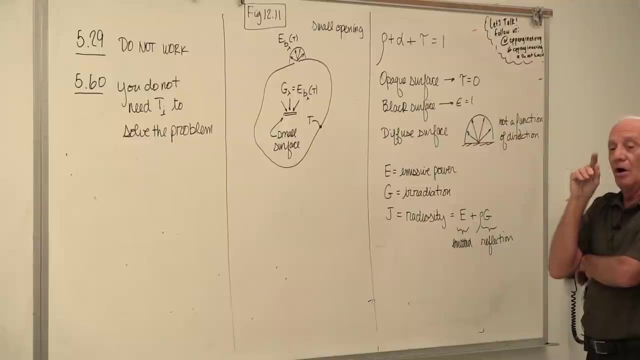 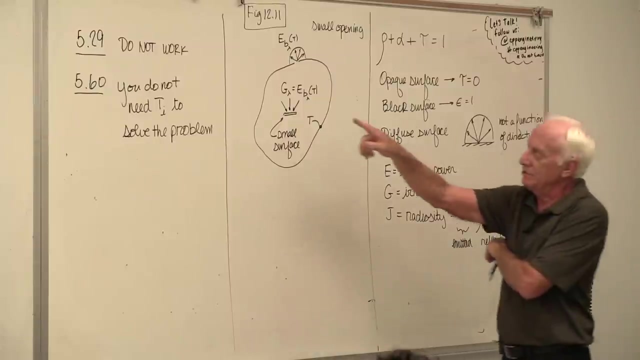 heat the walls, put a small hole in the wall. The radiation leaving that small hole has the spectral appearance of black body radiation. Also, if you put a small object in that large enclosure, the incoming radiation G looks like it comes from a. 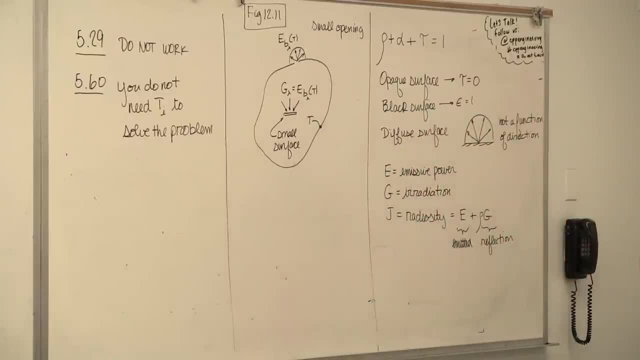 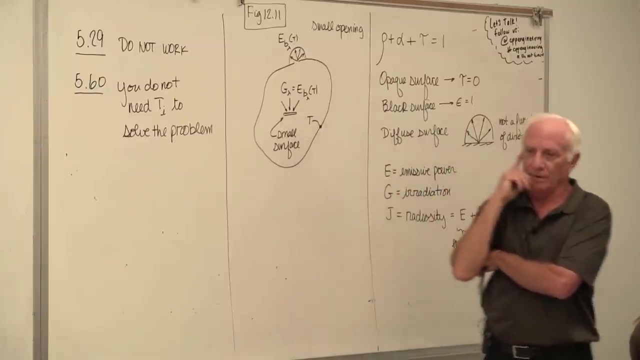 black body at the temperature of the walls. again, Not the temperature of the small object, The temperature of the walls. T Put a dime in a basketball. Okay, that's it. Small object: dime in a large enclosure basketball. 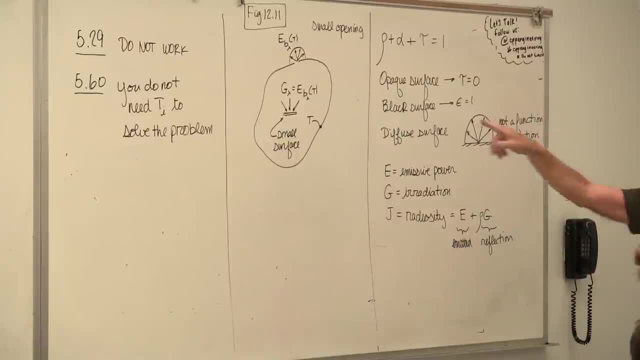 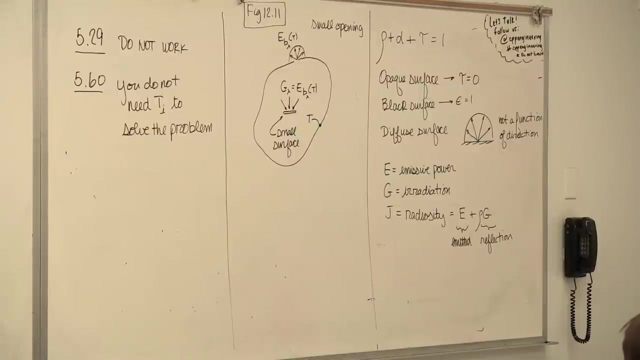 That kind of a scenario. Okay, we'll use this in a problem later on. Now, one of the last things in that area of definitions. we've got one more, I think. Let's see what it is. Yeah, here it is. 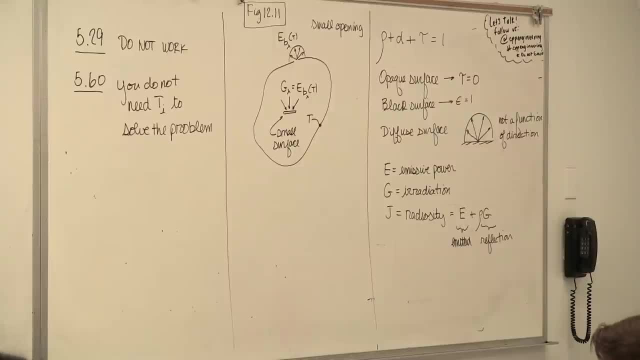 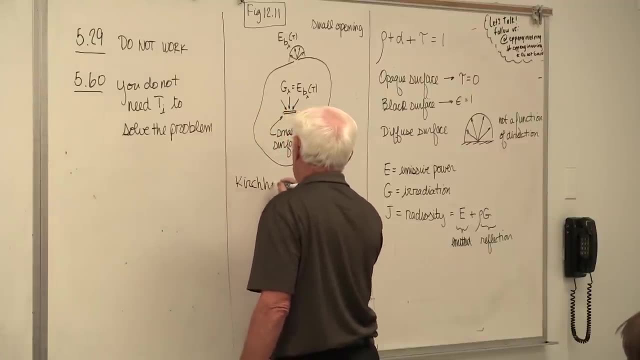 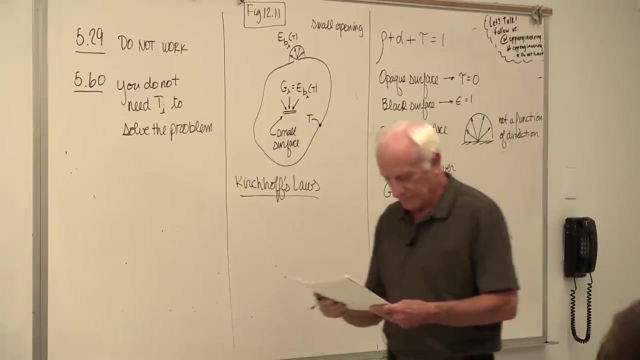 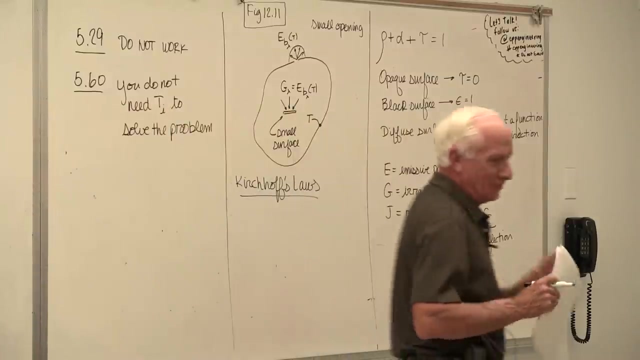 Okay, something, something called Kirchhoff's Laws. Okay, the first one of the Kirchhoff's Laws. There's really three, but I'm going to just do two. The third one's not that important for our class, so I'll just do two. 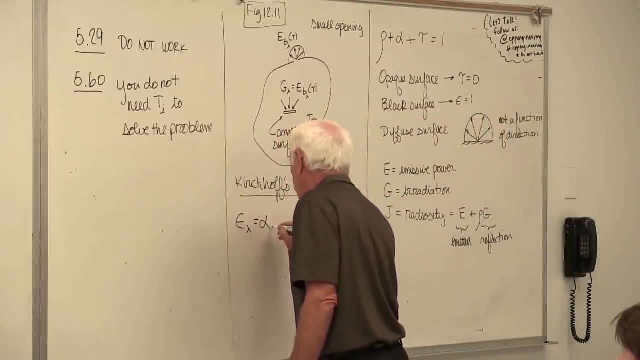 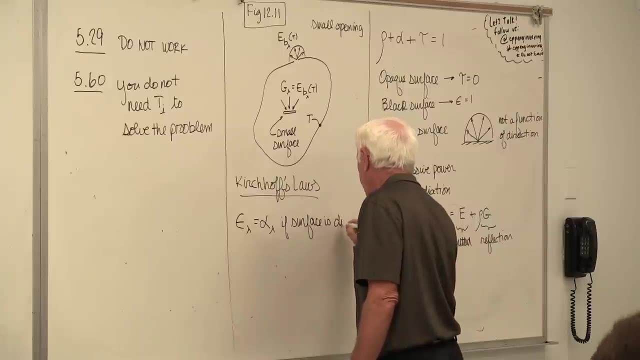 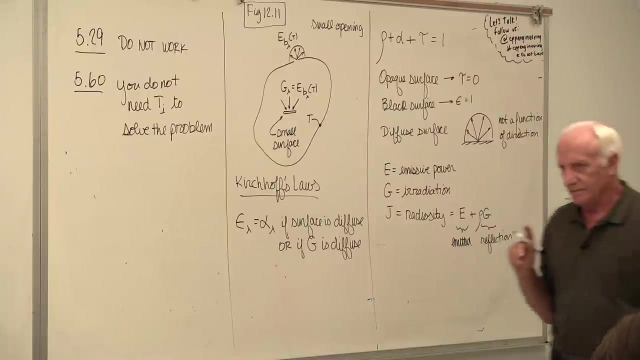 You can say that epsilon lambda equal alpha lambda if the surface is diffuse Or if the incoming radiation G is diffuse. He kind of walks you through it in the chapter. That's the first of Kirchhoff's Laws. The second one is: you can say: 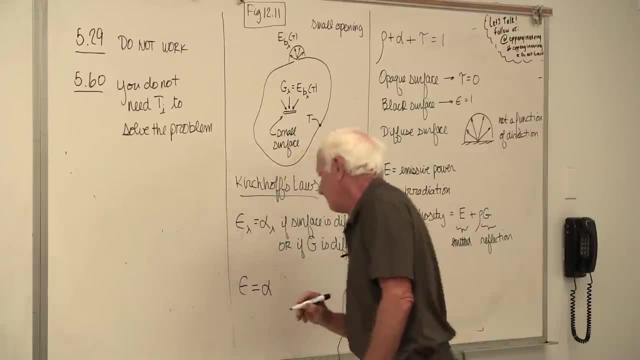 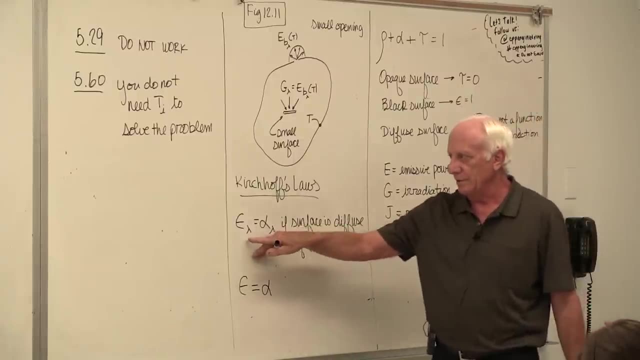 epsilon equal alpha. no lambda subscript, Don't forget. the lambda subscript means the word spectral. This is the spectral emissivity, This is the spectral absorptivity. Spectral means at a particular wavelength. What's the value of emissivity at a particular wavelength? 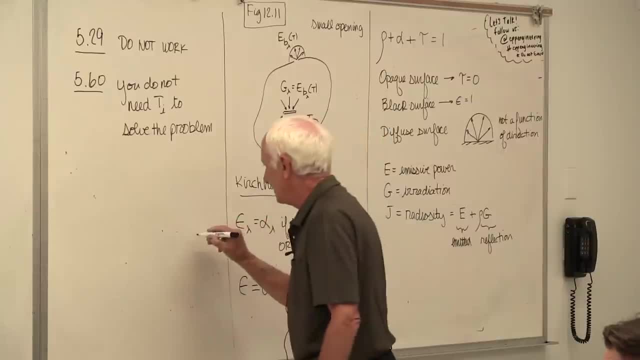 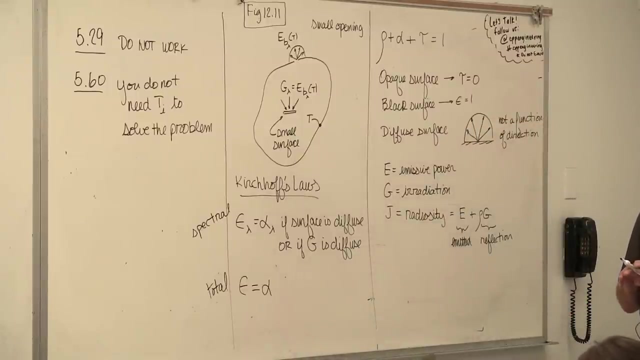 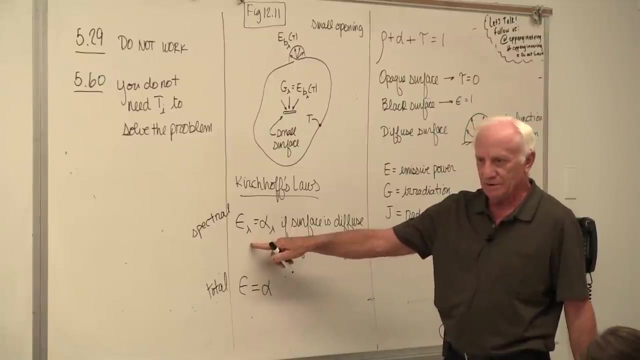 I'll put a note here. This is spectral. This is called total. The total emissivity equals the total absorptivity. The total means integrated over all possible wavelengths, zero to infinity. The total means integrated. You integrate epsilon lambda over all possible wavelengths. 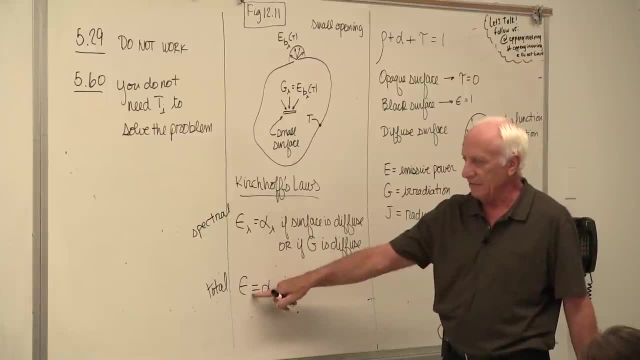 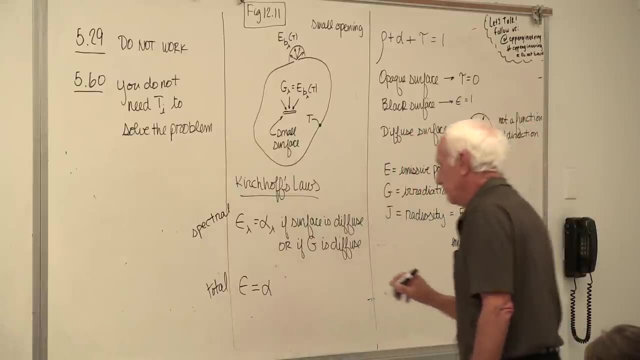 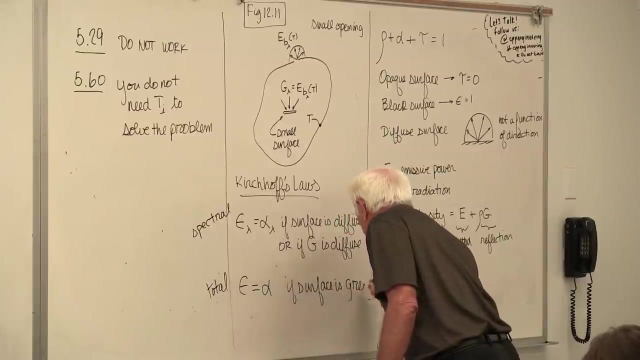 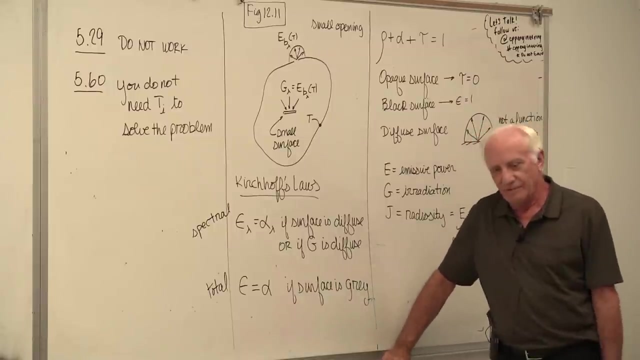 lambda equals zero to lambda equals infinity. That gives what we call the total emissivity or the total absorptivity. That's true If the surface is gray. There's another qualifier there too, If the incoming radiation appears to come from the same temperature. 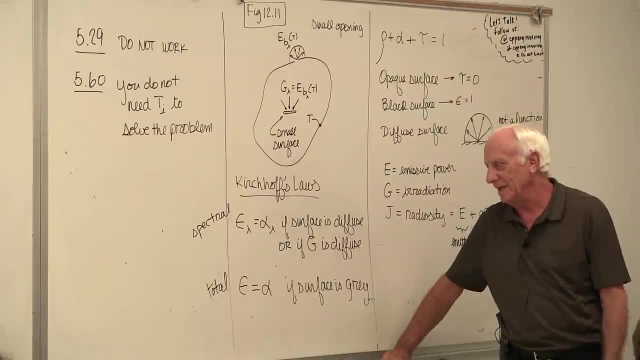 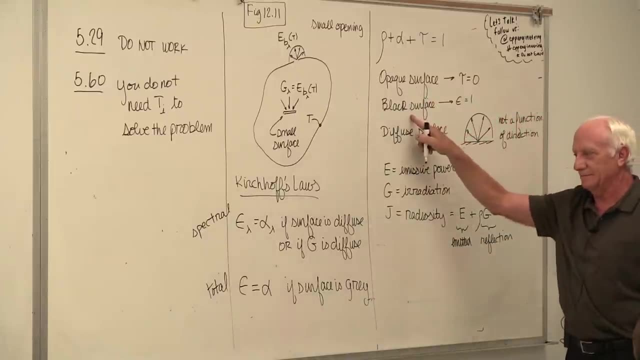 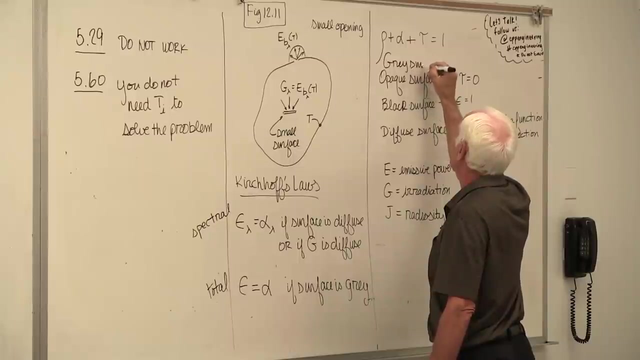 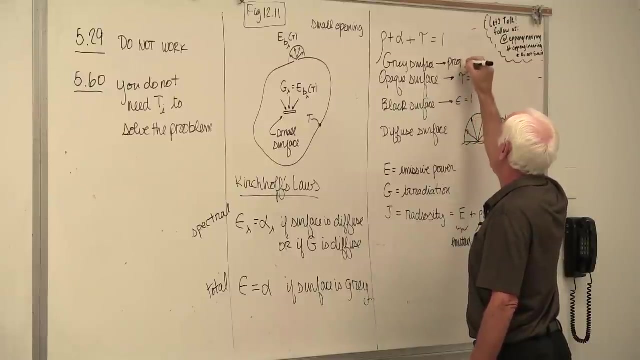 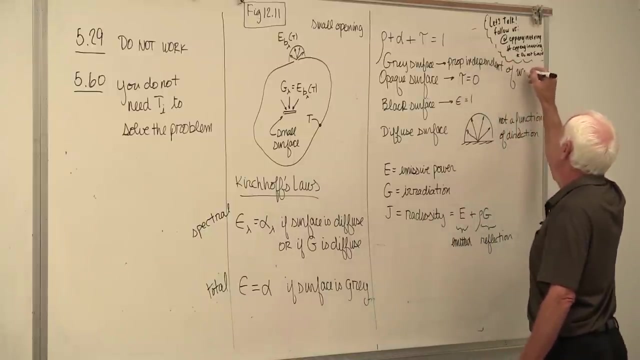 as the surface, but that happens rarely, so the one we're interested in is this reason: Okay, Opaque surface, Opaque surface, Black surface. Now we have another one, Chapter 12. Gray surface Properties independent of wavelength. 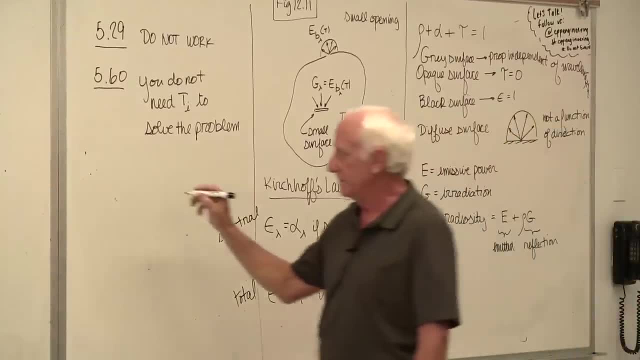 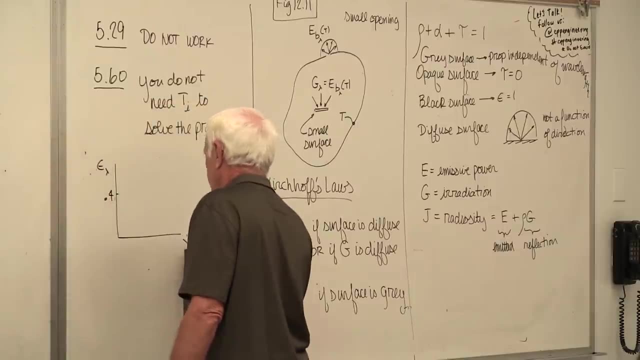 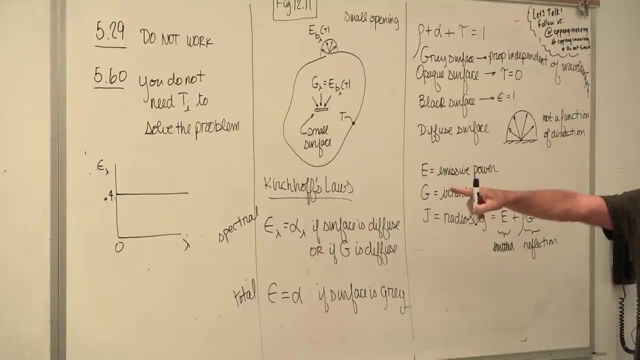 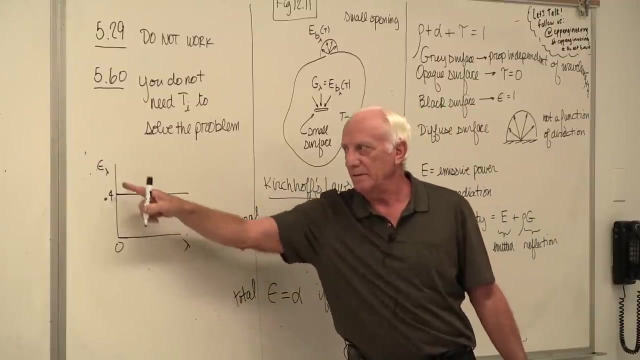 Properties independent of wavelength. For instance, here's epsilon lambda versus lambda. It doesn't depend on wavelength. That is a gray surface. Yeah, that's a gray surface. It might be alpha lambda. It looks like this. It might be rho lambda. 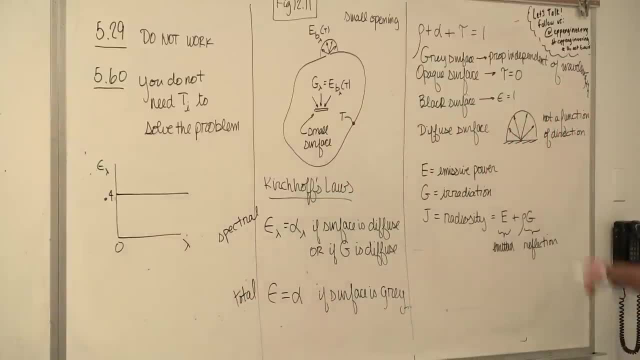 It looks like this: Properties epsilon, rho, alpha tau, Independent of wavelength. Okay, So Kirchhoff's Laws. Okay, I think that's about all we need. Yeah, Okay, Let's work. a couple problems using what's on the right-hand side of the board. 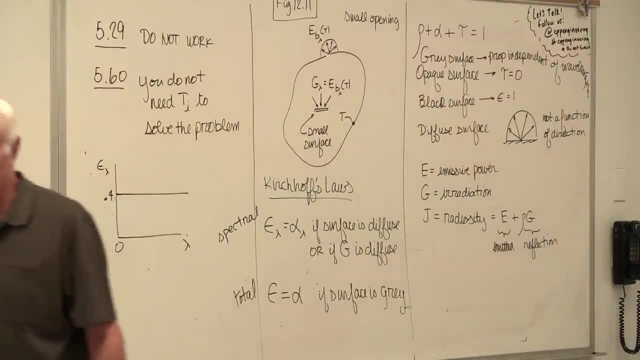 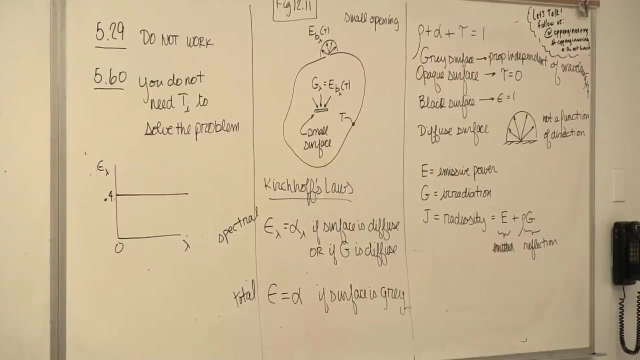 Chapter 12 is difficult to read cover-to-cover. You're much better off using the notes as a guide and filling in what maybe you need to fill in from the class notes in the chapter. But to read it cover-to-cover you won't sleep well at night. 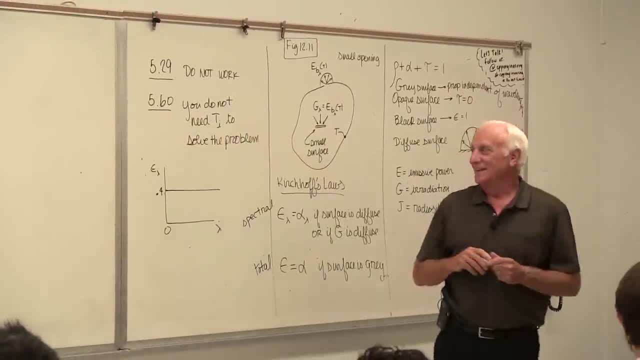 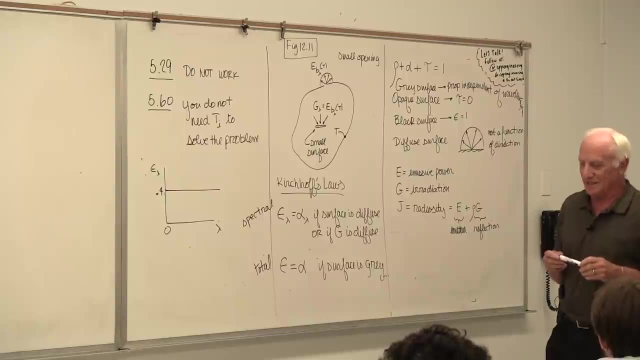 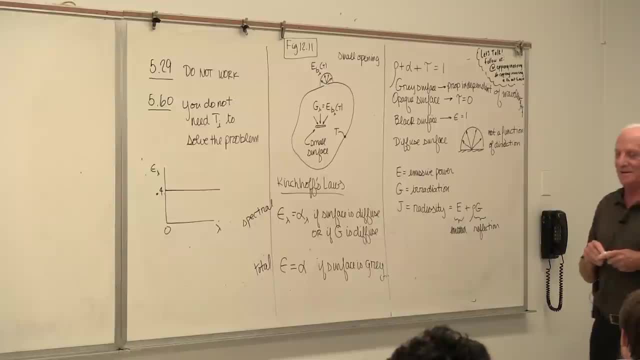 We had Planck's Law, We had the band emission, We had all that. So that was last time. Okay, So here we are this time. We're going to use this. now We're going to use this, And we're going to use this. 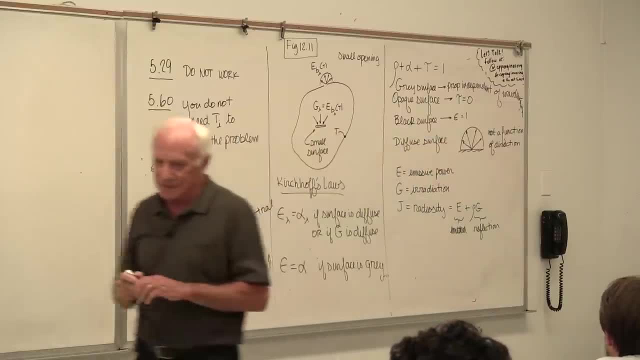 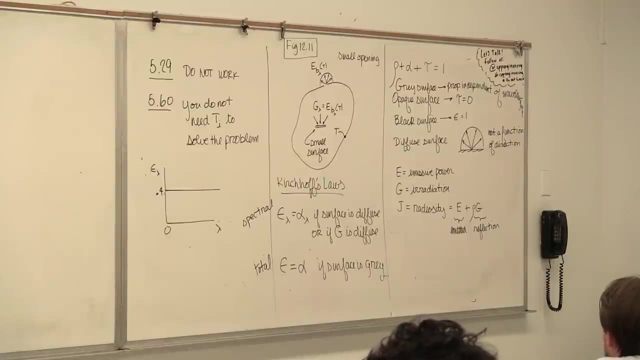 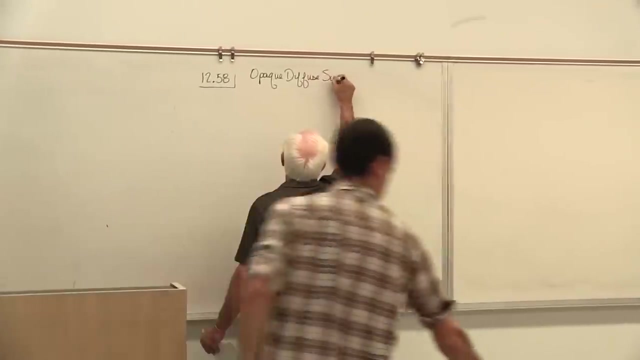 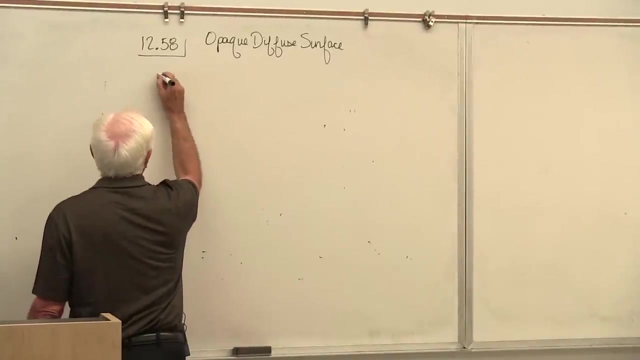 All right. So let's take a look at problem 1258.. It says that we have an opaque, diffused surface. It says we're given spectral absorptivity as a function of wavelength. Okay, Spectral absorptivity means alpha sub lambda. 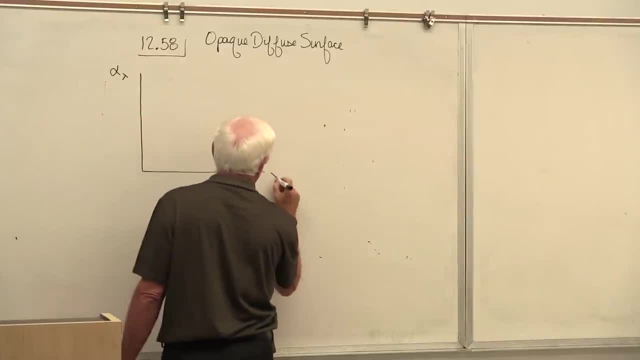 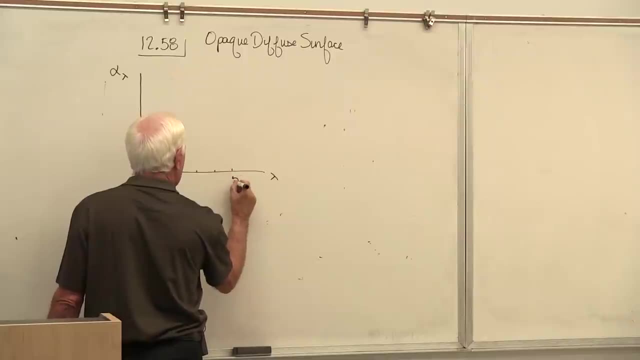 The lambda means spectral. As a function of wavelength lambda, We're going from zero to five, One, two, three, four, Five. One, two, three, four, Five. One, two, three, four, Five. 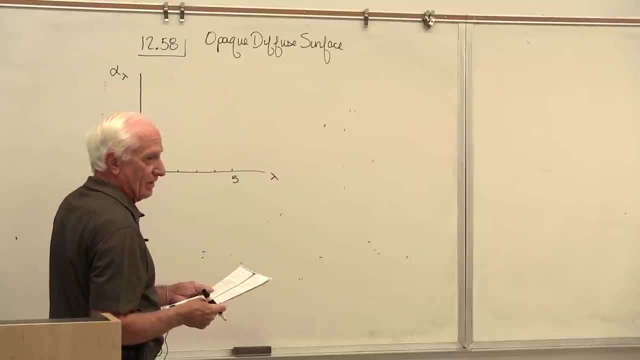 Five, From wavelengths of zero to two microns, wavelengths and microns. alpha lambda's point four. Okay, One, two, three, four, Five, six, seven, eight. One, two, three, four, Five, six, seven, eight. 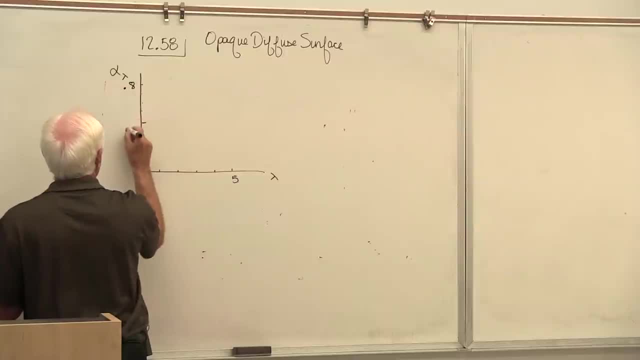 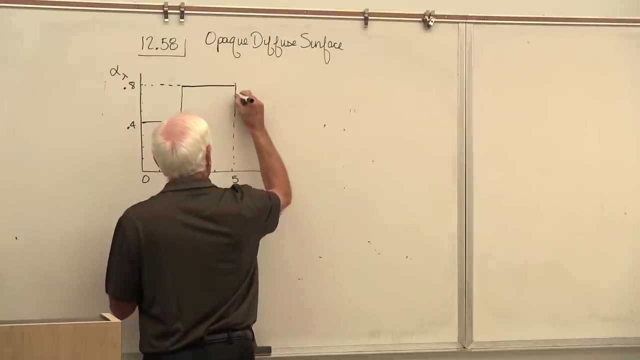 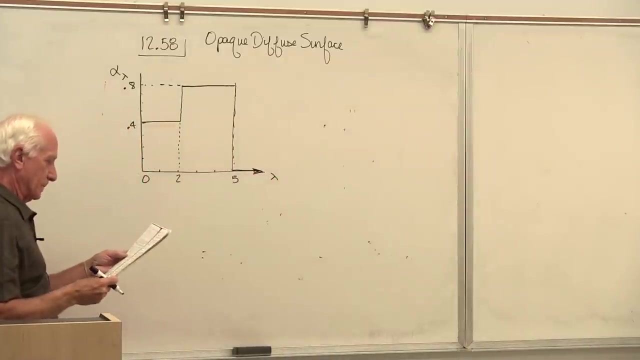 One Out to two, Out to two, Out to two. then it goes up to 0.8, then it goes out to 5 at 0.8, then it comes down to 0, and it stays at 0 all the way up. Okay, he says, I'm also going to give you an irradiation. 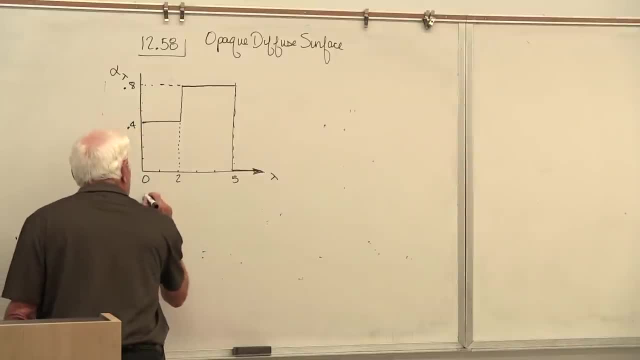 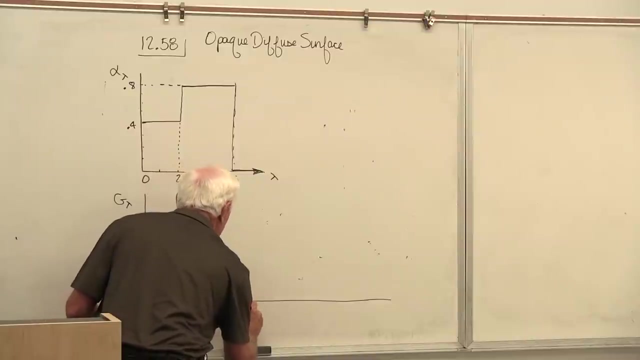 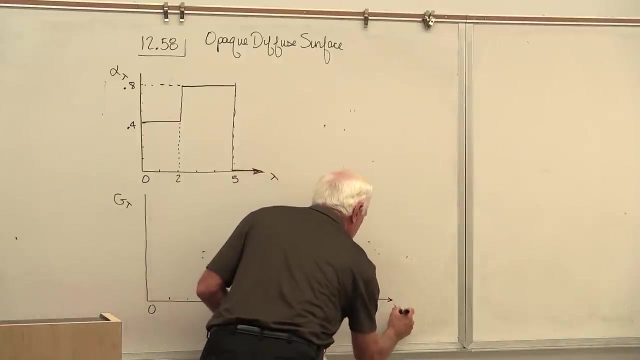 graph as a function of wavelength. So he gives a second graph. The second graph is the spectral irradiation G lambda- Okay, 0, 1,, 2,, 3,, 4,, 5,, 6,, 7,, 8,, 9,, 10, lambda From 2 to 10, it. 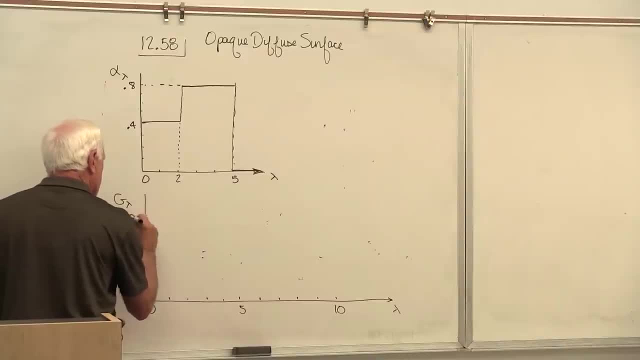 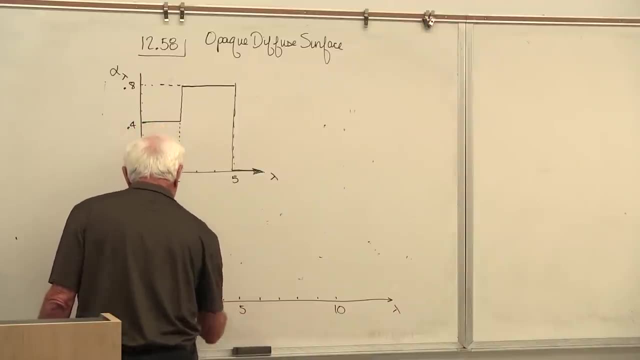 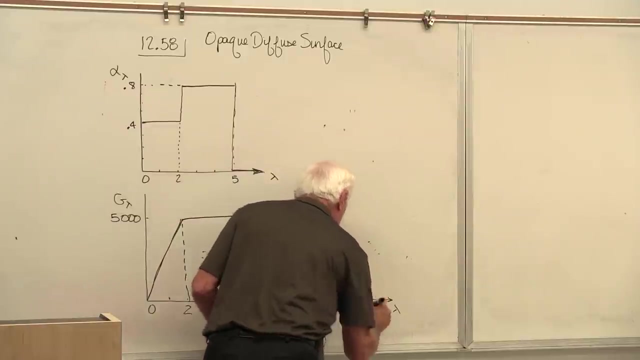 is 5,000 watts per square meter. 5,000 watts per square meter from 2 to 10.. Straight line, though straight line Constant out to 10.. At 10, drops down to 0 and goes over here. 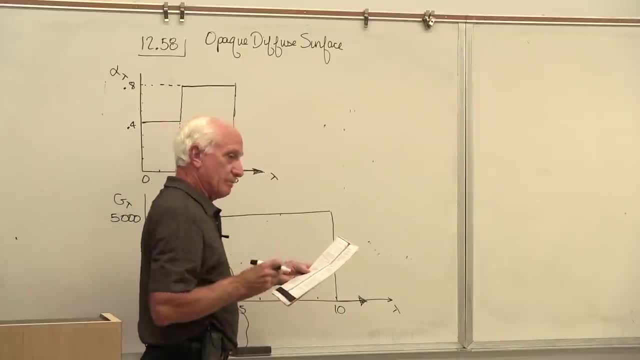 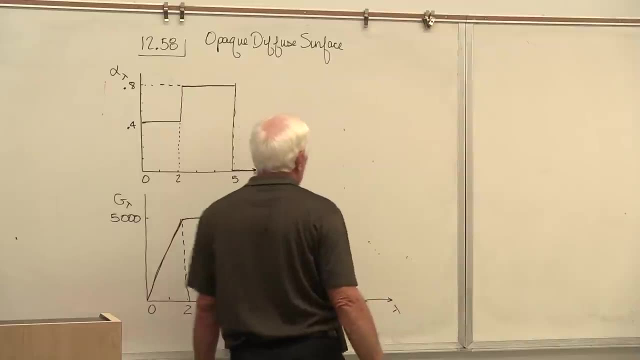 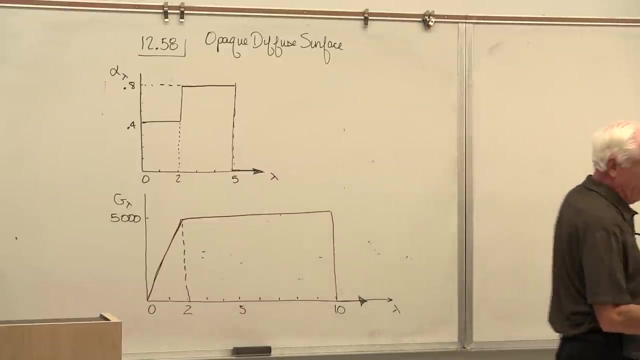 We'll do the first two parts. three-part problem. First part: what's the total absorptivity of the surface? I'll put it here. Okay, let's talk about these particular equations. I'm going to add those over here. We're not quite there yet. This is how we. 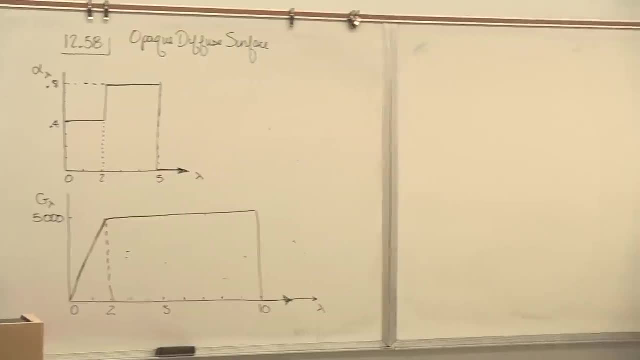 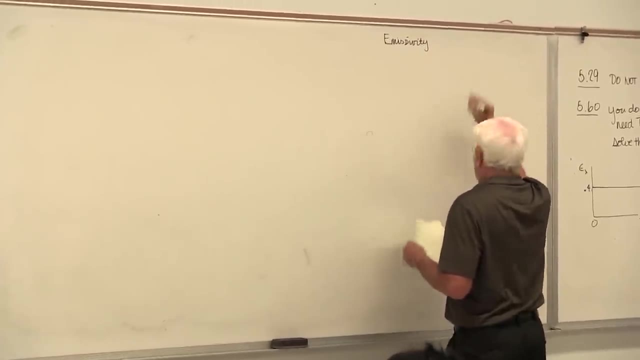 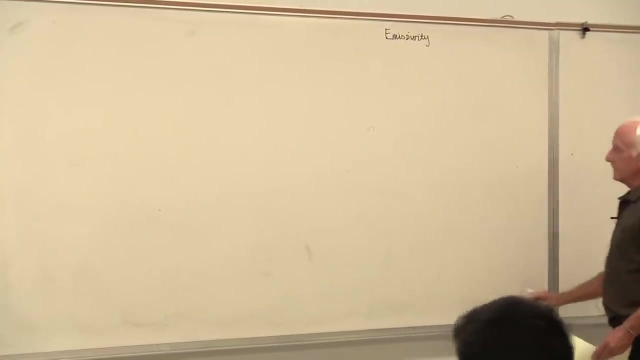 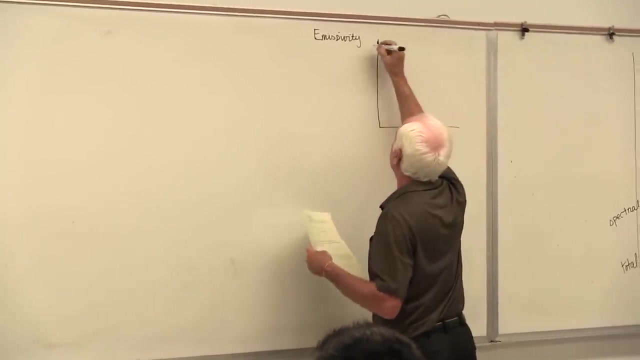 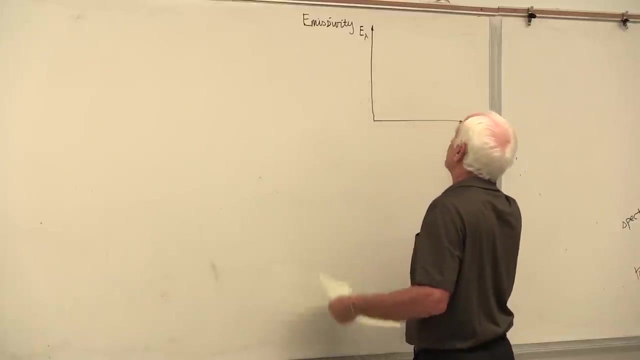 find emissivity. Okay, emissivity. how do we define emissivity? Well, let's draw a graph here similar to something like that. We have the. we're given the emissive power as a function of wavelength versus lambda. If the surface is black, it's black. If the surface is white, it's black. 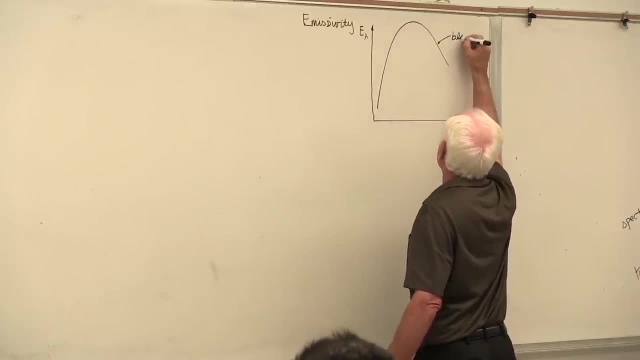 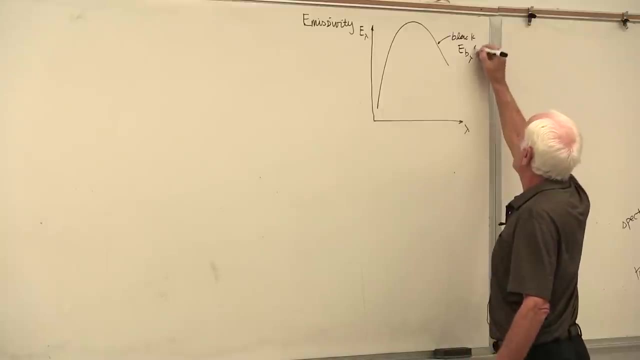 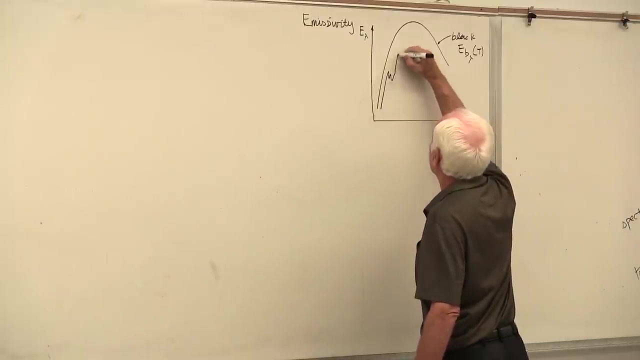 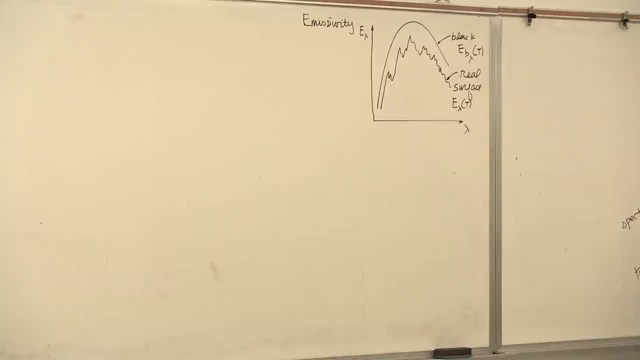 Emissive power as a function of wavelength at the same temperature, That real surface is jagged because it's not a nice, smooth curve. Okay, It might be this gray paint in the room on a wall. It might be the gray paint. These would be the real surface, the emissive 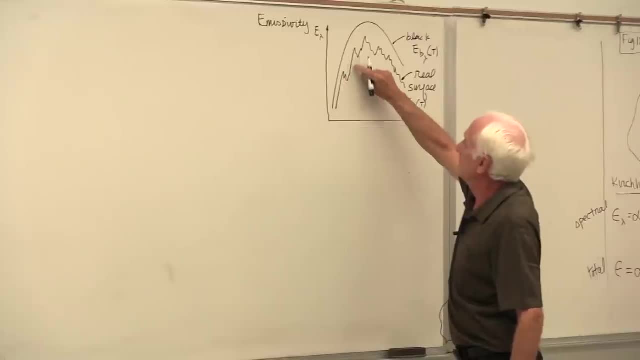 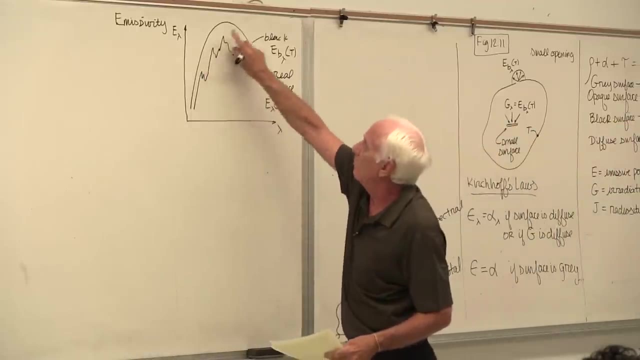 power of that gray paint here. If we'd figure out what the black body single power would, it would be this line here. At what temperature? Room temperature: 300 K. Both lines are at, let's just say, 300 K. 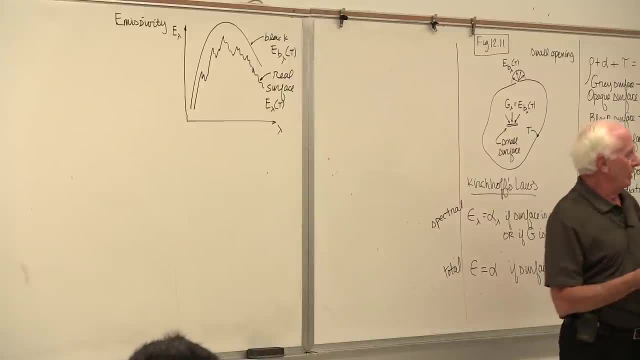 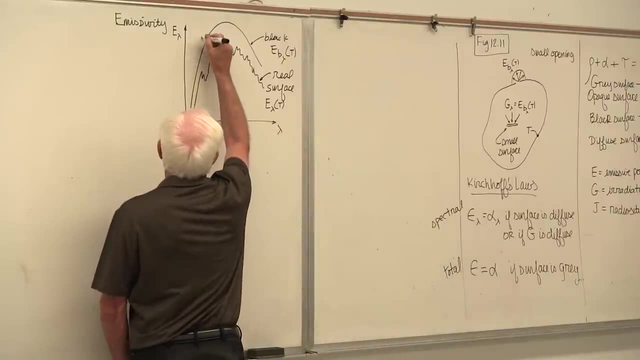 One's a black body at 300 K, The other one is the real gray paint at 300 K. So if we would take at any particular wavelength, take and divide the black body, divide the real by the black body. that's a definition. 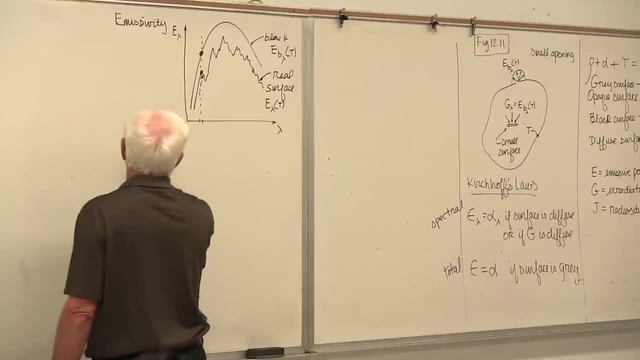 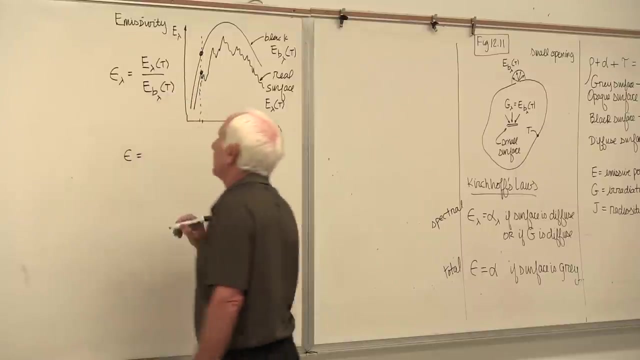 of spectral emissivity. So spectral emissivity, epsilon, Move it up here. Epsilon lambda equal E of the real body, E lambda of T divided by the black body. spectral emissive power. It's just a ratio of those two points. 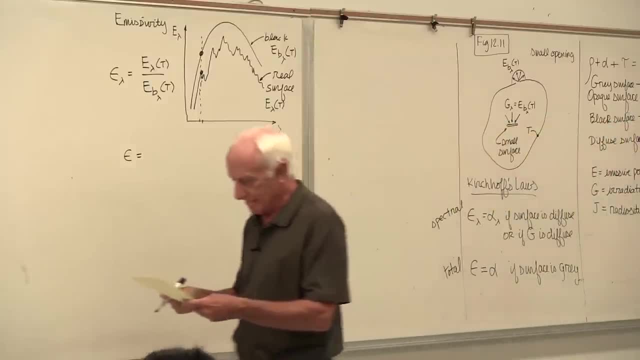 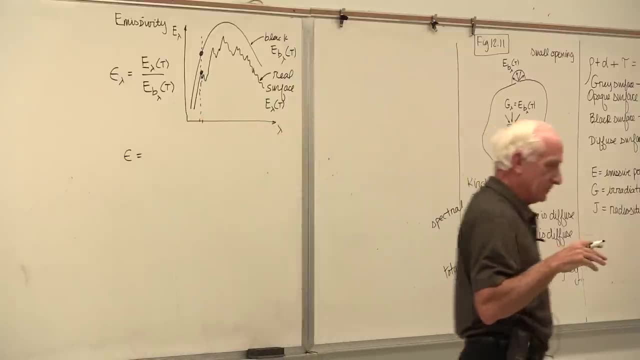 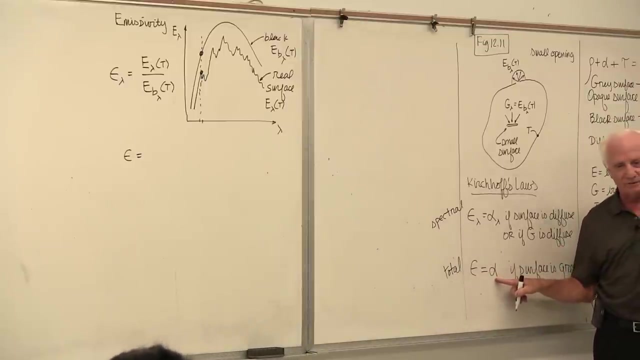 on a vertical line. Now, if we want to find the total emissivity of the surface, I can tell you right here: You want to find the total, You integrate over all possible wavelengths. okay, So I integrate these guys over all possible wavelengths. 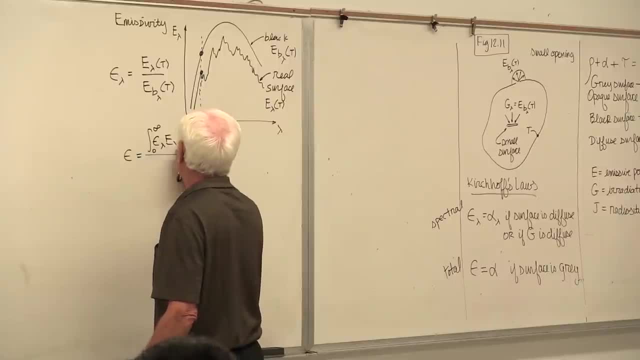 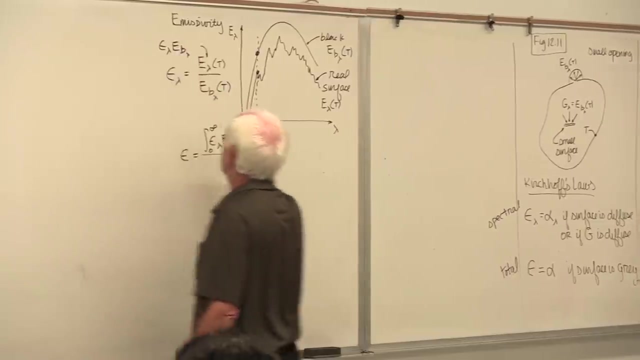 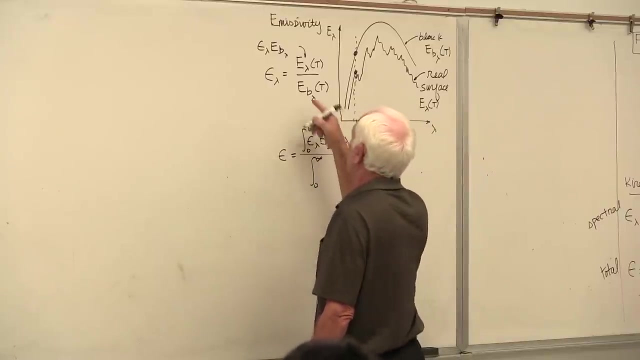 Epsilon lambda E B lambda. This guy right here, just so you know, is epsilon lambda E B lambda divided by black body emissive power total. Okay, there, it is. Okay, there it is Okay. there it is. 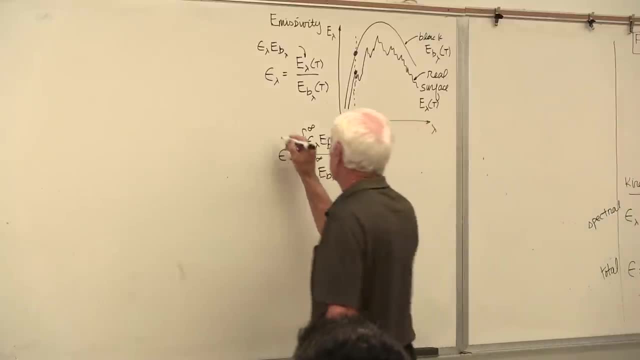 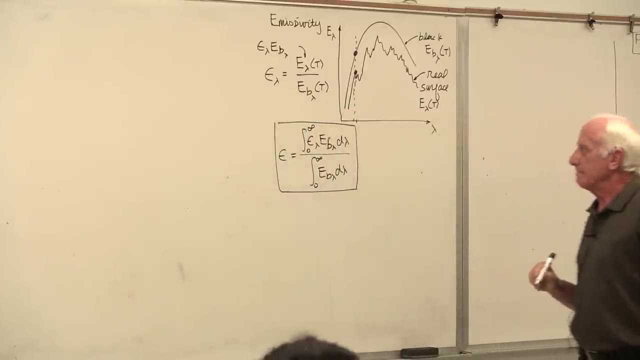 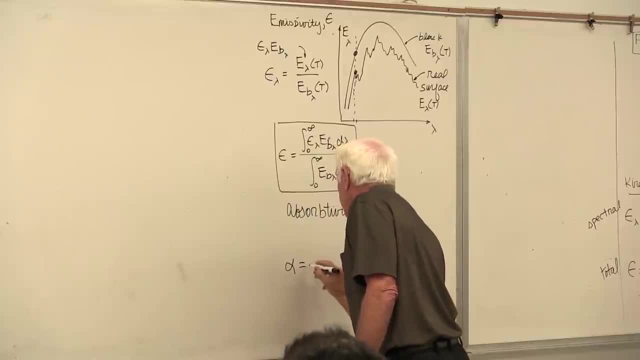 Absorptivity alpha: same way. We define it. the same way, We define it, the same way. This is the energy, this is absorbed, so it's G absorbed over the incoming radiation of G. The absorptivity is defined as the absorbed radiation over the total incoming radiation. 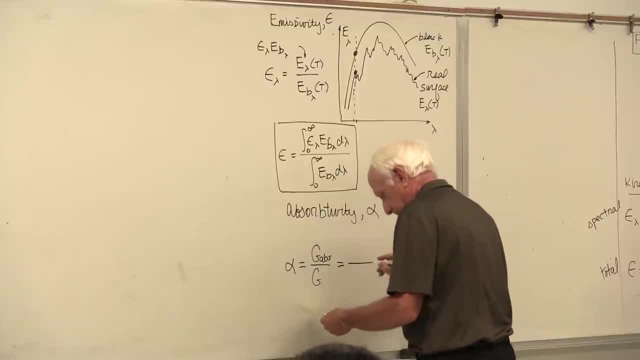 Okay, So we define it: zero to infinity wavelengths, alpha lambda- G lambda, D lambda, divided by zero to infinity of all the incoming radiation: G lambda, D lambda. Okay, that takes care of alpha. Reflectivity, Okay, reflectivity. 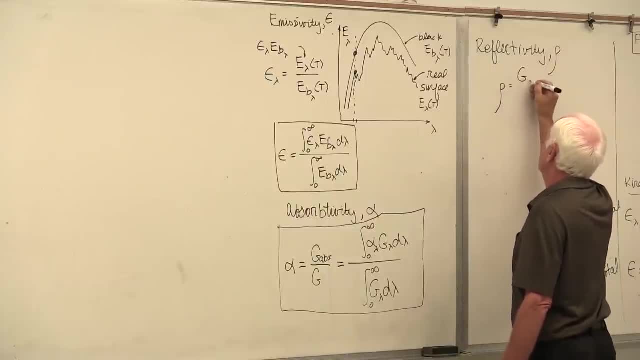 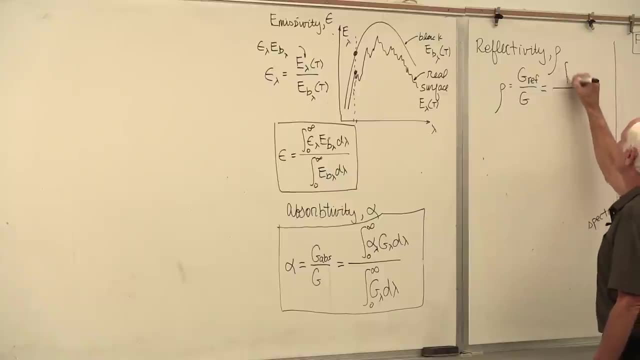 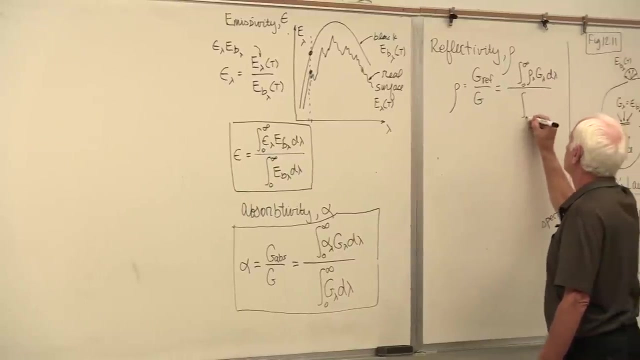 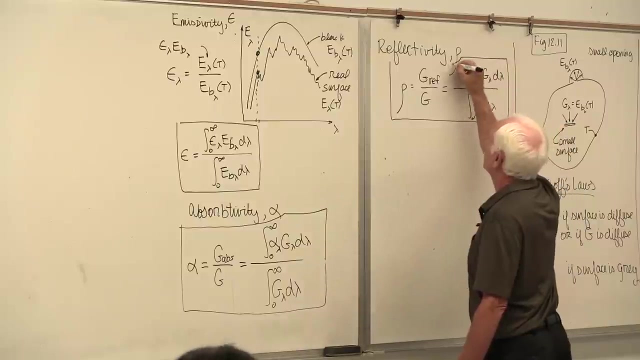 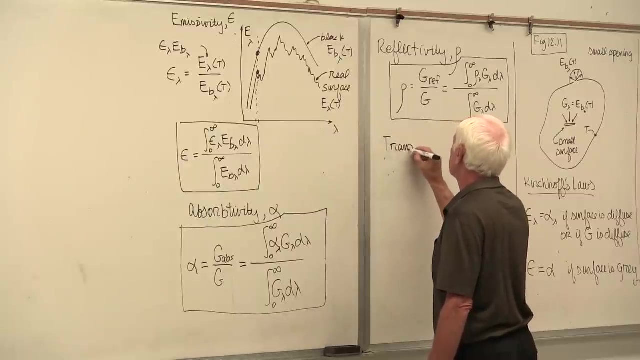 Rho. Rho is the reflected of the incoming radiation divided by the total incoming radiation. Okay, the last one transmitted Tau: The transmitted incoming radiation divided by the incoming radiation G. Okay, that takes care of alpha. Okay, the last one transmitted. 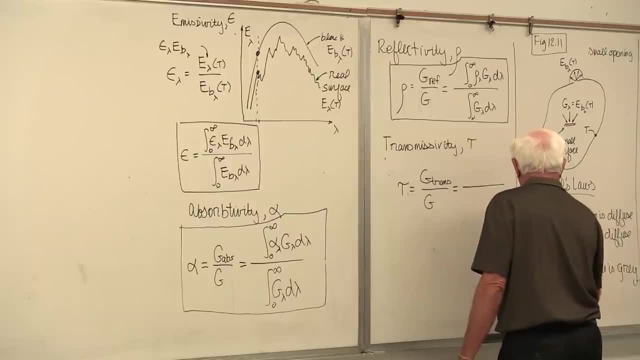 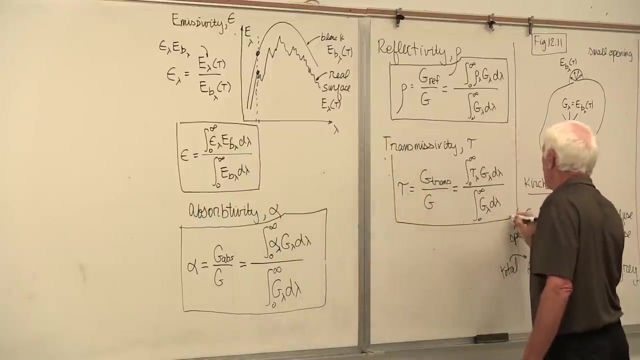 Rho. Rho is the reflected of the incoming radiation divided by the total incoming radiation. Okay, this is the of the incoming radiation. Okay, there are the four equations. Okay, Okay, that's it. There are the four equations. 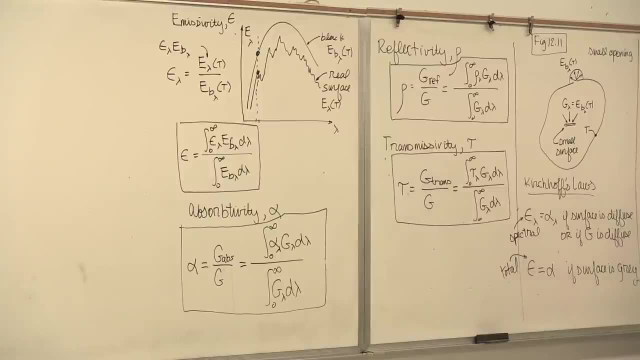 If you're given a graph of the spectral distribution of any of those four properties- epsilon, alpha, rho or tau- you use these equations then to find the total values of epsilon, alpha, rho and tau. Let's go back to our problem. 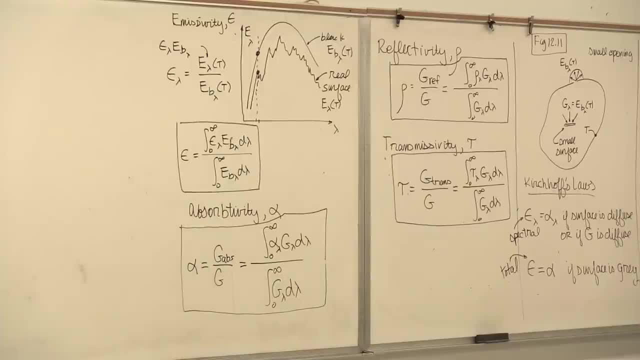 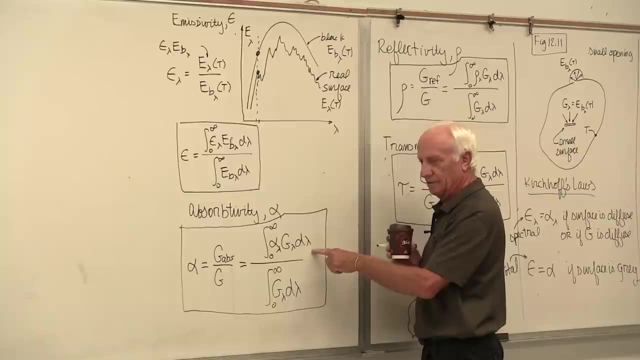 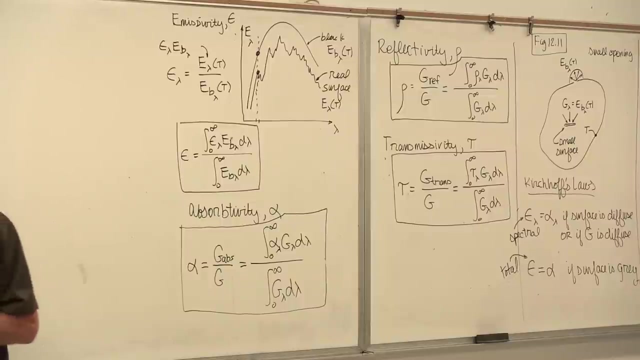 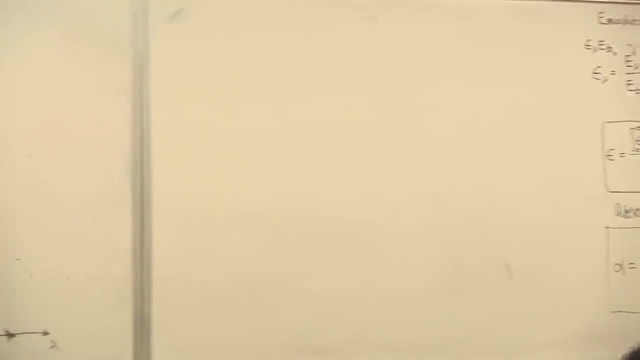 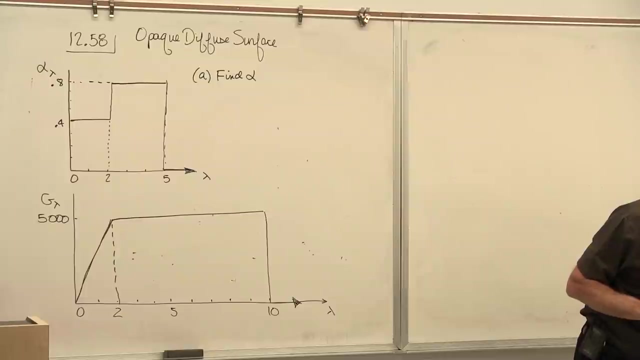 What did he give us? Oh, he gave us an alpha graph. Yeah, Yeah, Right down there, I know alpha lambda now as a function of lambda. Good Okay, Part one: find alpha. Part two: find emissivity. 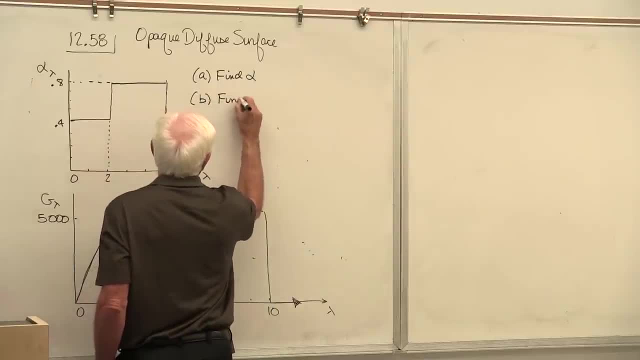 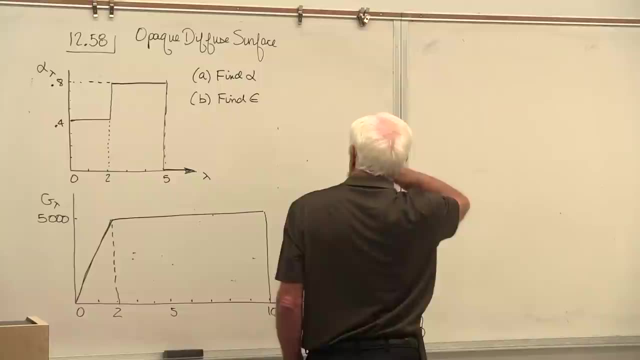 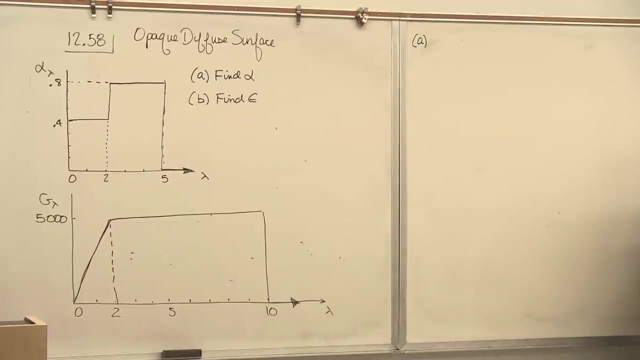 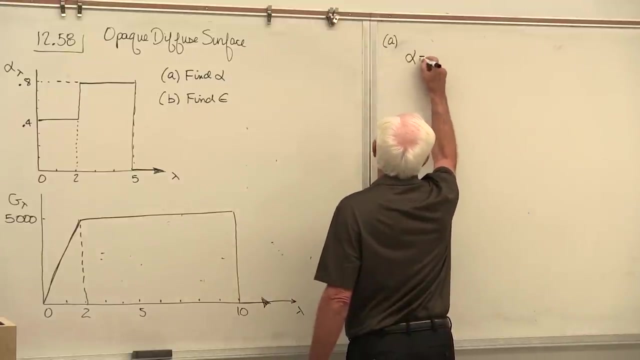 Okay, Let's do part A first. Okay, I'm supposed to find alpha. Well, it's not a big, you know. search There, it is Right there. Got it There, it is right there. So alpha equals integral zero to infinity. 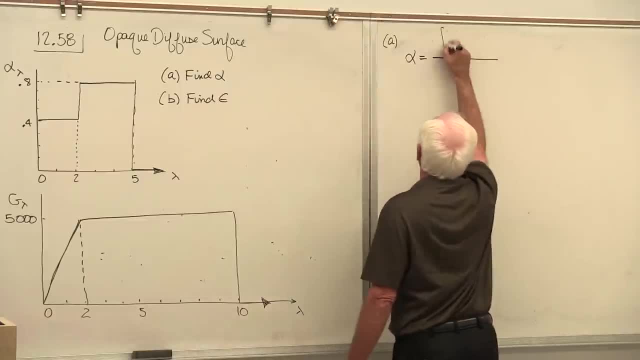 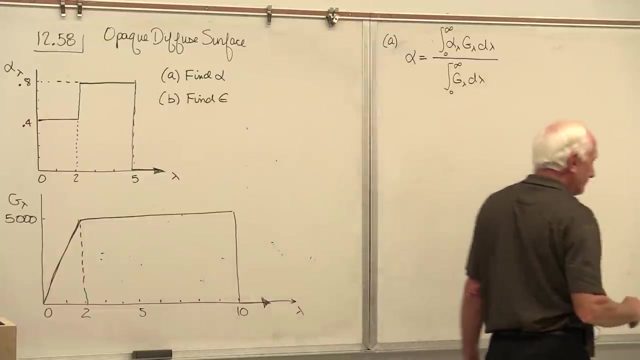 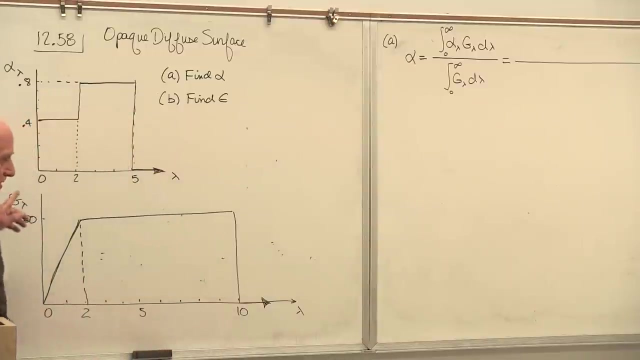 Okay, So alpha equals integral zero to infinity. Okay to infinity. alpha lambda g lambda, d lambda divided by zero to infinity: g lambda, d lambda. Now we're going to integrate by parts, And here's the rule: every time the behavior changes on either graph, that's going to be. 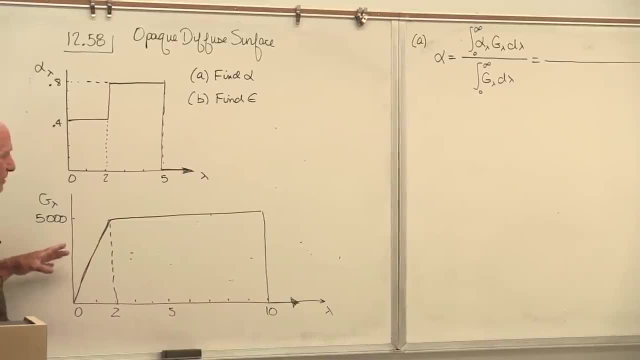 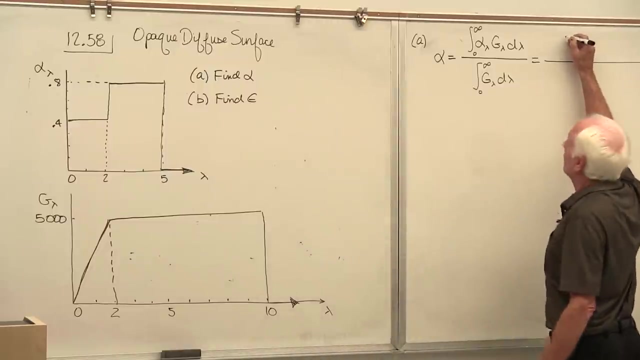 your limit of integration. If there's a change in either one of the two graphs, okay, oh for the alpha graph: at two something dramatic changes. The g graph: yes, at two something changes. So my first integral zero to two. 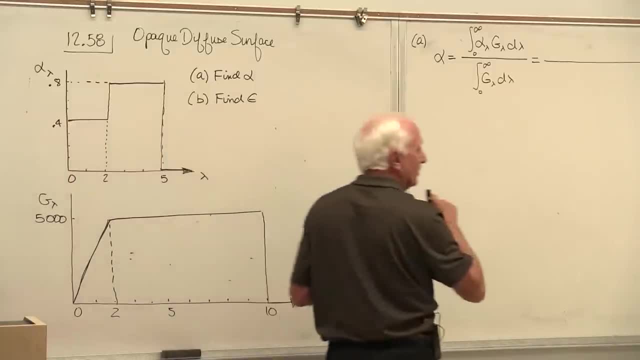 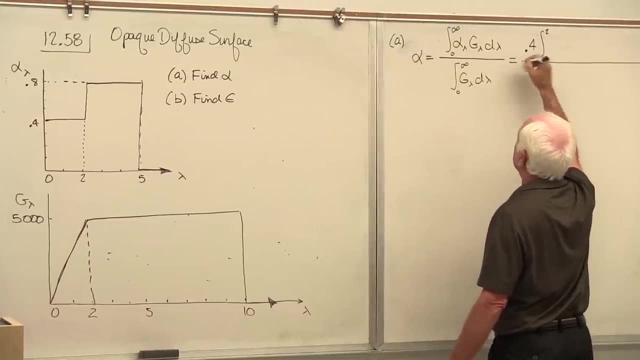 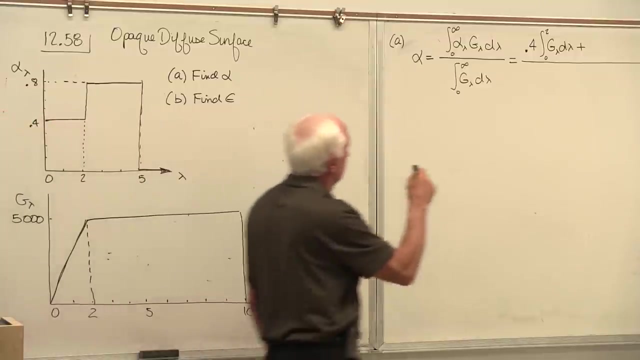 What's constant from zero to two. Alpha Float outside the integral sign .4, integral zero to two. What stays inside? G? lambda, d, lambda. The next breakpoint: look at both graphs: five, five, okay. integrate from two to five. 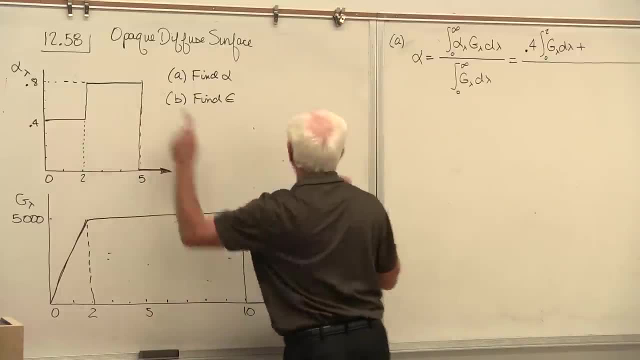 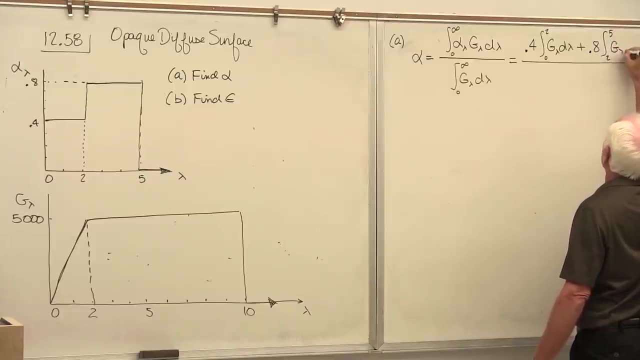 okay, What's constant? Look up here .8, also g. we'll come back to that integral of two to five g, lambda, d, lambda plus oh, ten. something happens Ten, Ten, Ten. So obviously from five to ten, integral five to ten. I'll put it in there by the time. 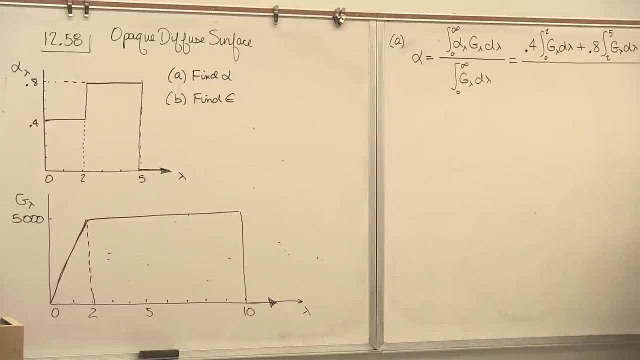 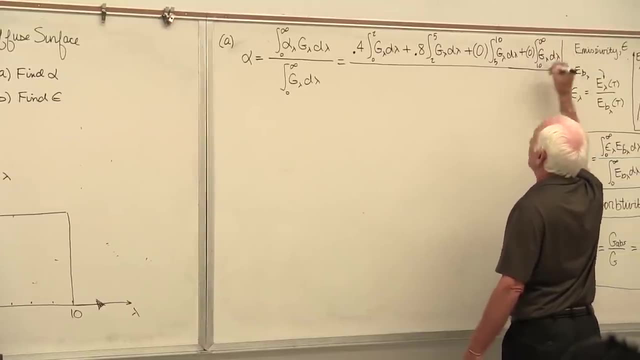 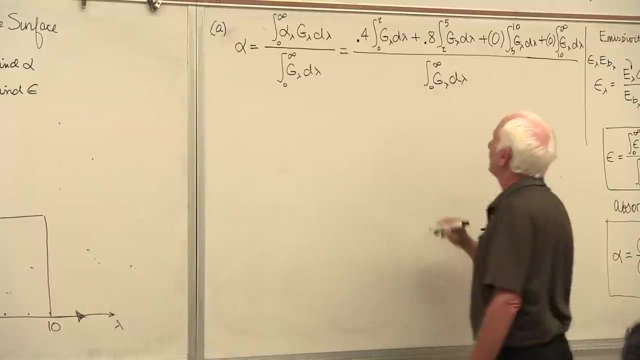 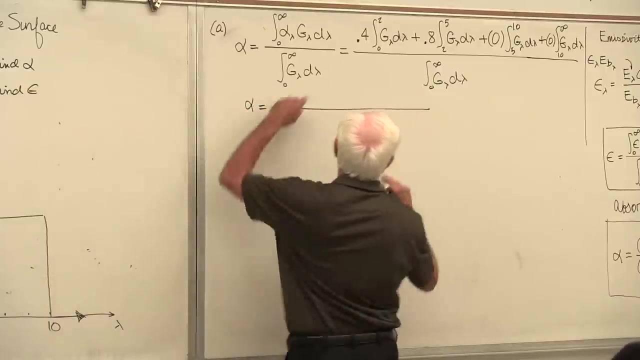 oh, it's zero plus zero integral, from ten to infinity. g lambda d lambda. divided by integral, zero to infinity: g lambda d lambda- Okay, alpha equal. this is the area under the g lambda lambda graph from zero to two. 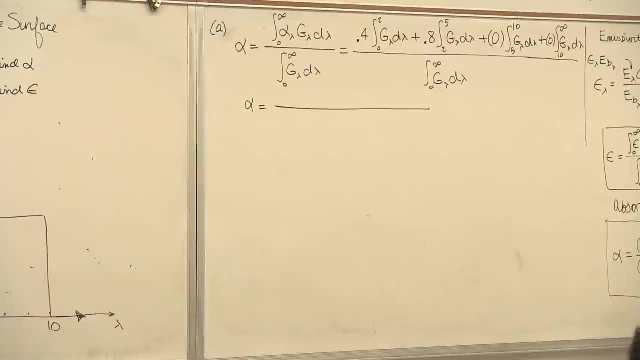 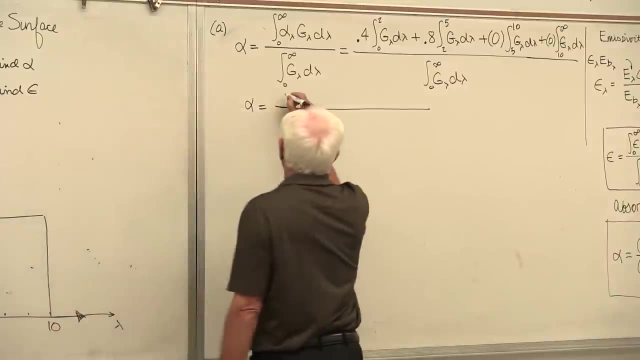 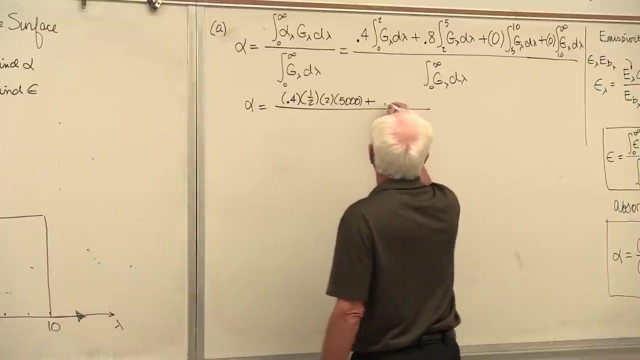 The g lambda lambda graph, zero to two. the right triangle one half base times height. base is two. height is 5,000, plus .8 times the area under the g lambda- lambda graph, from two to five. 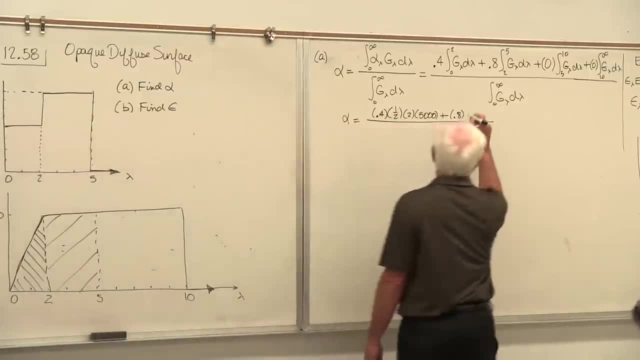 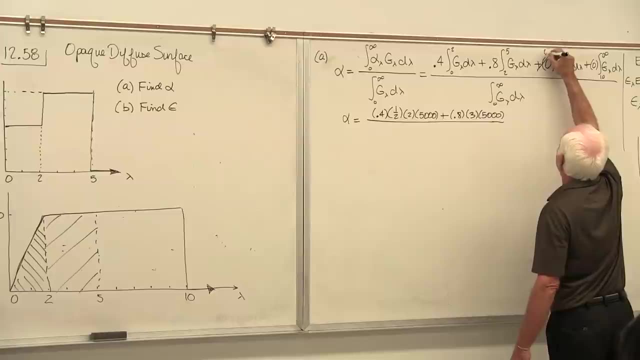 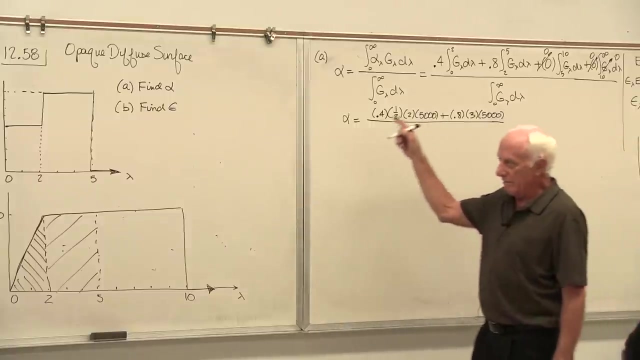 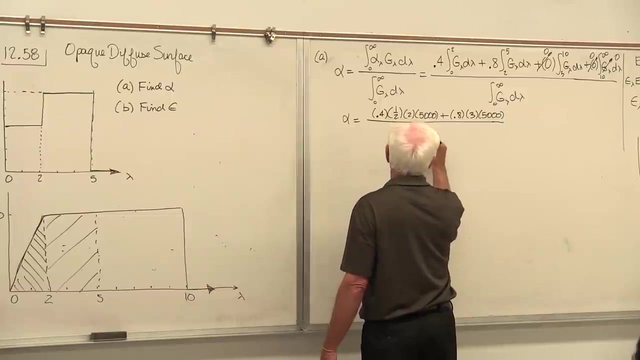 Rectangle three by 5,000.. Okay, Okay, Okay, Okay. This guy zero, this guy zero. G lambda here: zero. two zeros. G lambda zero. alpha lambda zero. divided by the area under the whole curve: one half base times height plus a rectangle. 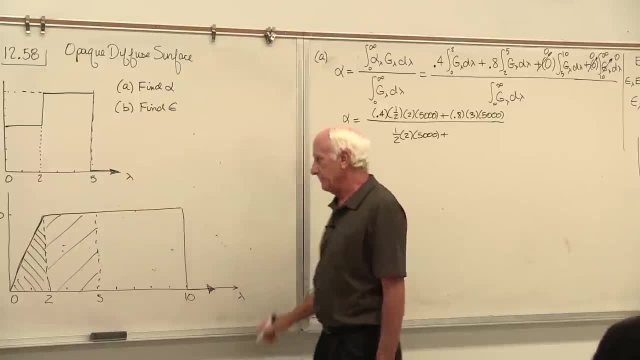 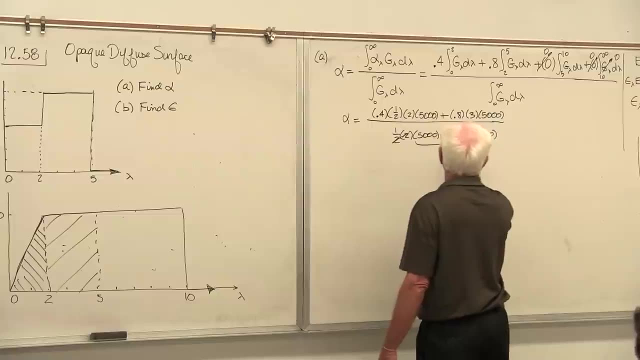 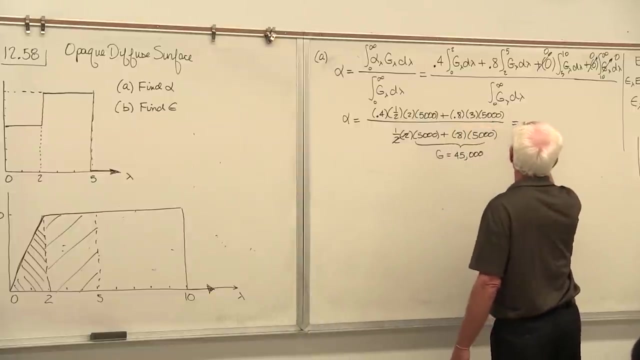 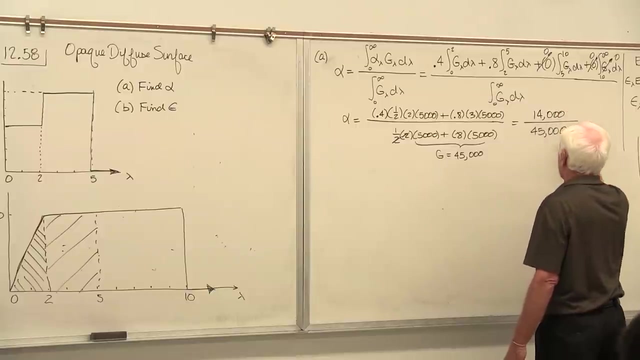 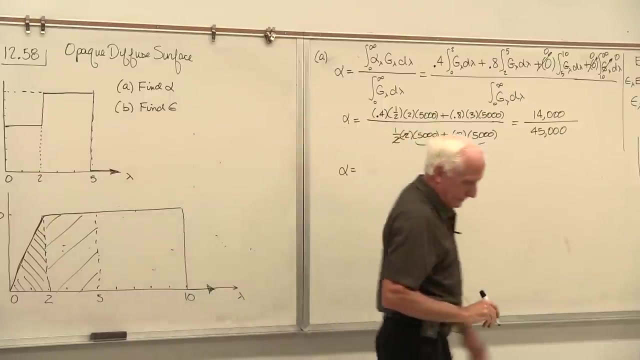 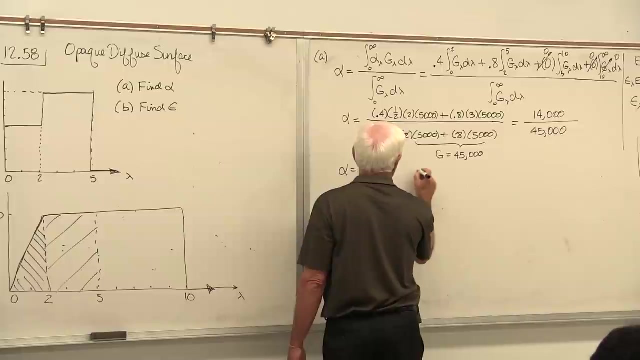 10 minus 2 is 8,, 8 times 5.. G equals 45,000.. I think that's 14,000,. let me just verify it. Yeah, it's 14,000.. So we end up with alpha .311.. Okay, that's part A. Now we'll do part B. 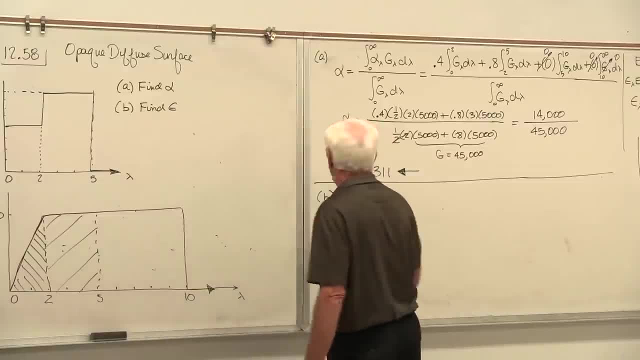 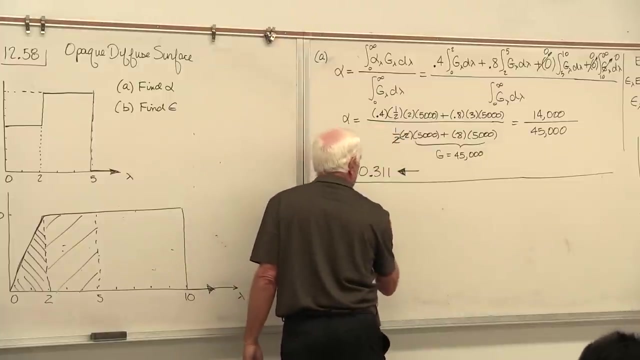 Okay, find the total emissivity. Okay, total emissivity, Transmissivity, tau, reflectivity, rho, absorptivity, alpha. Oh, there it is. He wants that guy. Okay, epsilon. Epsilon is equal to integral, zero, to infinity. epsilon lambda E, b, lambda, d, lambda. Okay, that's. 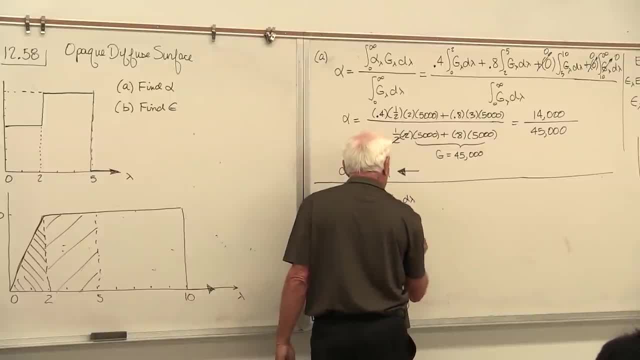 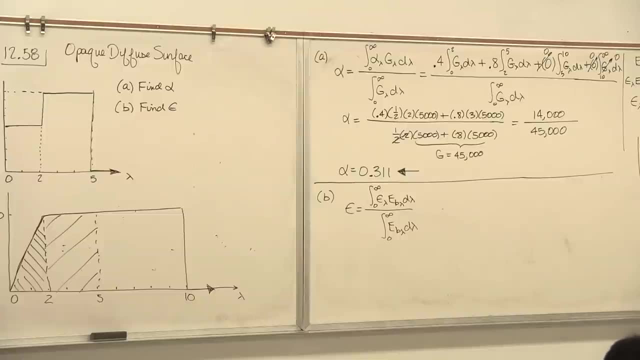 it Okay, Okay, Integration, Integration by parts. We're doing integration by parts. That's what we're doing. Anytime there's a change in the epsilon lambda graph or the G graph, that's your limits of integration. Say yeah, but he didn't give me an epsilon lambda graph, He gave me an. 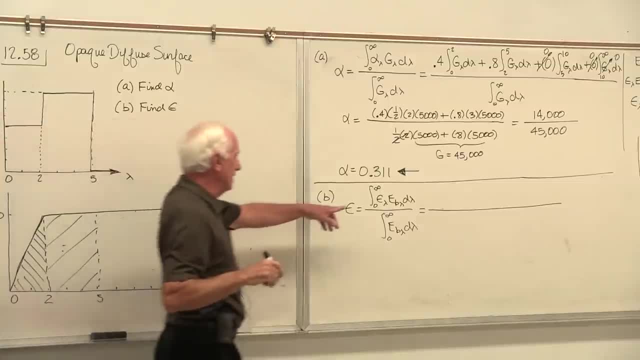 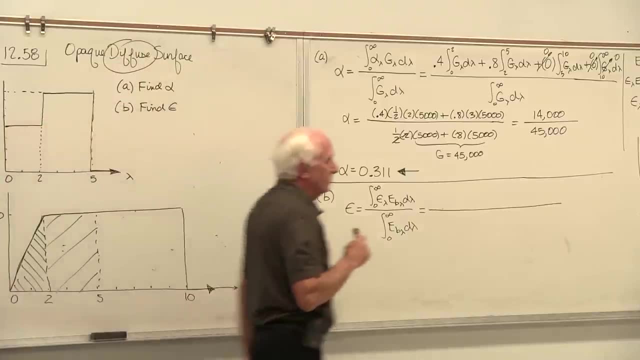 alpha lambda graph. I don't have the epsilon lambda graph. Oh, yes, you do. There's a magic word: Diffuse. Go over here Kirchhoff's laws. Oh, thank you very much. If the surface is diffuse, I can say the spectral emissivity equals the spectral absorptivity, So the 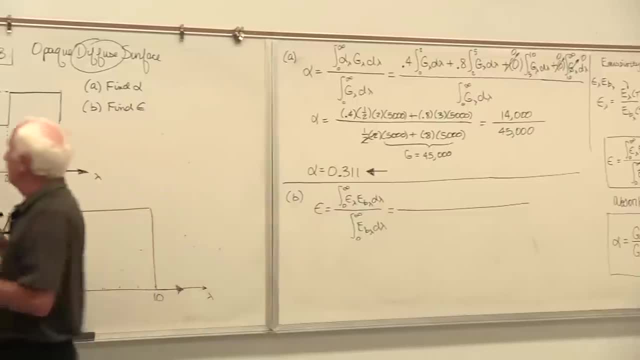 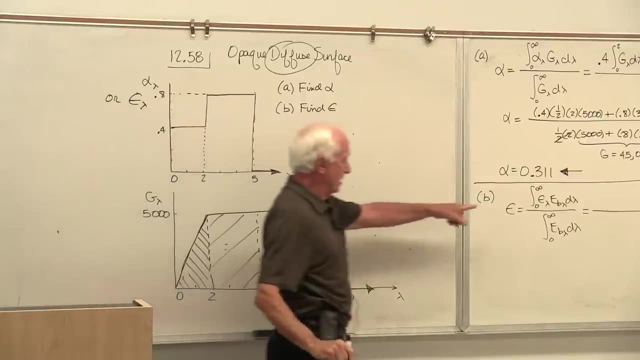 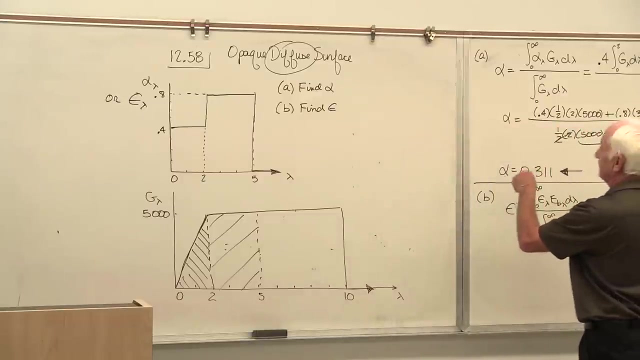 graph he gave me for absorptivity is also a graph for emissivity. Okay, there it is. The back goes in There. Limits of integration. Now we've got this. the same thing: 0.4.. Integral zero to R2.. E b lambda, d lambda. 0.8.. Integral to R2.. 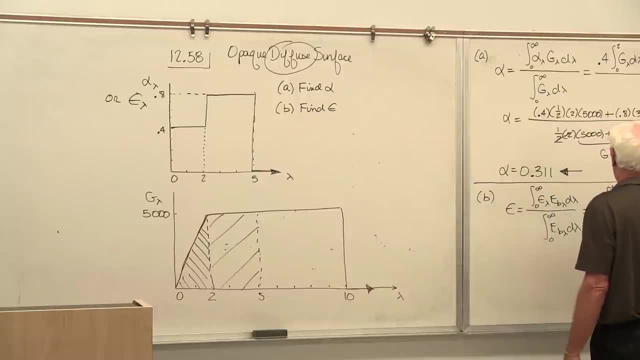 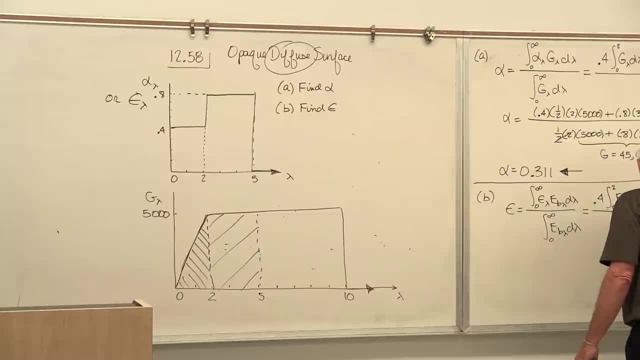 by e, b, L and it's e by D, learnt O, a, That's 5.. Two to 5.. E v lambda d lambda, Divided by integral zero to infinity. E v lambda d lambda, OK, Ok. 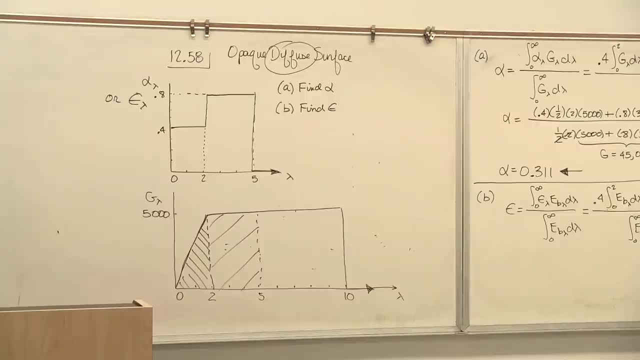 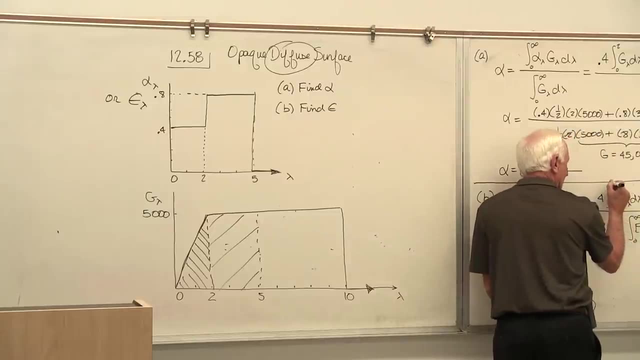 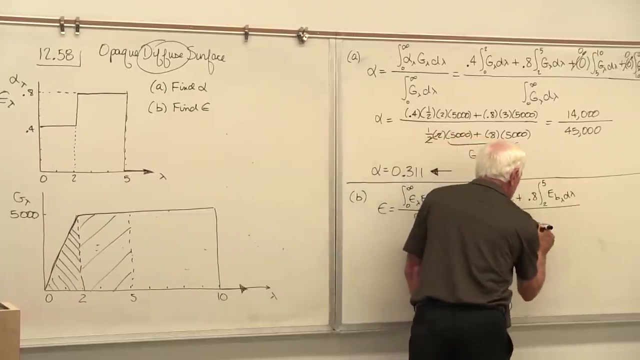 Ok, Ok. Then I say: gee, you know what This looks familiar. I think I've seen this somewhere before in Chapter 12.. Yeah, you have That thing right. there is F0 to 2 microns. Okay, Table 12-1.. 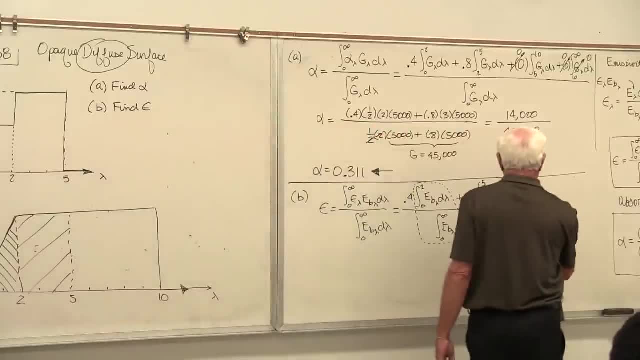 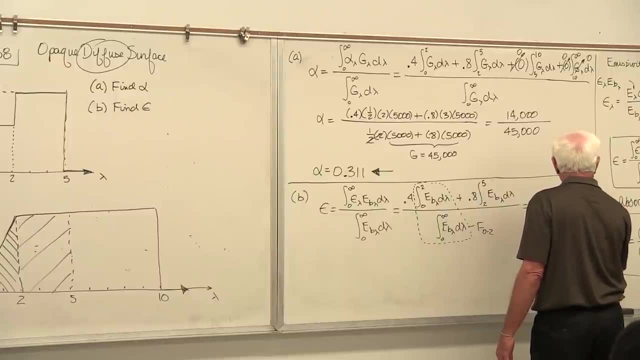 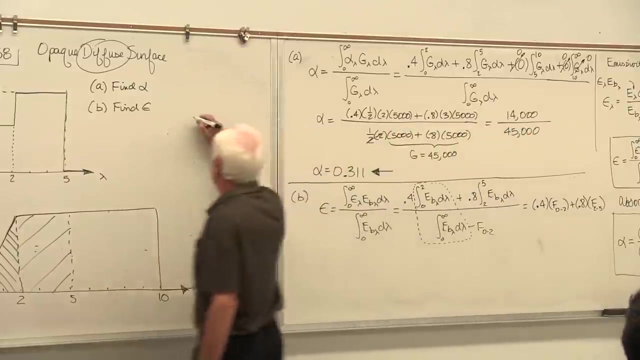 Table 12-1.. So this becomes 0.4, F0 to plus 0.8, F2 to 5.. Band emission: we covered band emission last time two times ago. Okay, Got to go to Table 12-1 to get the F factors. 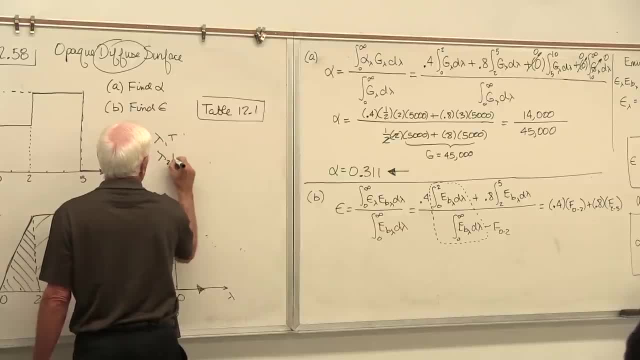 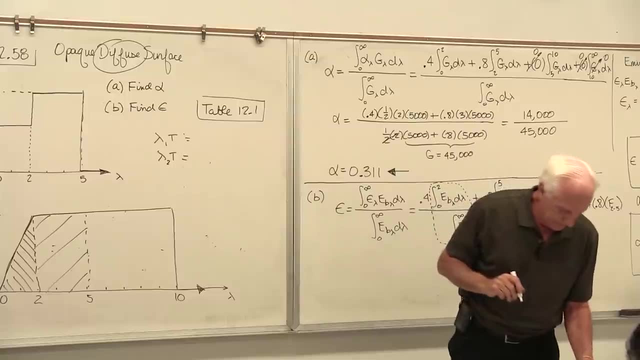 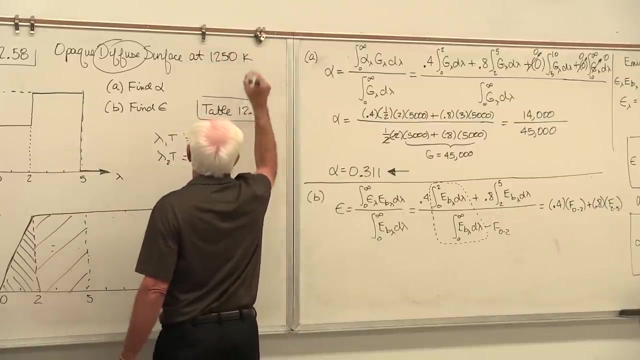 Lambda 1T, Lambda 2T. I need both those guys. Okay, Let's read the problem. Okay, The temperature of the surface is 1250K. All right, At 1250K, What temperature is that? 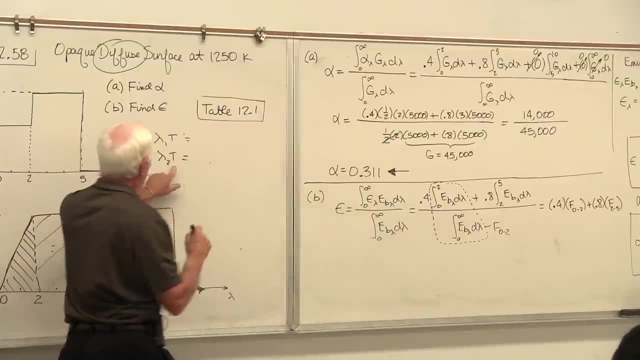 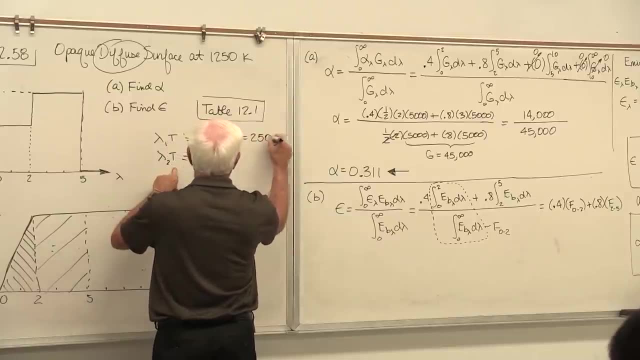 Well, that's the temperature. That's the temperature of the surface. of course That's 1250K. So we have 2 microns times 1250K 2500.. Lambda 2 is 6 times 1250.. 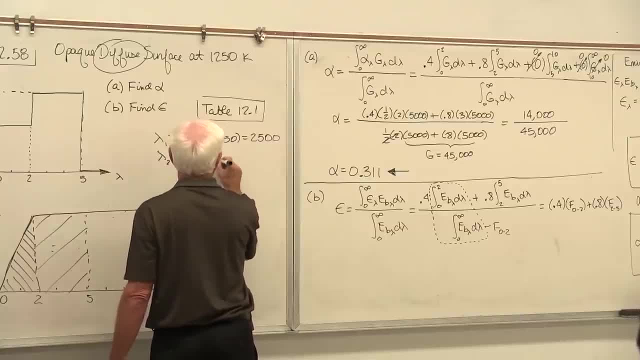 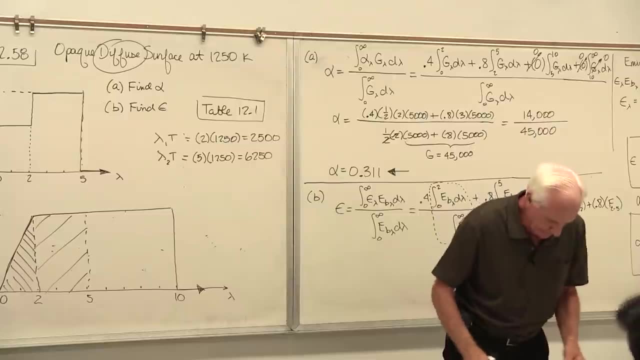 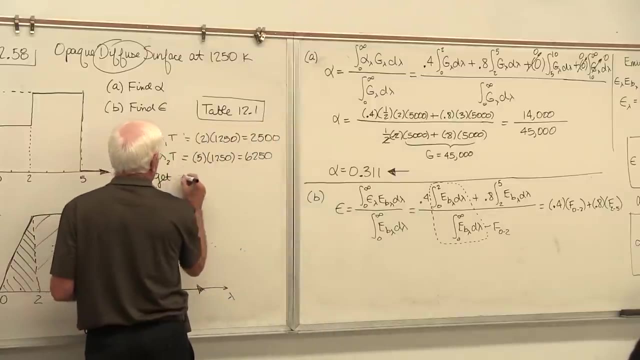 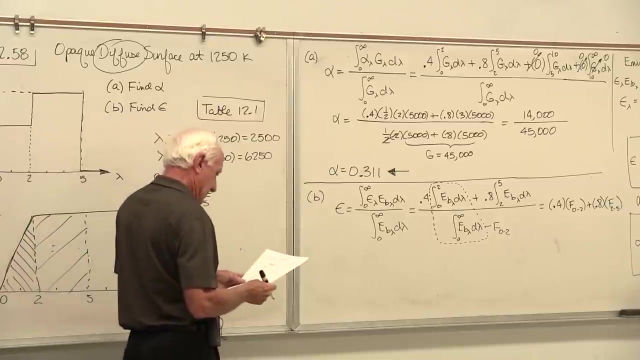 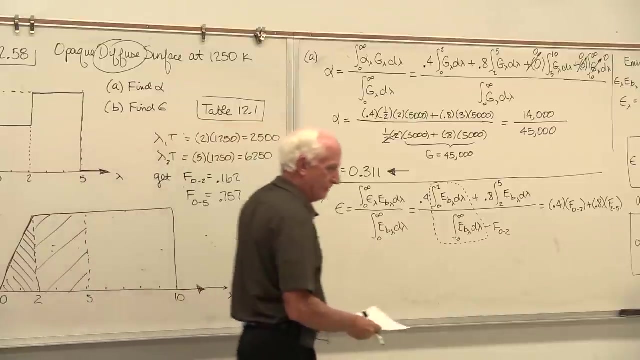 Oh fine, pardon me, 6250.. Okay, And we get F0 to 2, and we get F0 to 5,: 162,, 757.. Okay, There they are. Come back over here, Do what it says. 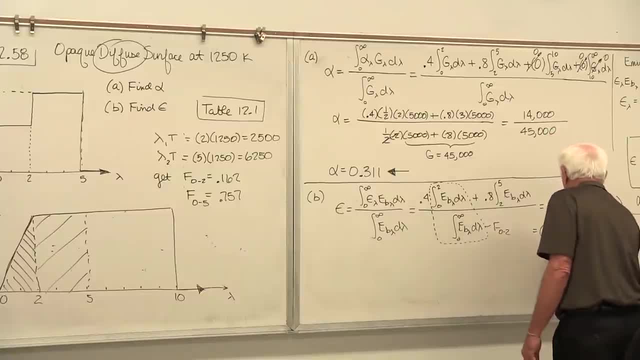 0.4 times F02, 162.. Plus 0.8,. now, don't forget, this is band emission. so you take F05 minus F02, 757 minus 162, and I get epsilon, the total emissivity. 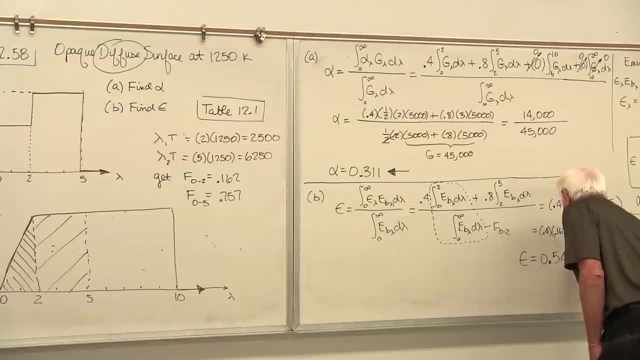 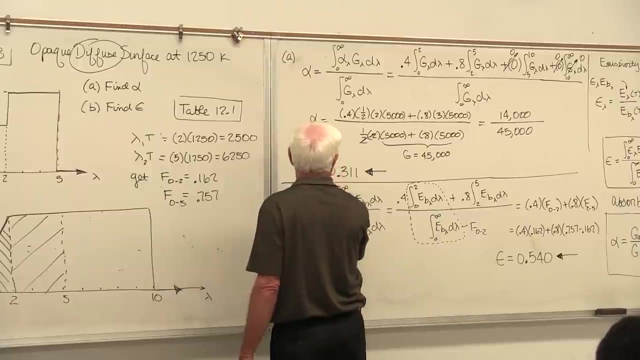 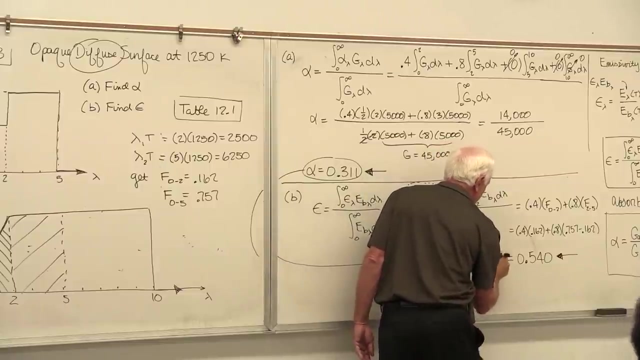 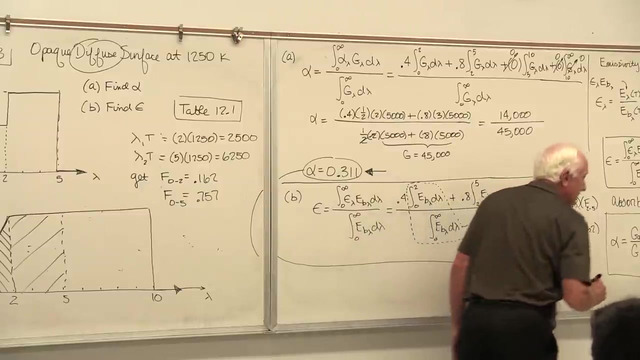 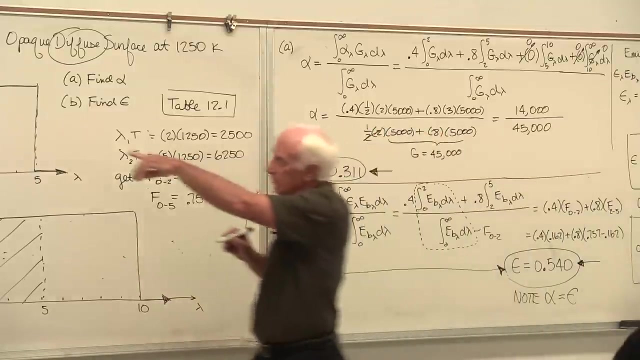 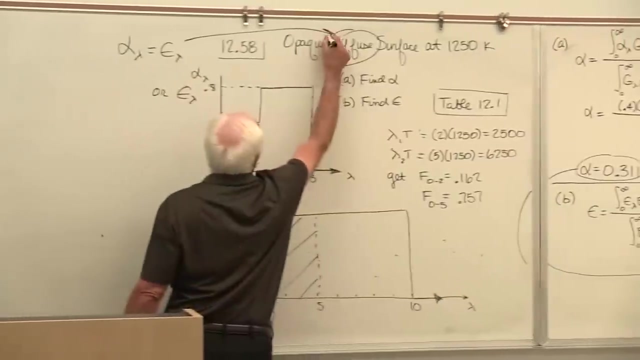 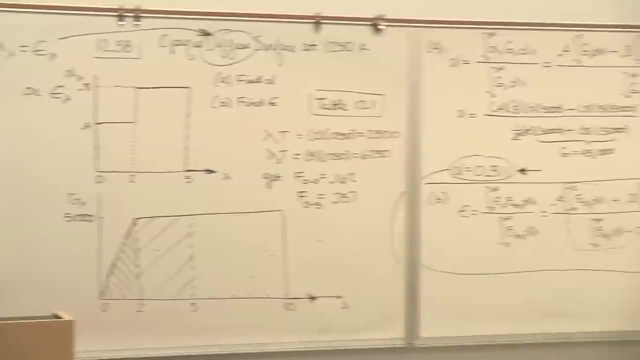 .540.. You can see the answer. The answer is: alpha is not equal to epsilon, But of course, alpha lambda equal epsilon lambda. Why? Because of the word diffuse? Go back over here again. When can I say epsilon equal alpha? 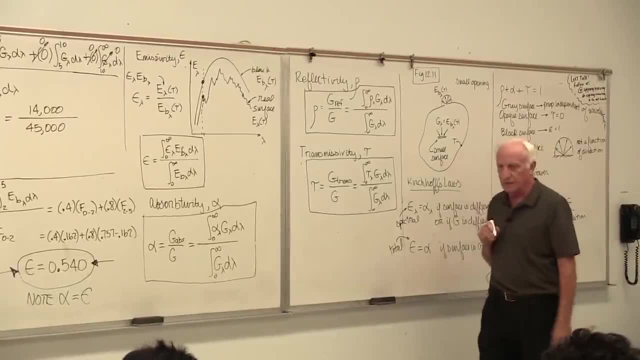 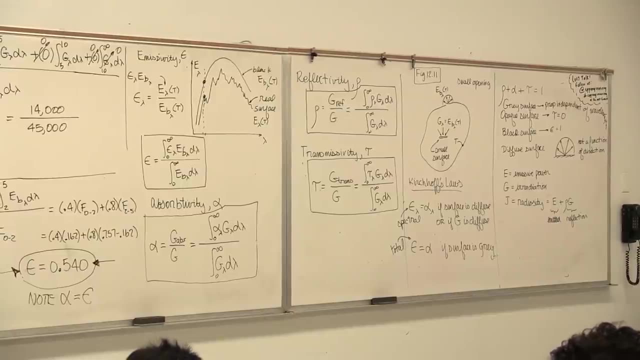 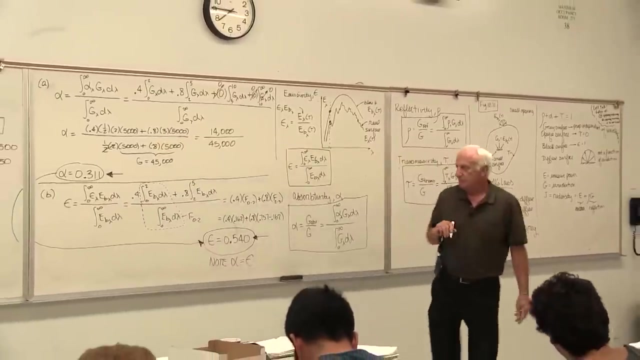 Here it comes. If I see the magic word, the surface is gray. It's not a function of wavelength, No, it's a function of wavelength. Look at it, It changes. So no, I can't say that, I can't say, I can't say: alpha equal epsilon, uh-uh, illegal. 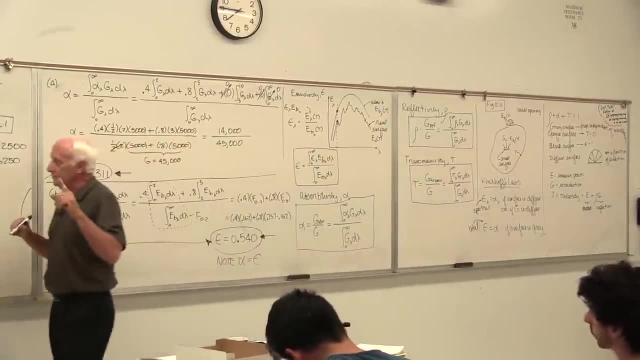 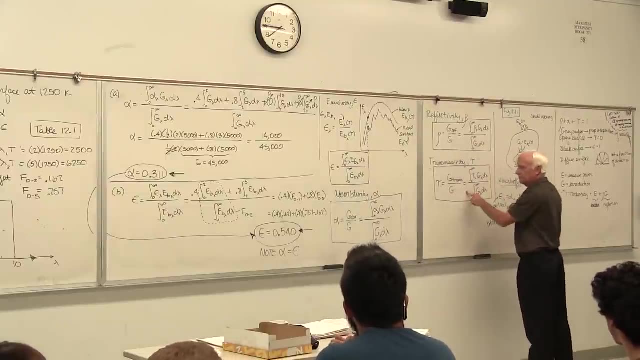 When did I use the G graph for the solution? I used the G graph wherever those equations and boxes show the symbol G. I used the G graph for this one, for this one and for this one. And where do I use the temperature of the surface? 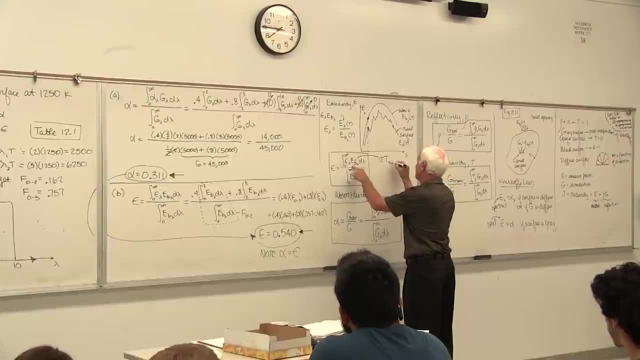 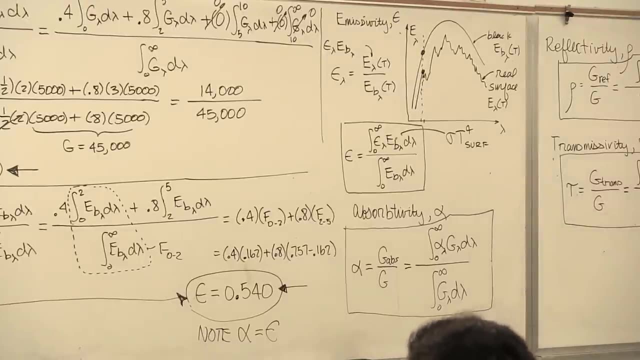 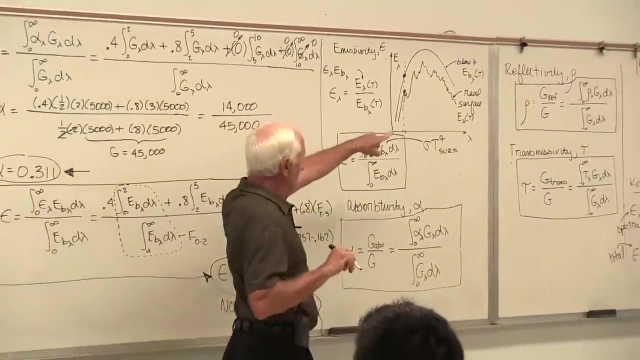 Look E B lambda, sigma T, surface to the fourth Right there. So that's what the G graph does for you there. okay, It allows you to calculate these properties: reflectivity, transmissivity, absorptivity. 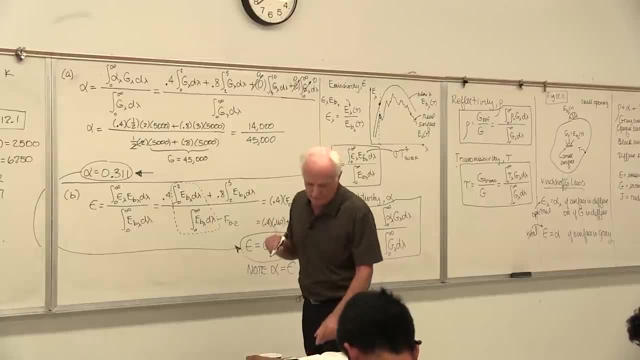 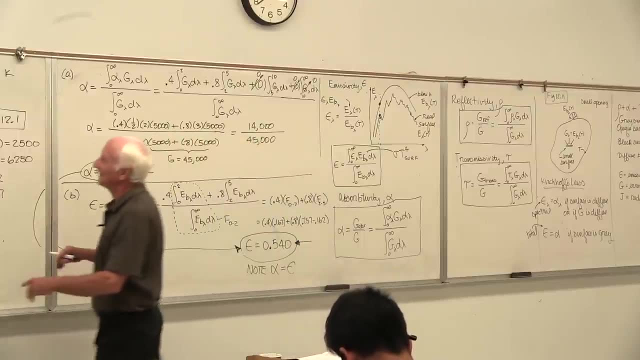 Okay, I think that pretty much covers everything on that problem. Is that supposed to be a node on alpha that's not equal to epsilon? Oh yeah, Which one On bottom Bottom? Yeah, Thank you, That's it, Thanks. 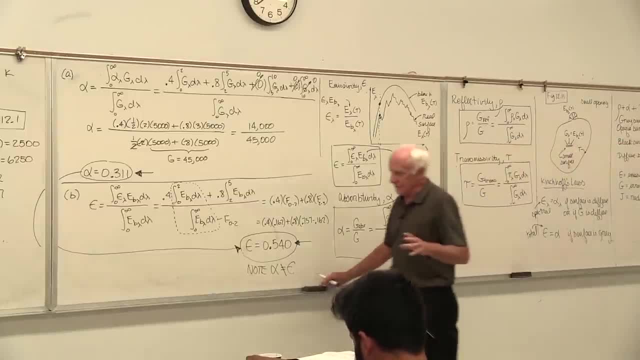 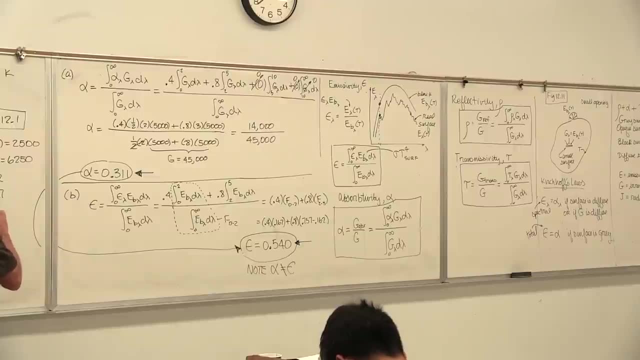 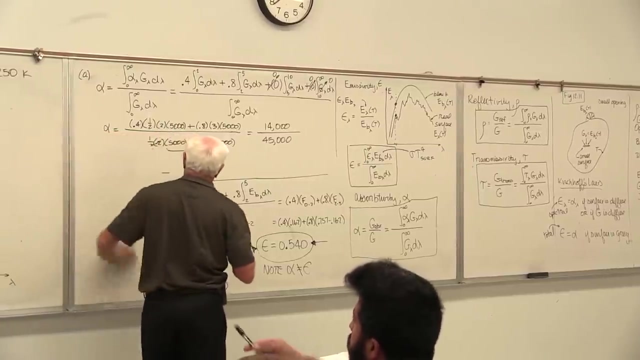 Okay, Let's do another one. I'll show you a little variation. now. I'm going to put these guys side by side, so I'm going to save this. I'm going to put the next problem right here: 1259.. 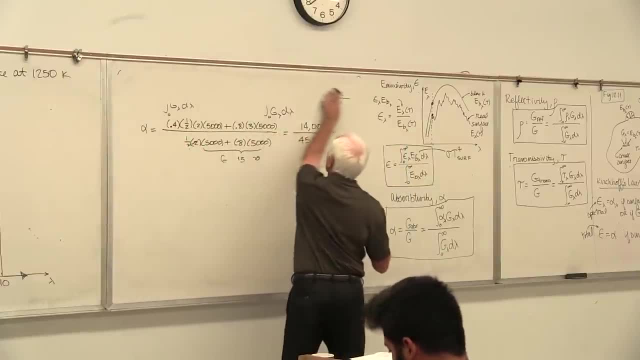 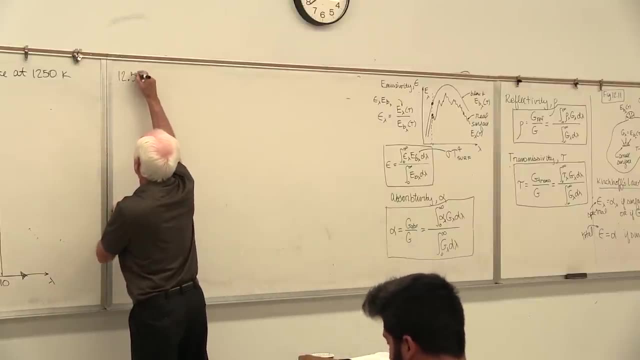 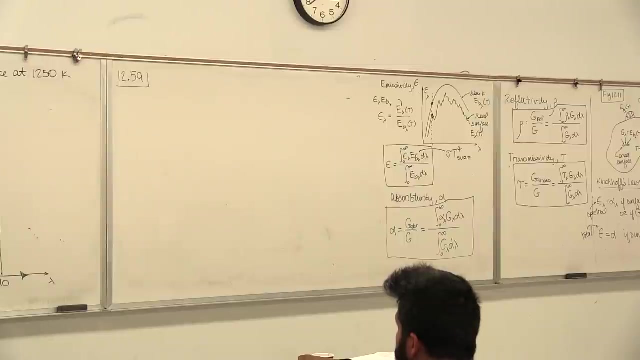 Okay, Okay, Professor. how come you don't use the area for the top graph? Which one? This one? Yeah, What area? When you're doing the calculations, you just use equal to 0.4 instead of 0.4 times 2.. 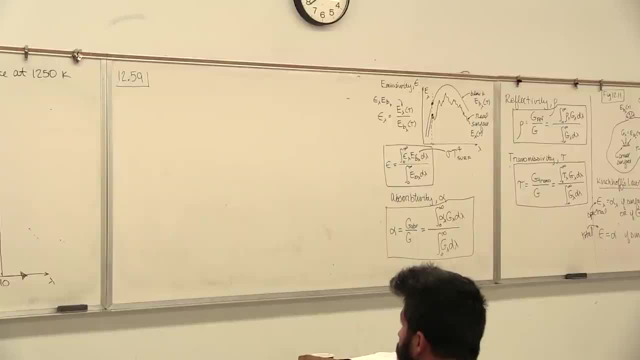 I pulled the alpha outside. I'm left with what? Am I integrating the area under the epsilon graph or the G graph? This is the integral. This is the area under which graph. I don't have this. I don't have this. 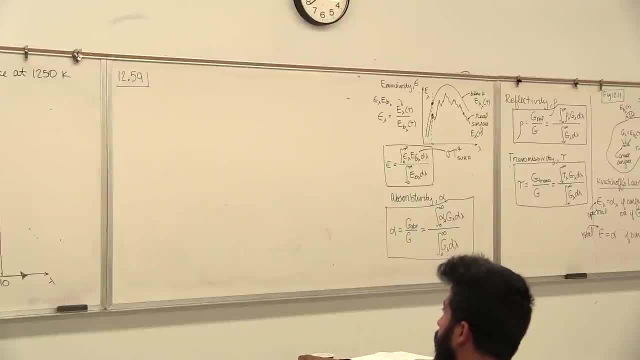 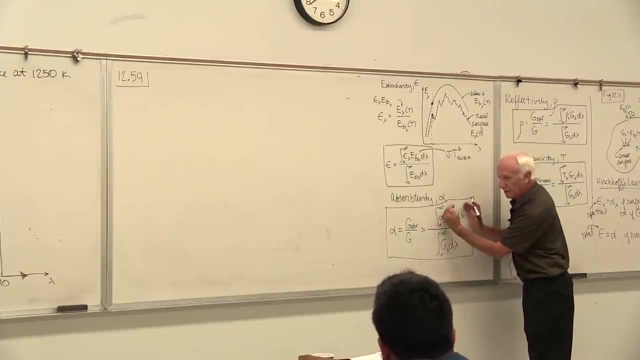 No, no, no, That's the area under that graph. No, I don't have that. I have this area here. Pull the alpha Outside the integral sign, because it's constant. What are you left with? The area under the G graph, not the area under the epsilon graph. 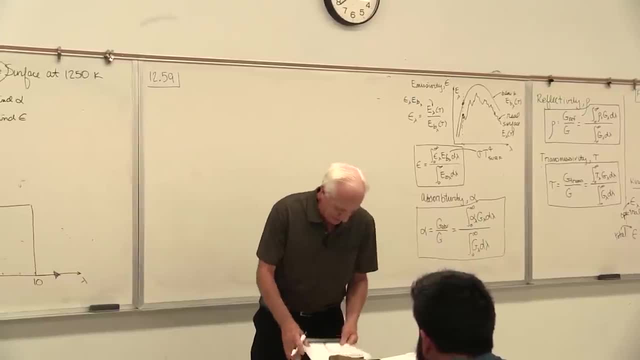 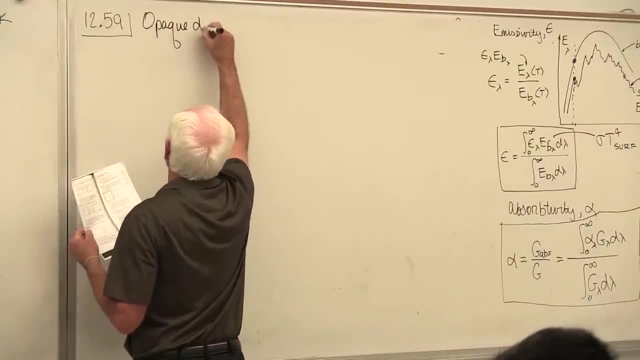 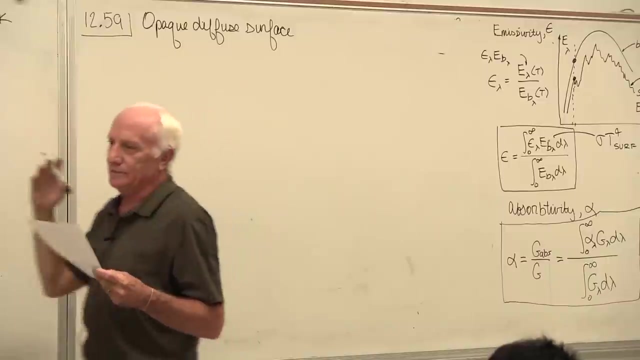 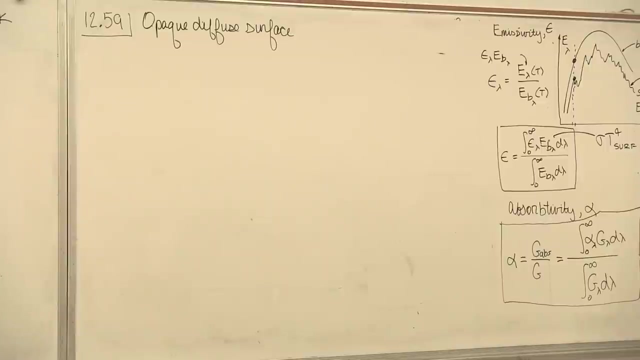 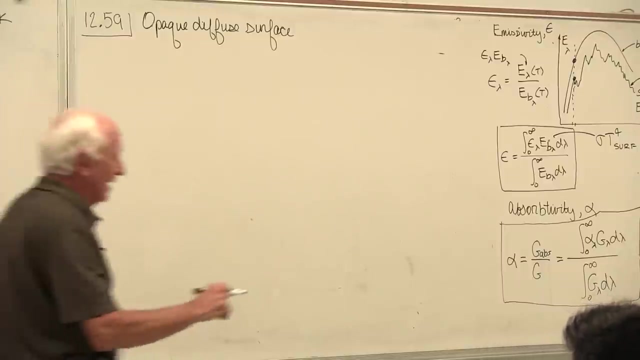 Yeah, Okay, Let's read this one. Okay, Opaque, diffuse surface. Well, just, I'll take this one step further. if you want to complete something, Let's just say. somebody also said fine reflectivity. Well, okay, I'm sure not going to go through this thing right here, because I don't have a graph for. 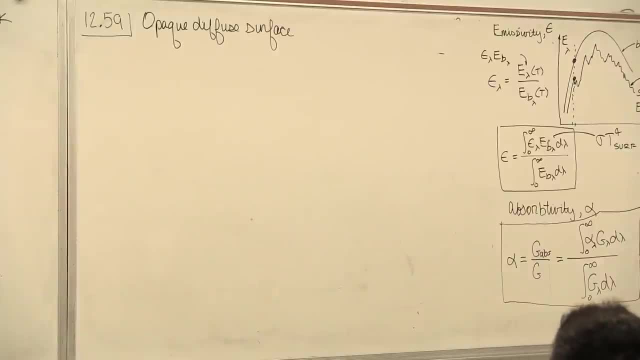 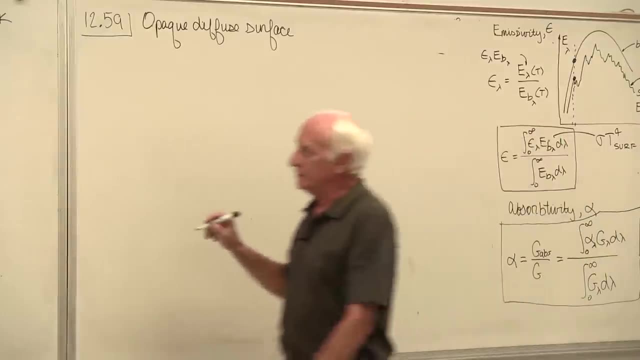 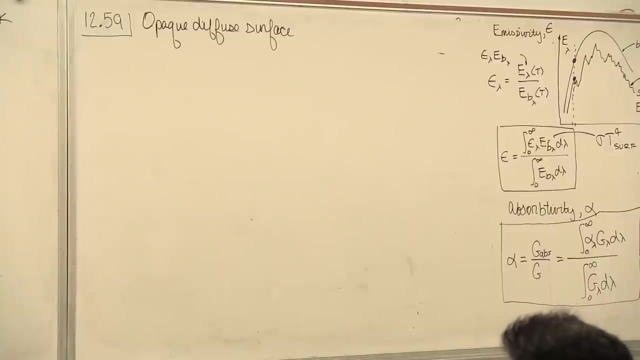 it. I don't have a graph for it. I could get a graph for it, but I don't. But I do know this guy up here. There we go, There we go. Alpha, Oh, magic word: Opaque. 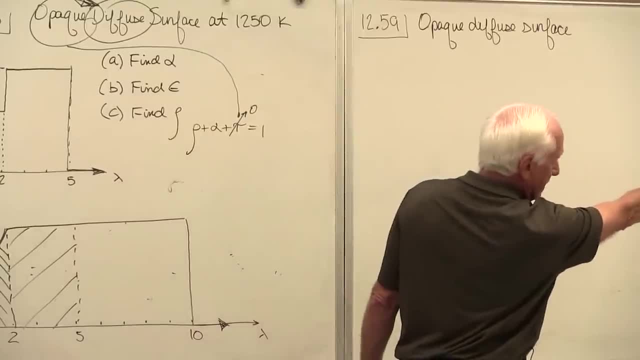 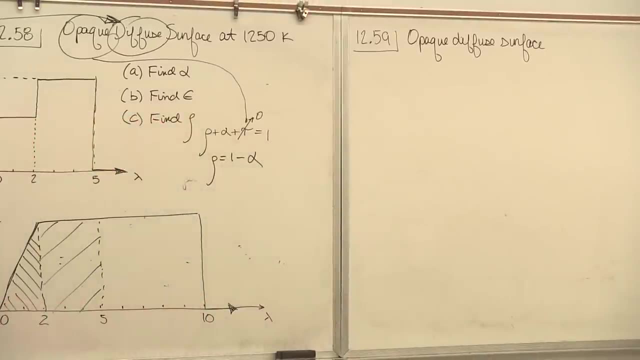 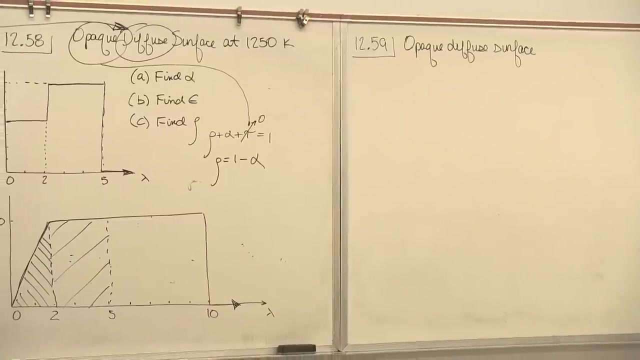 Tau equals zero, Says it over there. Opaque tau equals zero. So what's the reflectivity? One minus alpha. You got it Okay. So now we found all four properties: Epsilon, alpha, rho and tau. Okay, 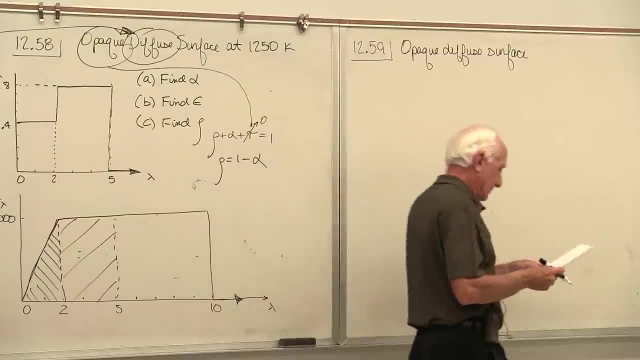 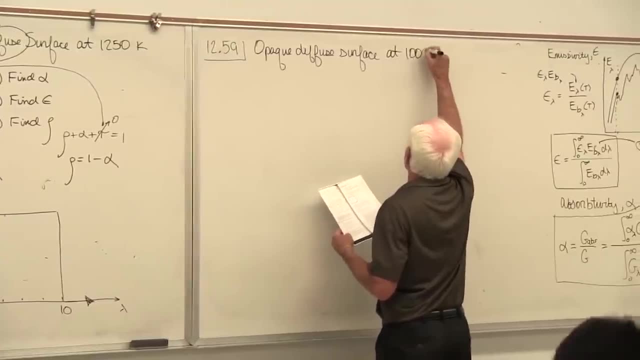 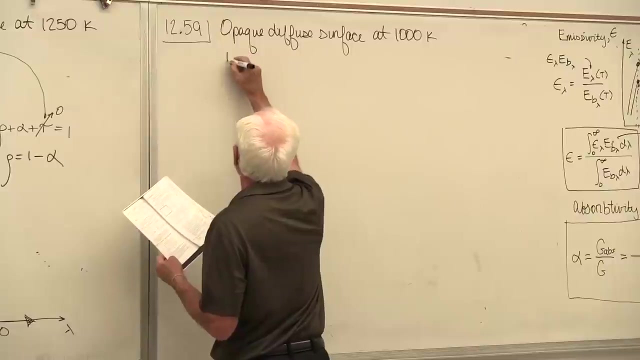 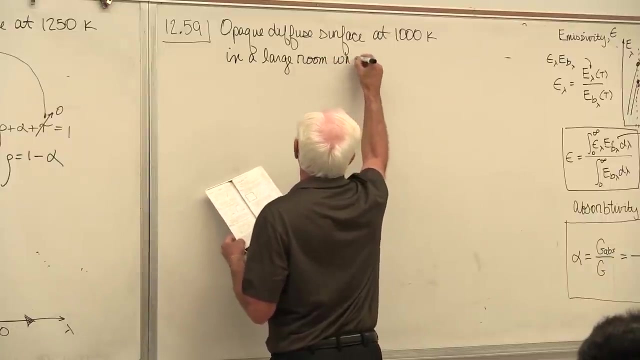 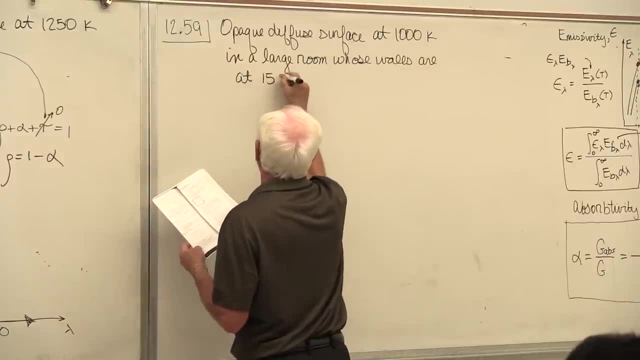 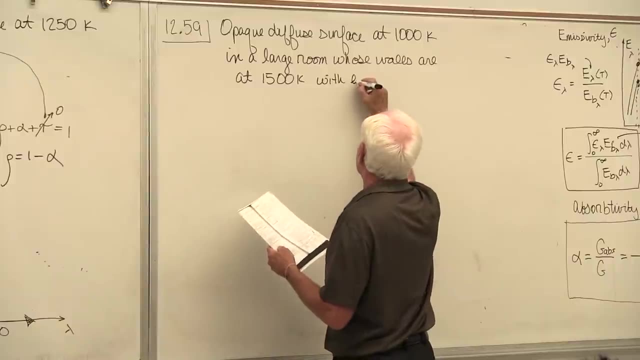 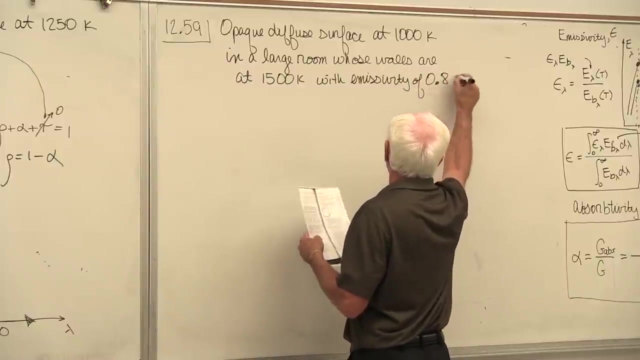 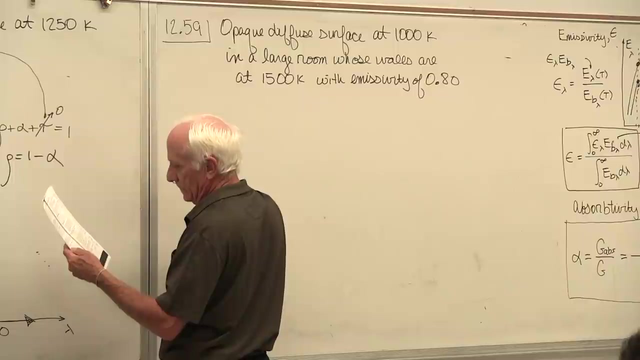 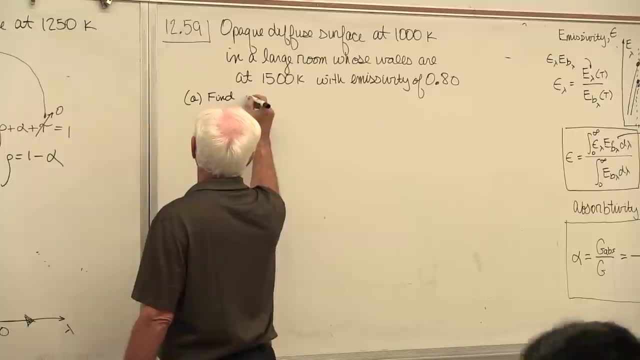 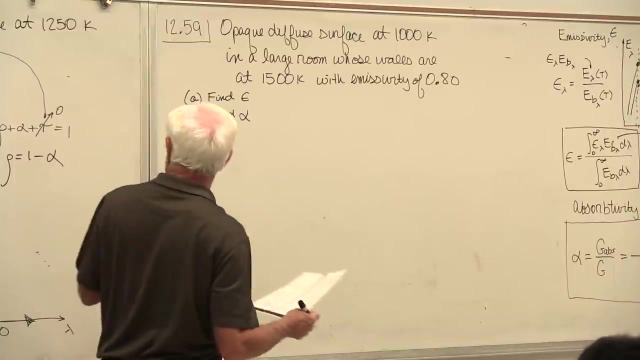 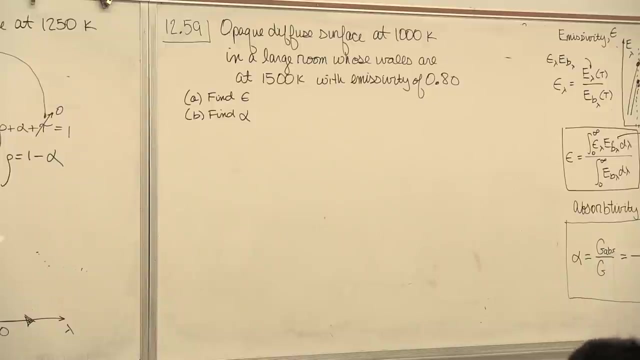 Okay, Okay, Okay, Okay. Okay. Well, let's do the part A first. I'm not going to do part A, I just worked it for this problem. The first part of 1258 said find well. second part said: find emissivity if the surface is at 1250.. 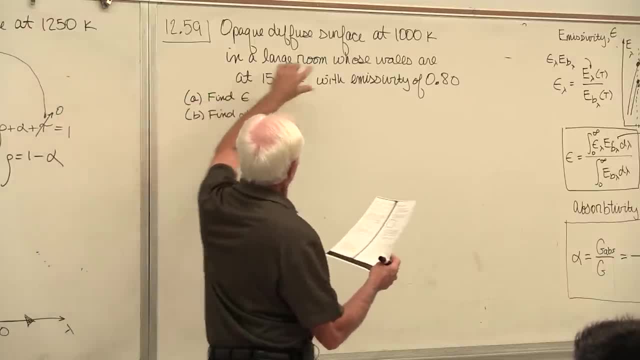 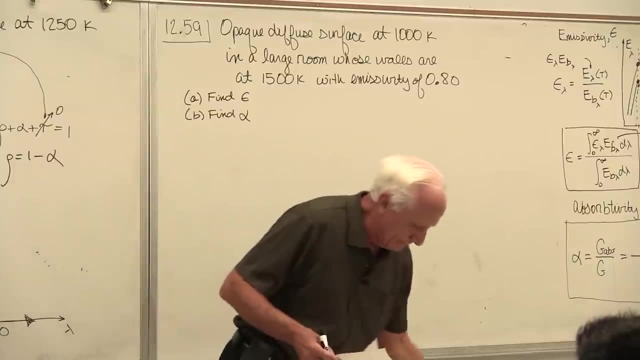 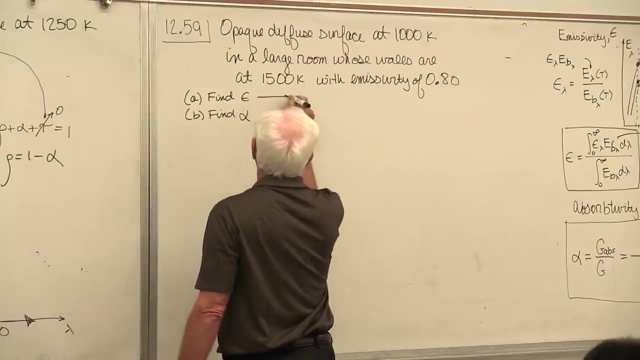 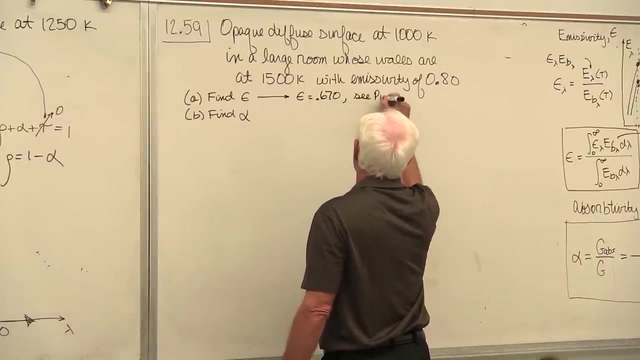 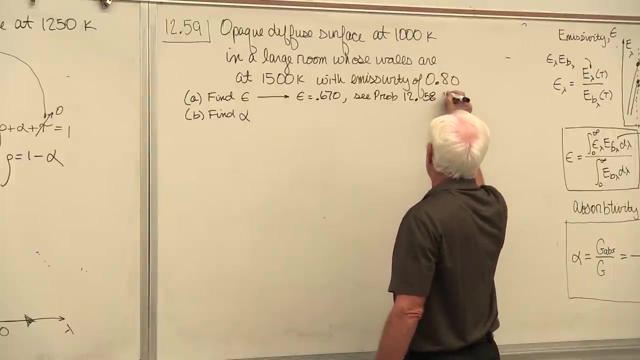 Same thing here. Find the emissivity if the surface is at 1000.. You can do that now. I just worked it for you. The answer is: the emissivity is 0.670.. Zero C. problem 1258, part B. 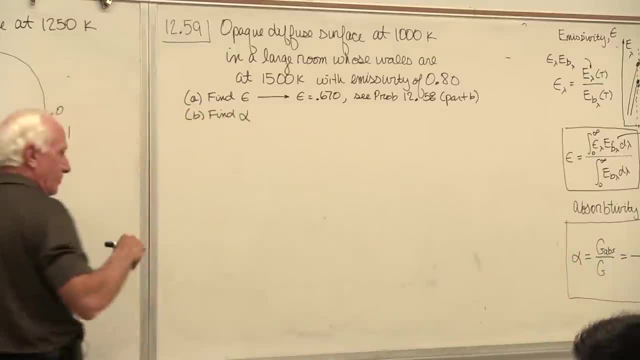 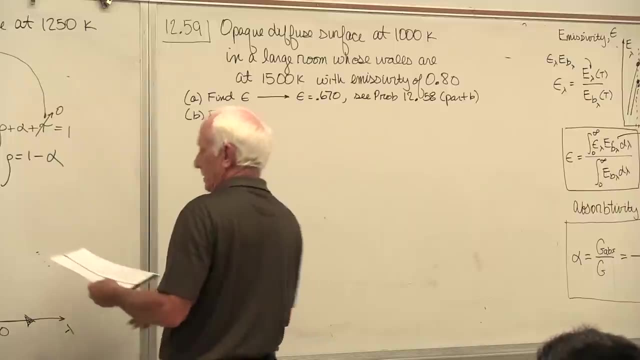 Okay, you can find it just like we found it. You used the table 12 on the fractions of energy, and so on and so forth, So I'm going to draw a picture of what he gave us here, though, and I'm going to put that over here. 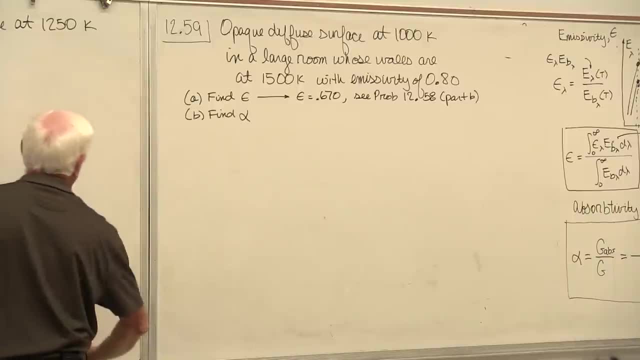 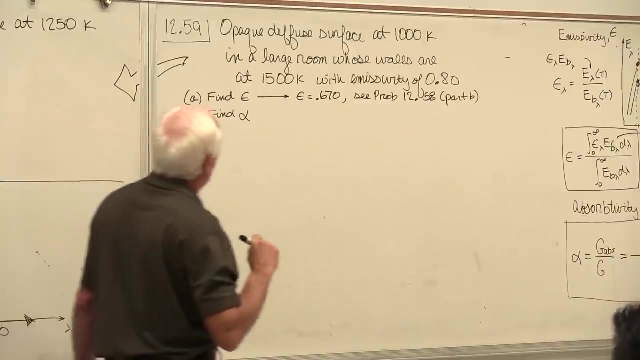 Here. You did just say in the problem with the emissivity of 0.8.. Say it again: Sorry, You wrote With the emissivity of 0.8, so why is it 0.670?? Oh, oh okay. 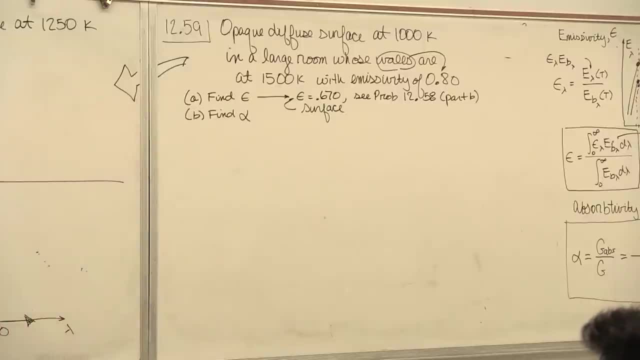 There's a. this is a small object in a large room. The emissivity of the walls of the room are 0.8.. The emissivity of the small object in the room is 0.67.. Okay, There's two emissivities. 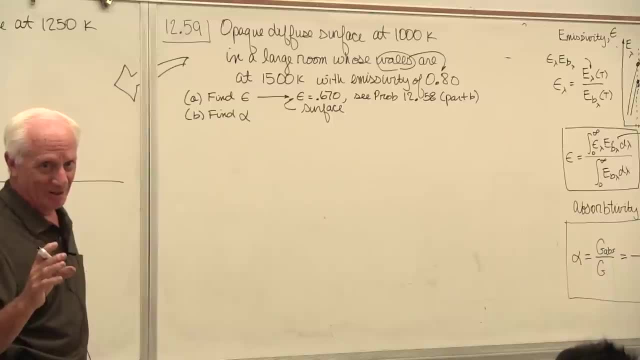 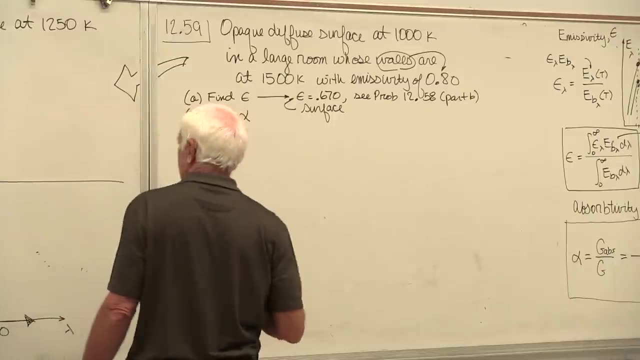 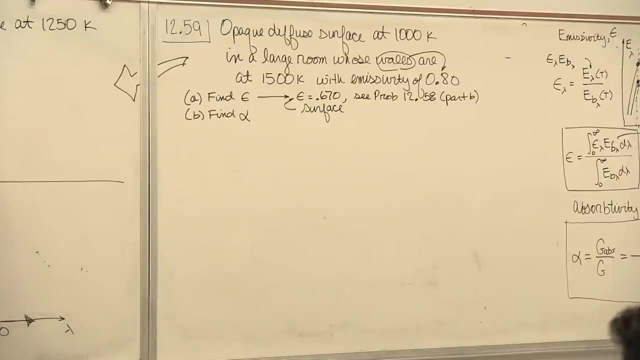 All right, A dime and a basketball. What's the emissivity of the inside of the basketball? What's the emissivity of the dime inside the big basketball? Alpha, Find, alpha. Here's the graph he gives us. He gives us epsilon: lambda versus lambda. 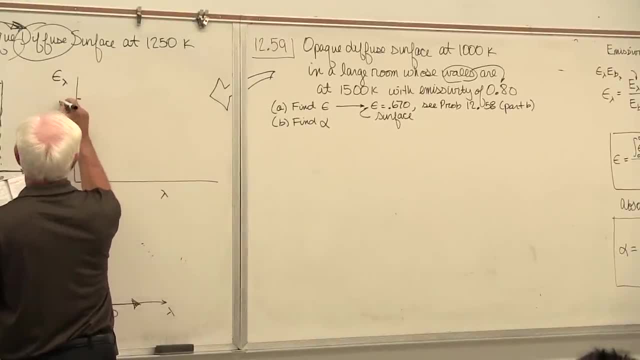 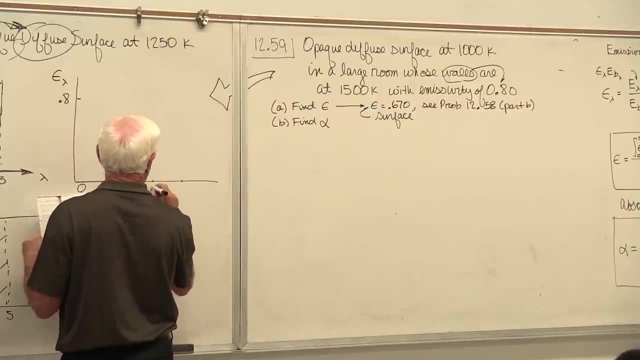 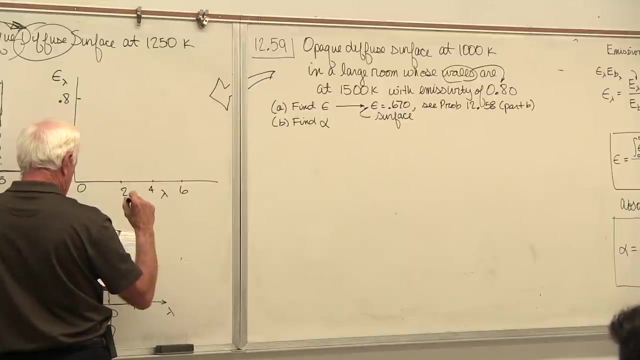 And let's see, we're given eight-tenths up to here: Zero, two, four, Six microns, Okay, And it goes up to six and then down to 0.3.. Goes over to 0.6,, down to 0.3, and on. 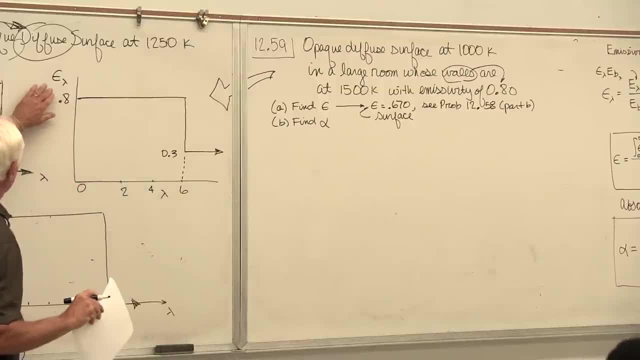 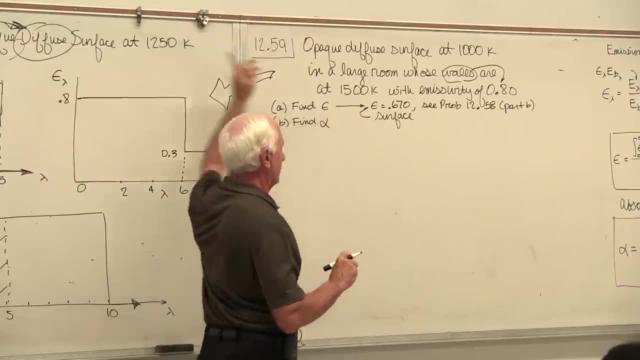 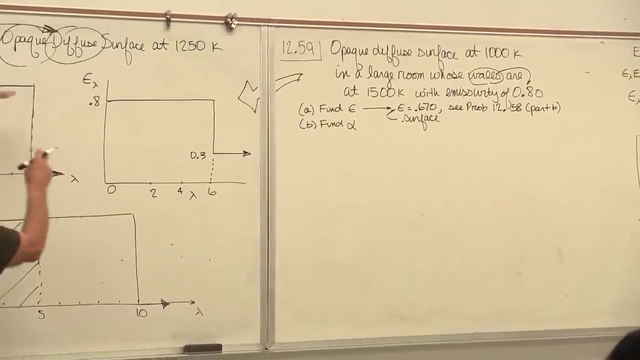 Okay, So we're given in this problem an epsilon lambda, lambda graph. We use that for part A to find epsilon, Just like we did in problem 1258.. Over here, what were we given? An epsilon graph, Problem 1259, we're given what? 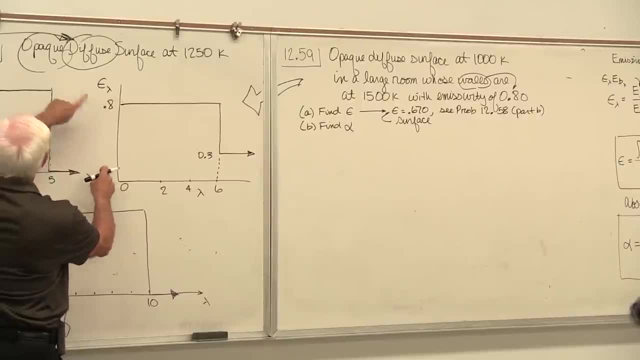 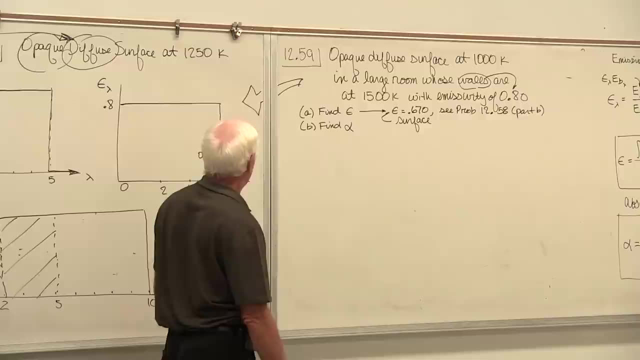 An epsilon lambda graph. What do we do with it? We find the emissivity. We did. We find the emissivity, You can do it. You know the rule. The problem said: oh it's diffuse, Go over there. 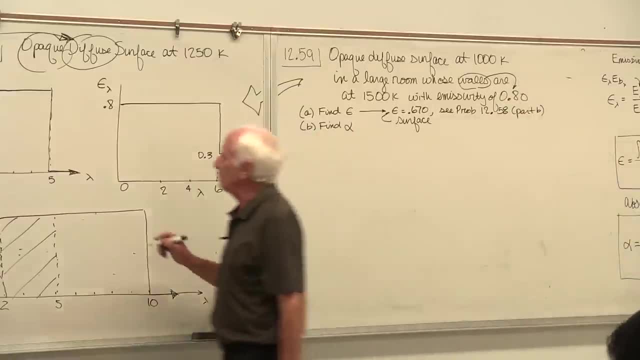 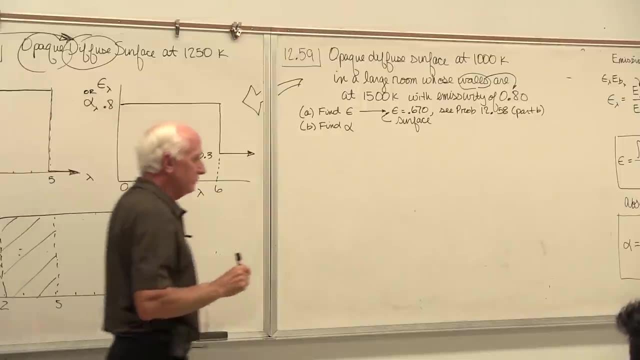 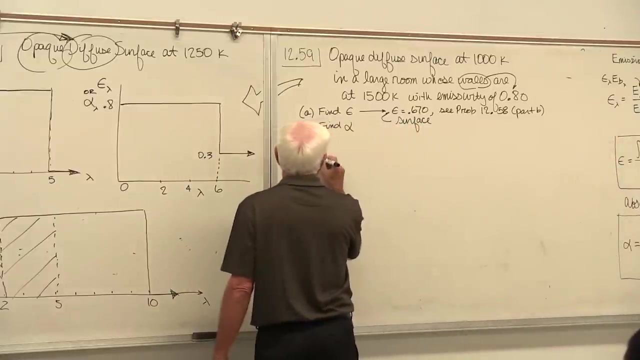 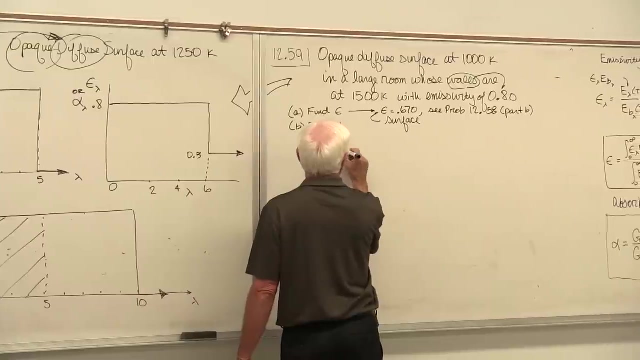 If it's diffuse, then that means alpha lambda. equal alpha. Okay, So this is an equal epsilon lambda. So this is the same thing as epsilon lambda graph. Now you go to the equation for alpha. There it is. Alpha is equal to zero, to infinity. alpha lambda. 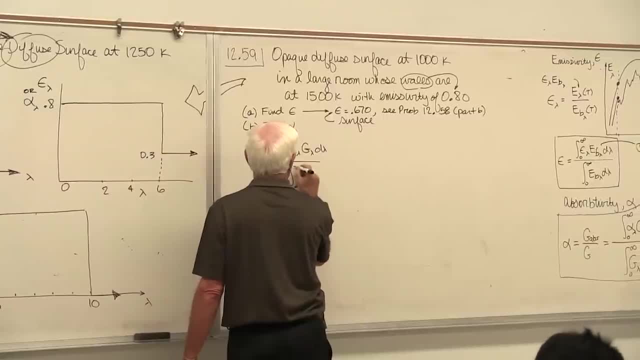 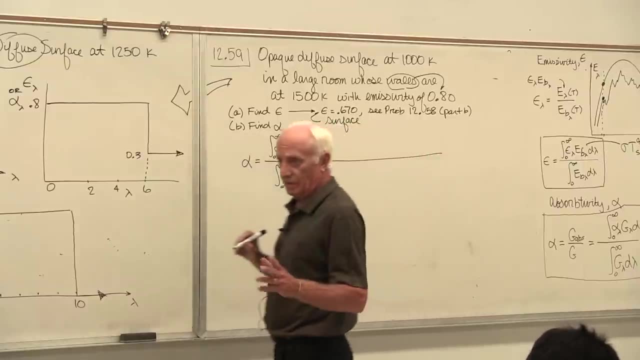 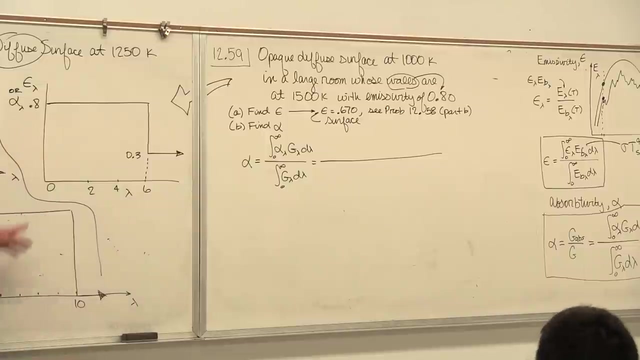 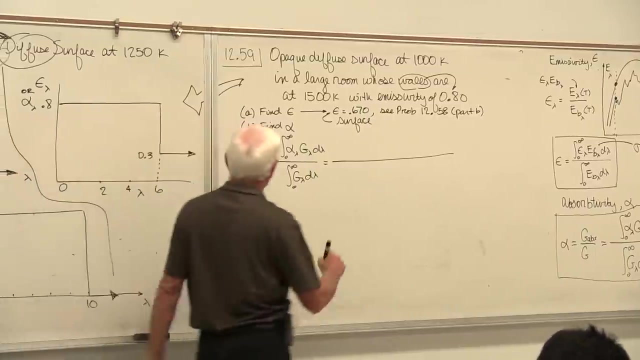 g lambda, d lambda. Now we integrate by parts Wherever there's a break point in the graph. Don't forget now there's only one graph, There's only one graph. There it is Break point six, Six. Next break point: infinity. 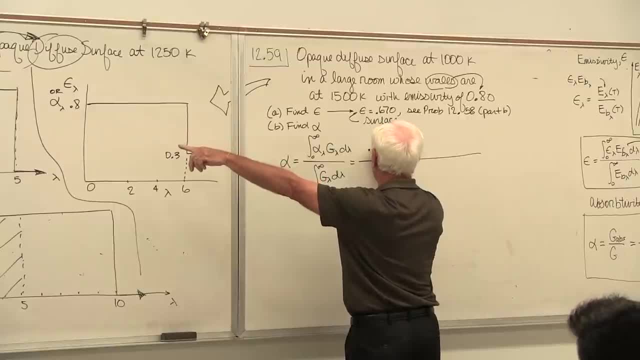 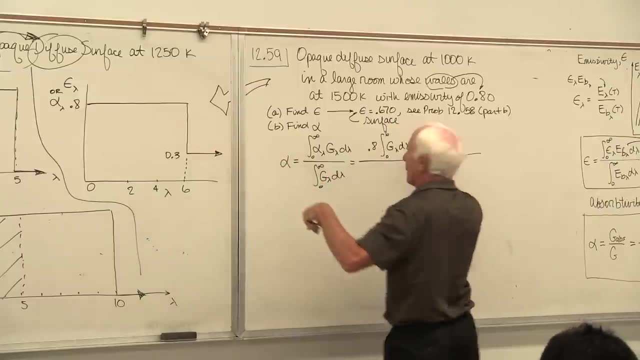 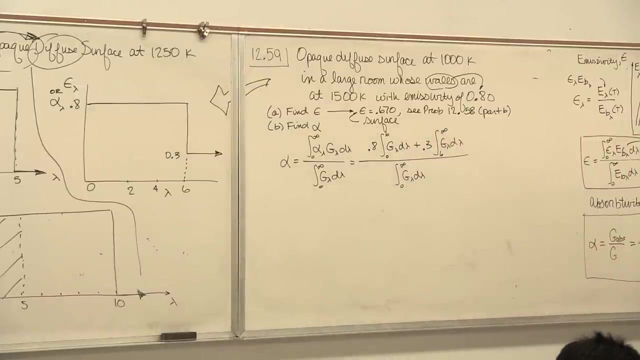 Okay, what's constant? Alpha lambda eight-tenths. Pull it outside the integral sign, Okay. next one, from six to infinity, alpha .3.. Okay, divide it by the difference in the two problems. The first problem gave you a graph of spectral irradiation. 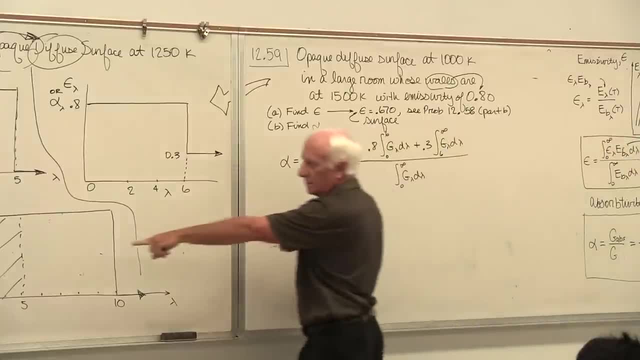 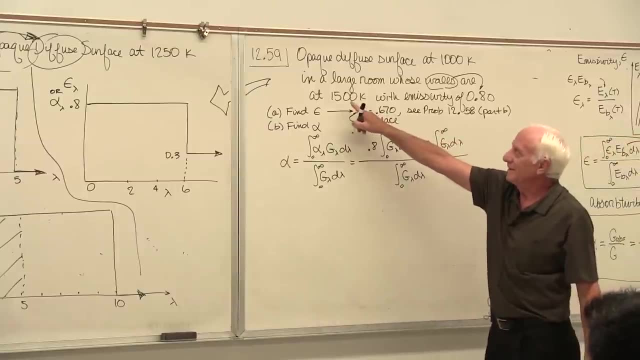 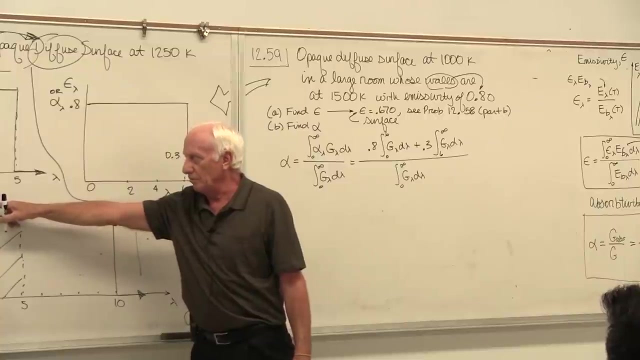 G: lambda versus lambda. The second problem didn't give you a graph, but uh-huh, there it is. It told you the temperatures of the wall in the room. This problem did not give you the temperatures of a wall in a room. 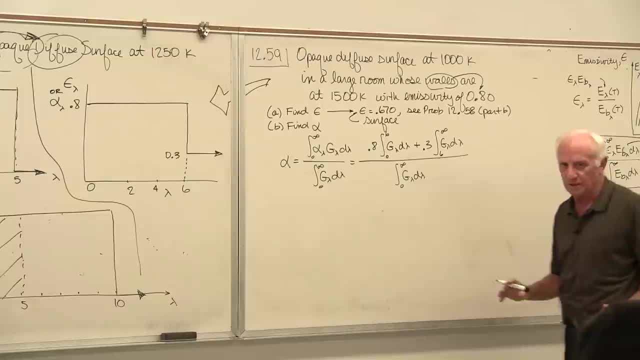 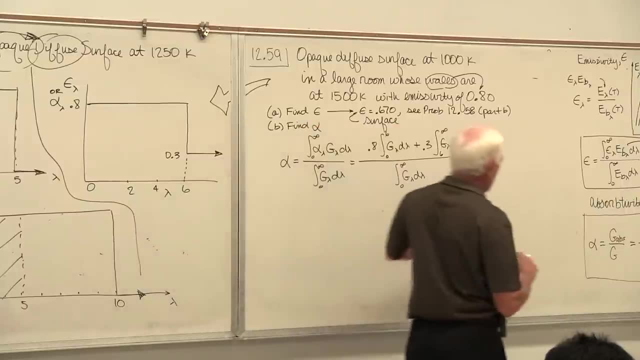 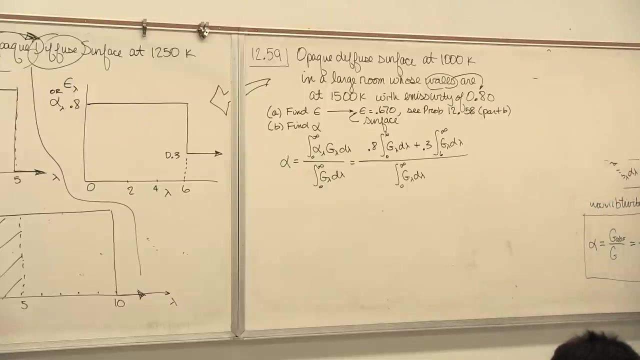 They gave you G lambda versus lambda graphs. They're different approaches to the problems. Okay, let's break it down. I'm going to erase this. We've got this already down. Okay, All right, so that becomes this: 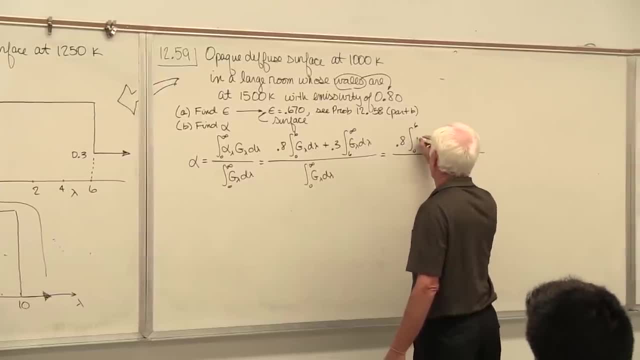 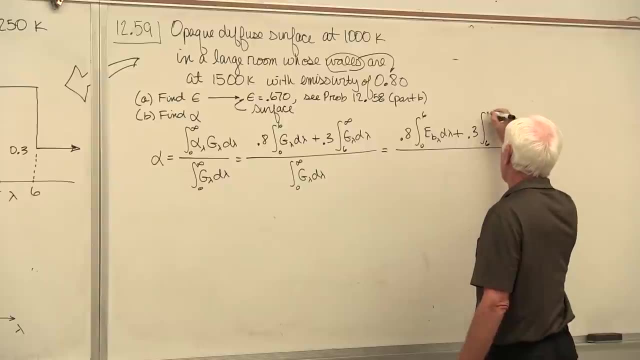 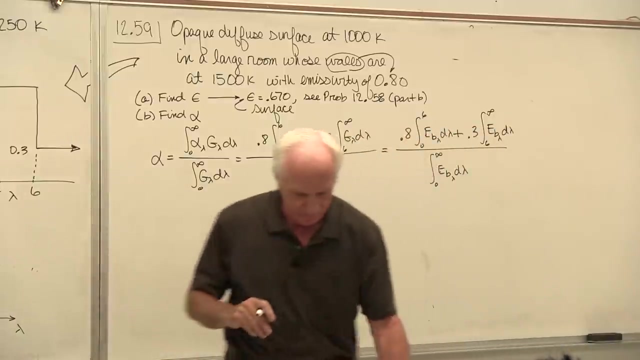 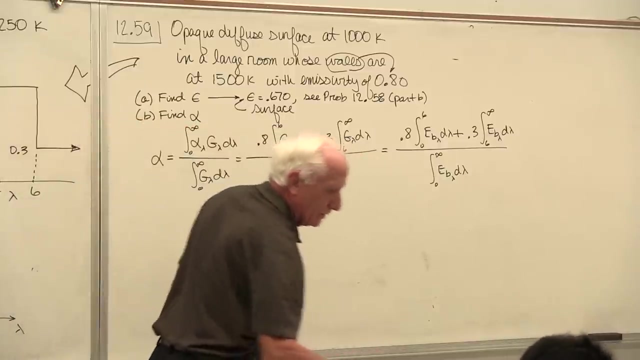 I go over here and say: oh, you know what? 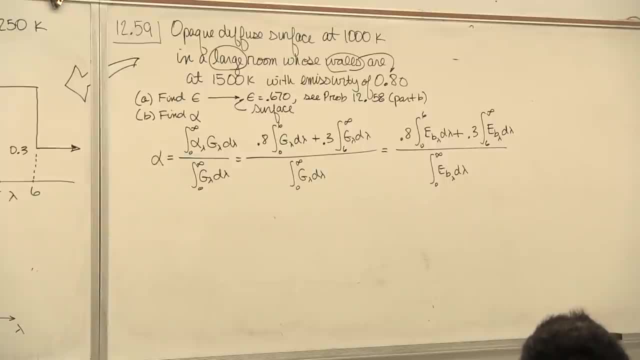 This is a small surface in a large enclosure. Yes, it is, And if that's true, you're allowed to replace the incoming spectral irradiation G lambda with E B lambda. at the temperature of what? The walls in the room? The walls in the room, not the surface. 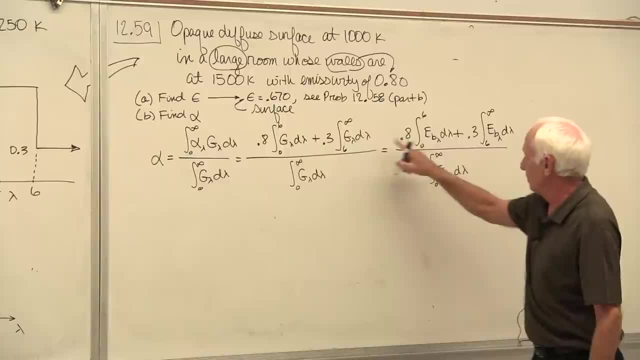 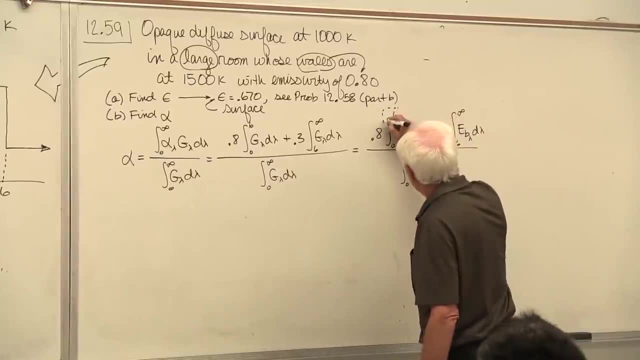 The walls in the room. I did it. I replaced the G lambda with E B lambda because of that picture over there. Okay, And I say you know what? I think I've seen this before somewhere in chapter 12.. Yes, you have. 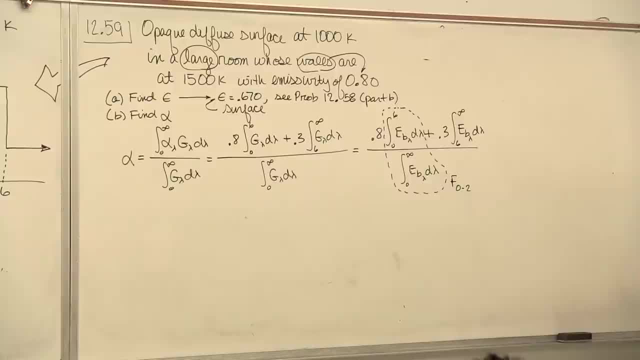 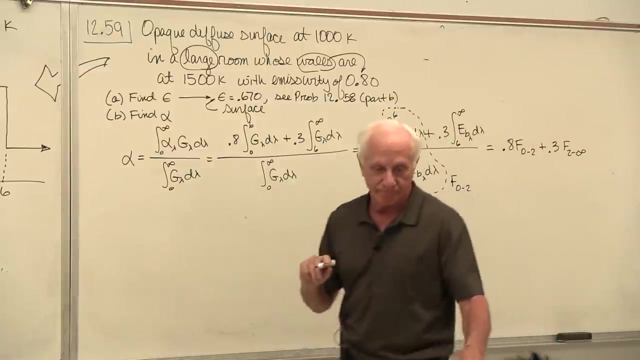 That's F zero to two. Okay, So now this becomes 0.8 F zero to two plus 0.3 F two to infinity. Yeah, See, It's six. That's zero to six. Oh yeah, It's six, yeah. 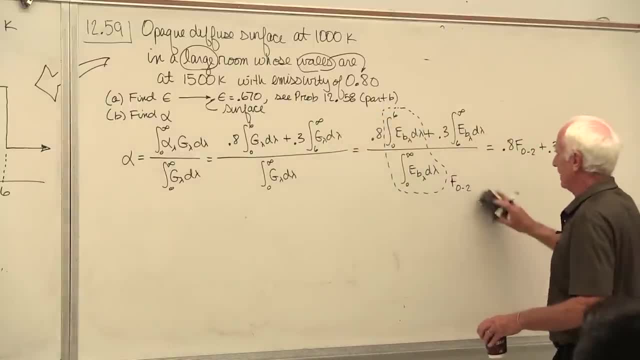 I'm going to go on the picture. Thank you, This guy was six things: This should be six, and that should be six, and that should be six, Six, six and six. Got it, By the way, in the book. he helps you. 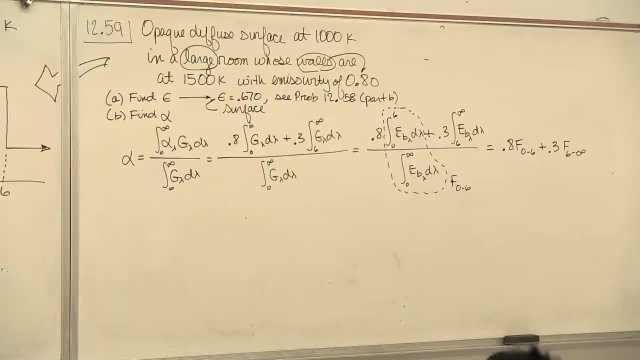 If he means that this, that G lambda, is zero after 10, there's a, he puts a red line in the book. This is a red line. That's a red line. That's a red line. That's a red line. 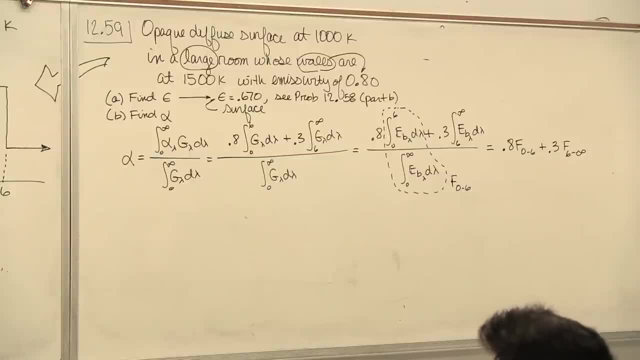 And he puts a big fat red arrow like that arrowhead, That means assume it's zero all the way to infinity. When he puts the big fat red arrow here, that means assume that epsilon lambda is 0.3 all the way out to infinity. 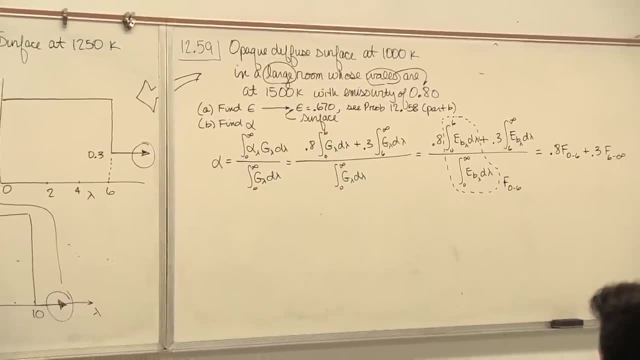 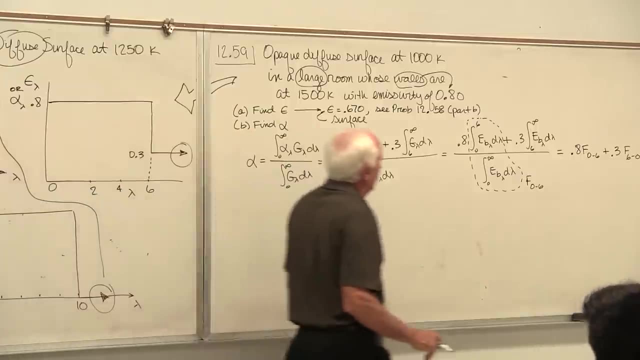 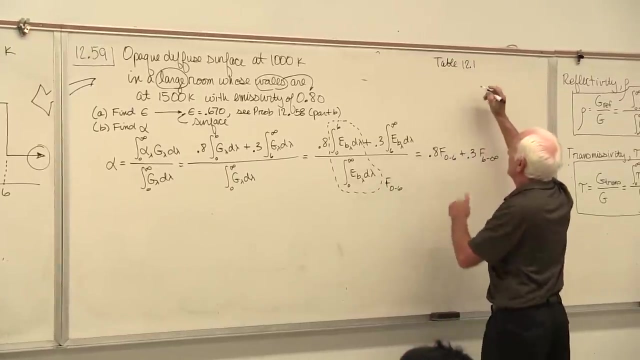 so you know there's no more breakpoints in it. The big red arrowhead indicates it goes out horizontally to the right until infinity. Okay, Table 12.1. again, We have to get lambda 1t and lambda 2t. Well, this guy is infinity. 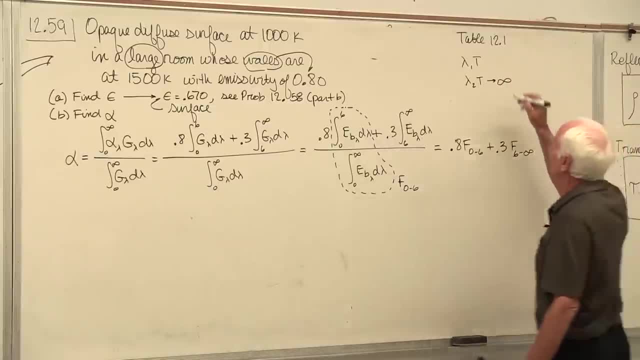 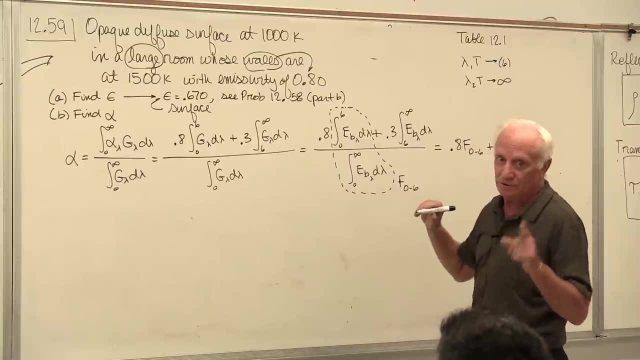 The second lambda is lambda equal infinity. The first lambda is equal to six. So we have six times the temperature. Now you got to be careful. There are two temperatures given here and don't make a mistake. If you don't make a mistake on them, do you use 1,000? 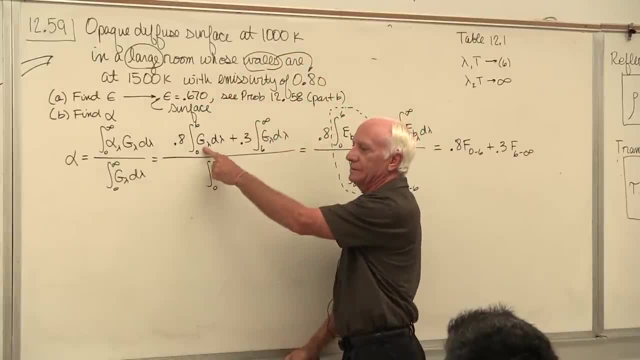 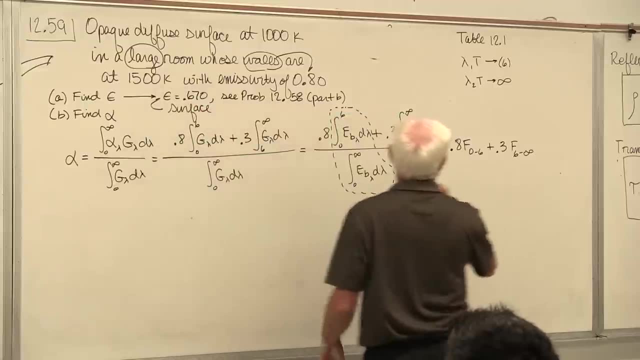 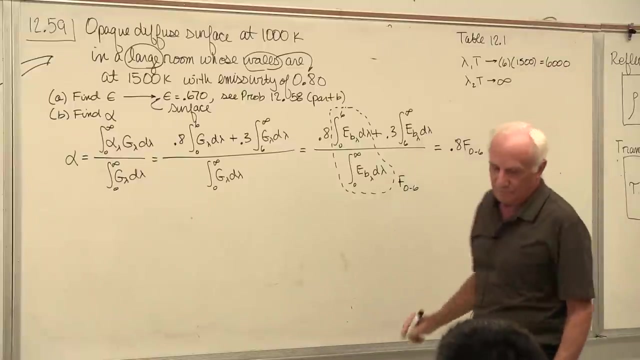 or do you use 1,500?? You're saying this is the irradiation. Where did the radiation come from? The walls of the room? Oh, 1,500.. Okay, So get the right temperature and there's two choices. 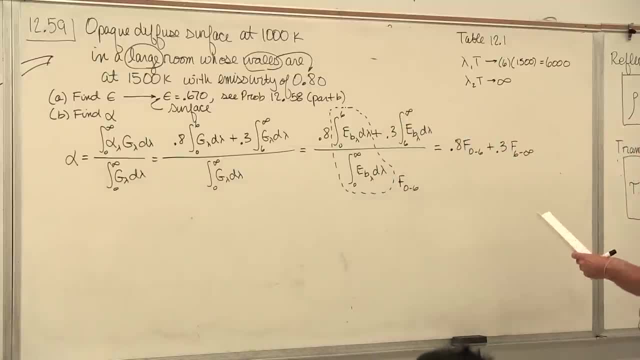 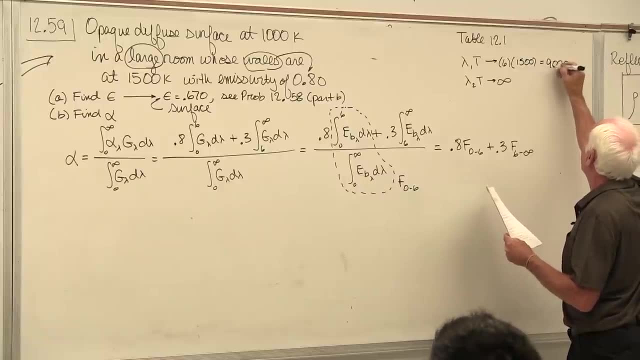 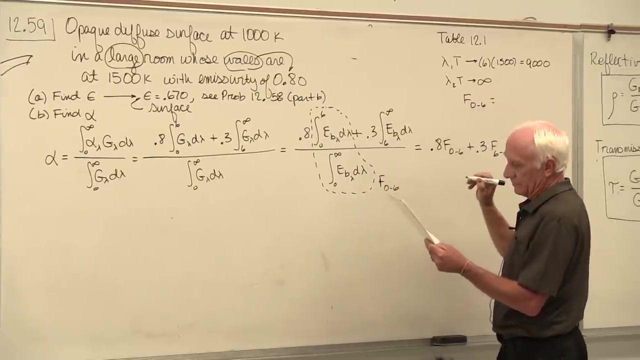 The surface temperature or the room wall temperatures Six times 1,500.. Six times 1,500.. That won't do it. How about nine? All right, So let's do the F's then. F zero to six from the table: 12.2 is .890.. 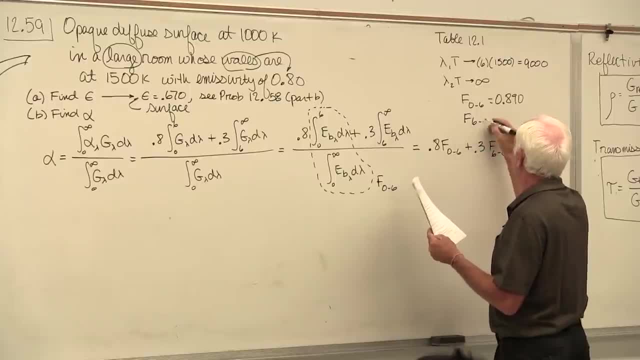 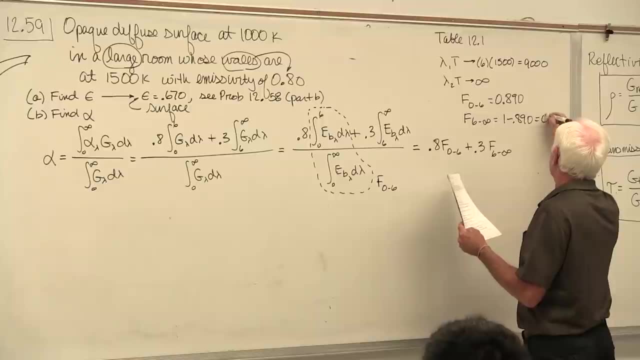 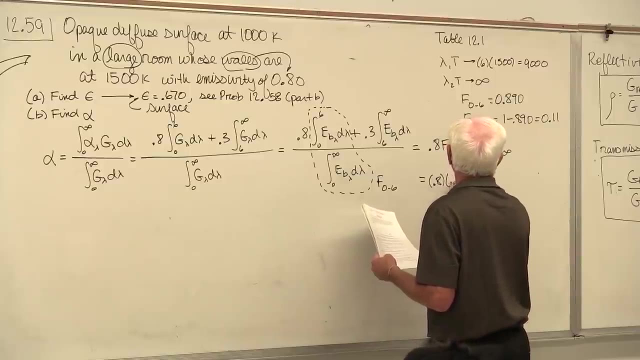 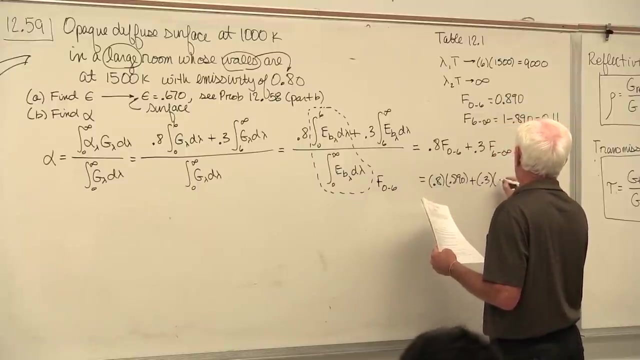 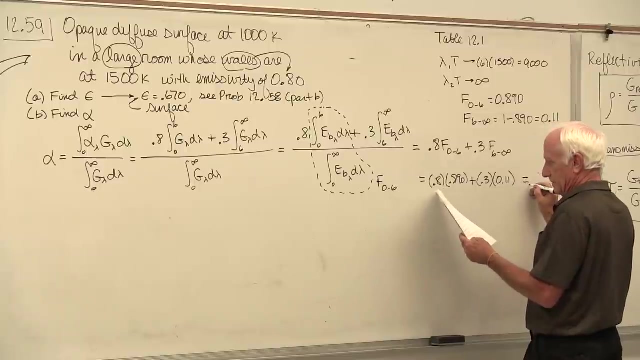 F from six to infinity is 1 minus .890.. One one, All right. So this becomes eight-tenths, three-tenths, So alpha then comes out to be 0.745.. Notice from part A: even 70.7.5.. 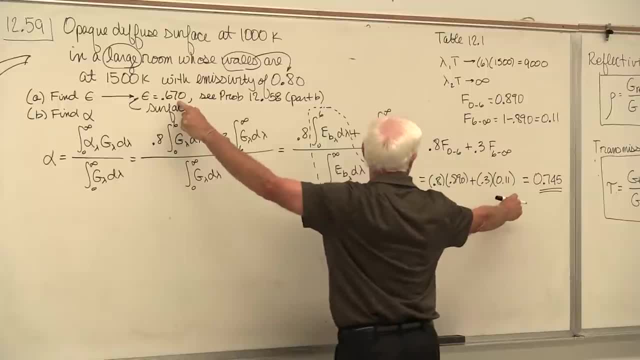 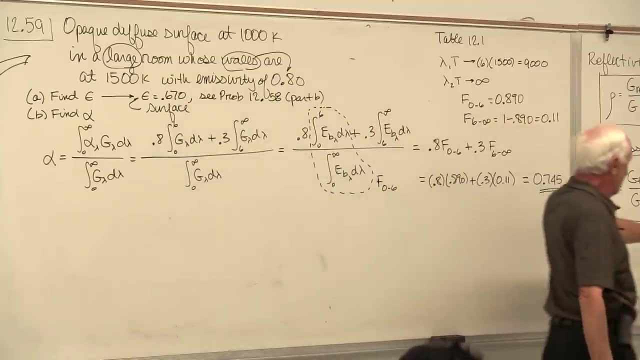 All right, So this becomes 70.670.. Part B: absorptivity: 0.4, 0.745.. They're not equal. Why aren't they equal? Because nobody said the surface is gray, Just like problem 1258.. 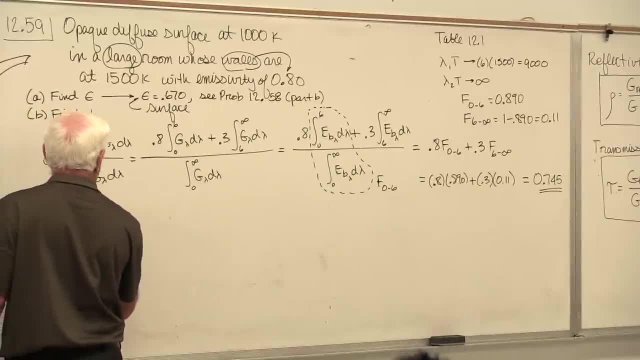 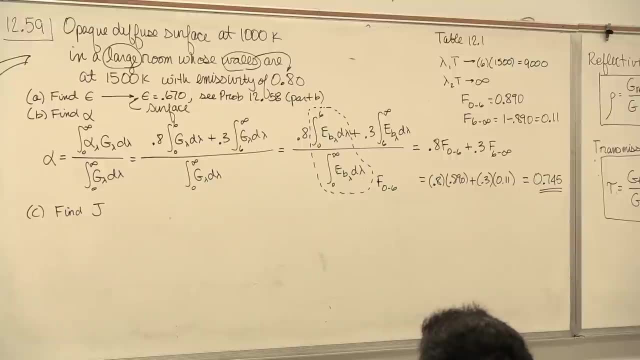 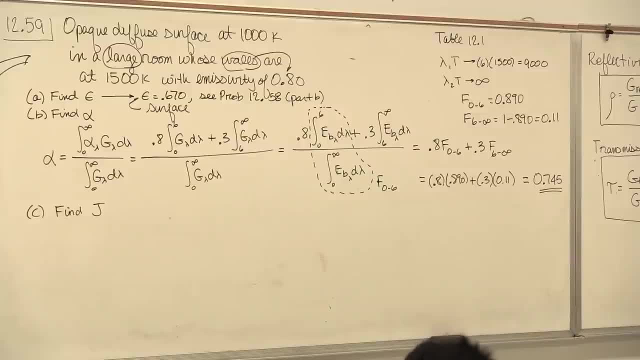 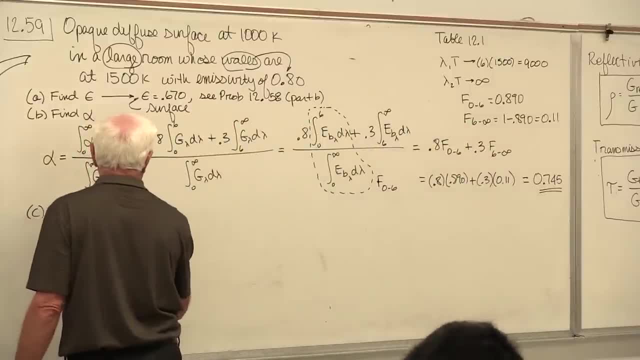 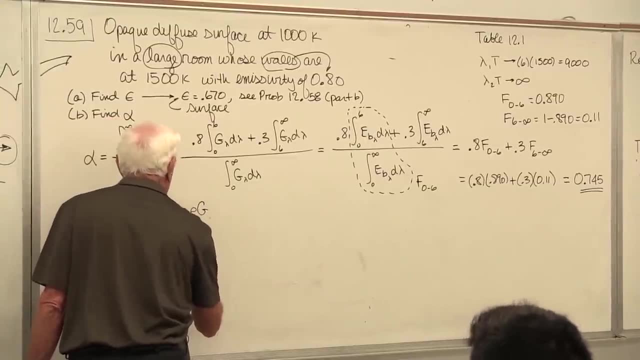 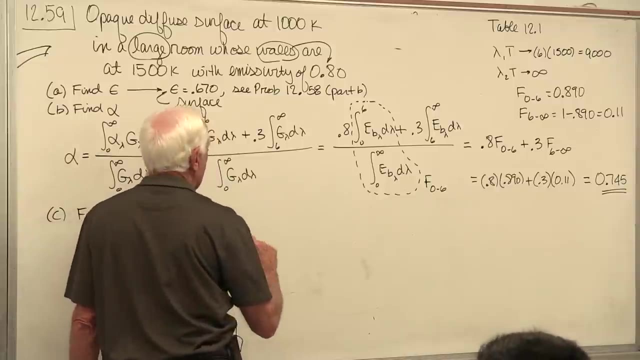 Okay, So J equal, E plus rho, G. All right. So what is E? This is epsilon, sigma T to the power zero, E to the fourth plus rho. Do I have rho? No, Did it say opaque? Yes, it did. 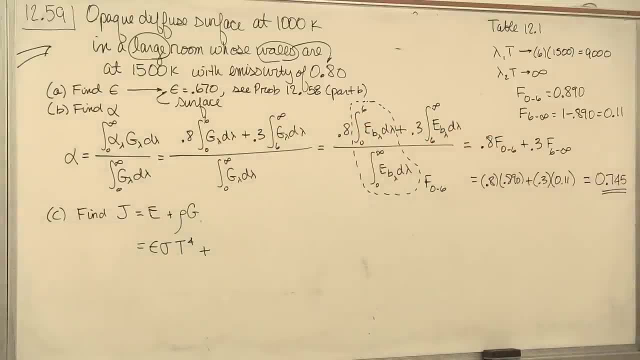 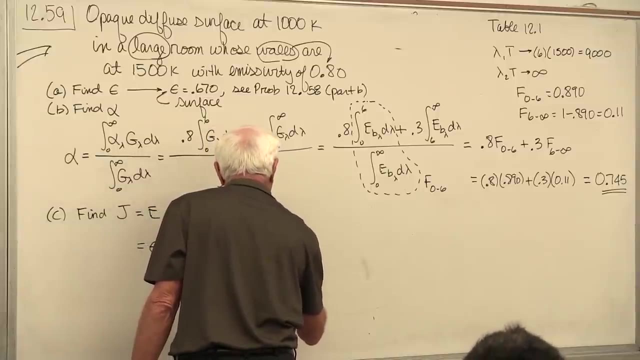 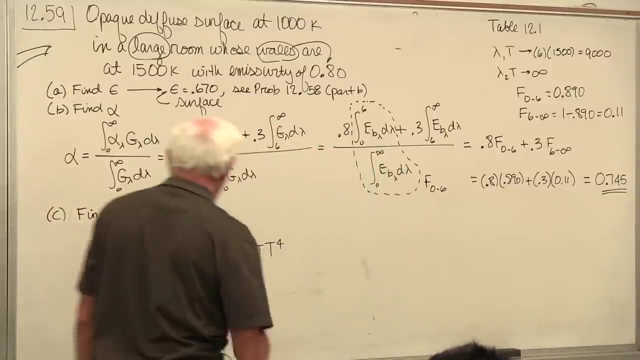 If it's opaque, what do I do? I put tau equals zero here, and if I want rho, rho is equal 1 minus alpha, and I just found alpha. I forget it. So why is it though? why would it be 0?? 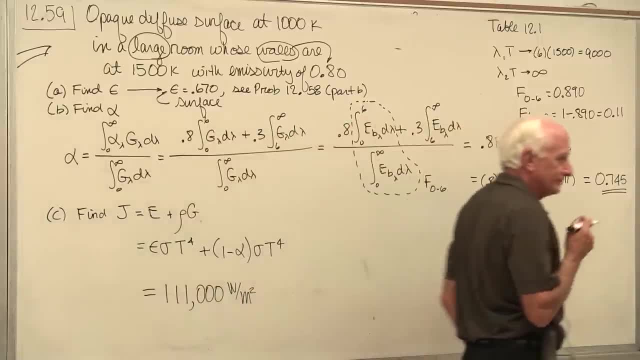 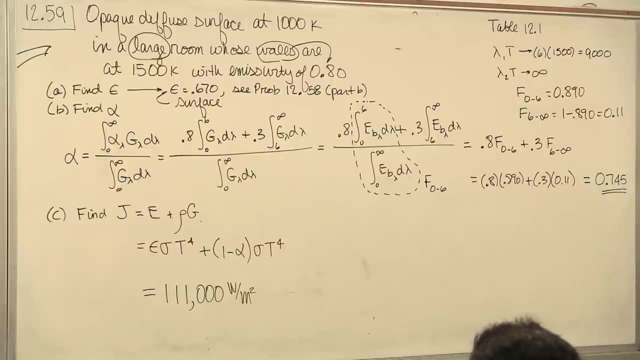 111,000 watts per square meter. 111,000 watts per square meter. Why did I replace G with sigma T to the fourth? Look at the picture again. From a small object in a large enclosure, G looks like it comes from a black body at the template. 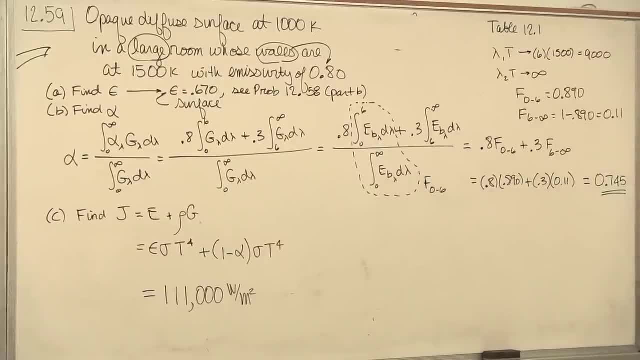 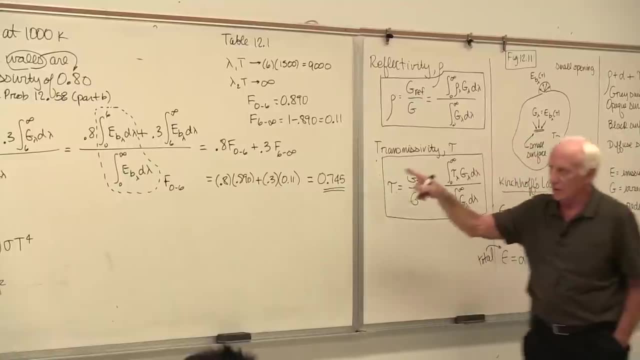 If I put rho, rho and you put sigma E, it becomes rho, rho, rho. That's from a large enclosure. so that would have taken some space to get here, because that's the temperature of the housing body. at the temperature of the walls, A black body. sigma t to the fourth, But you better. 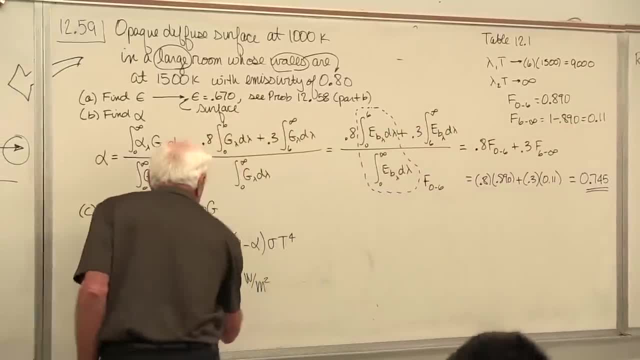 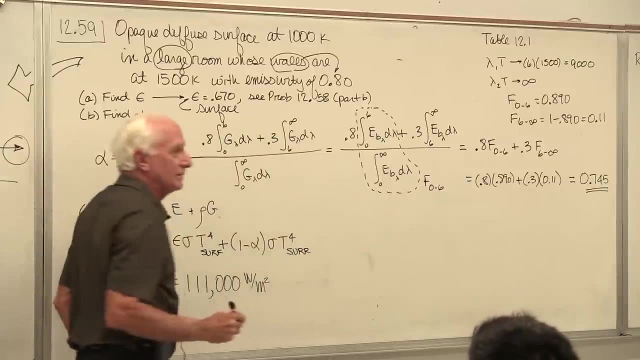 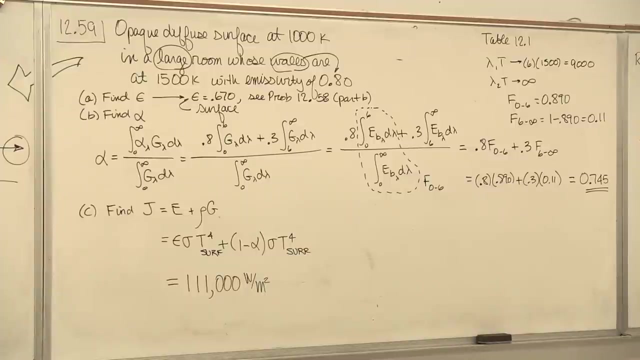 be careful. This is temperature of the surface and this is temperature of the surroundings. Don't put the same temperature in for both of you. you'd be dead wrong. There's two different temperatures in this problem. You can see the contrast of these two problems I put on. 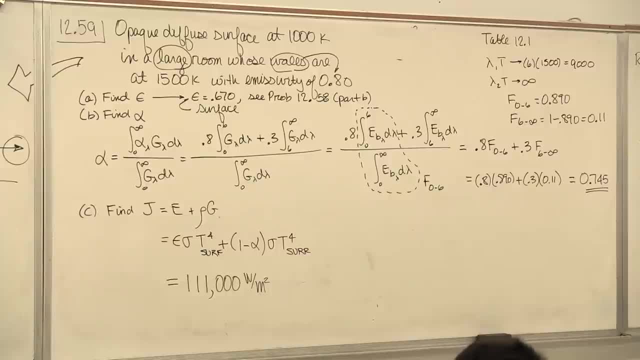 the board. The first problem: somebody can give you a graph of epsilon or alpha or rho or tau. Okay, Then they'll tell you they could give you a graph of the incoming irradiation G. They won't tell you this- the temperature of the surroundings. They won't say it's a. 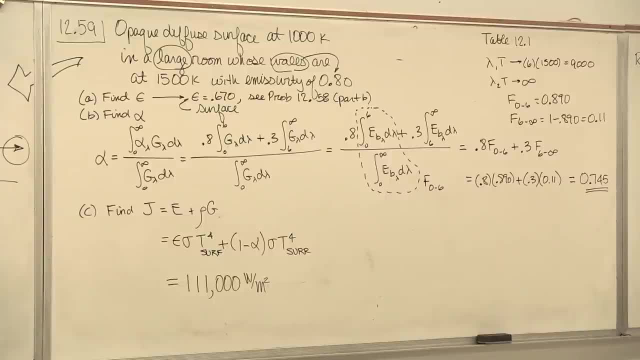 small object in a large room. no, This problem. they'll give you again a graph of maybe epsilon or maybe alpha, maybe rho, maybe tau. They'll give you a graph, Here it is. Then they won't give you a graph of the incoming radiation, spectral irradiation They'll give you instead. 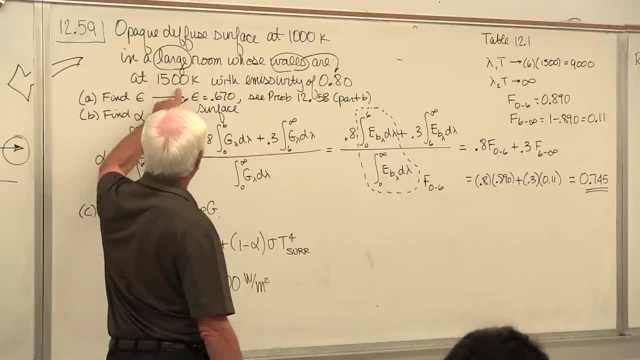 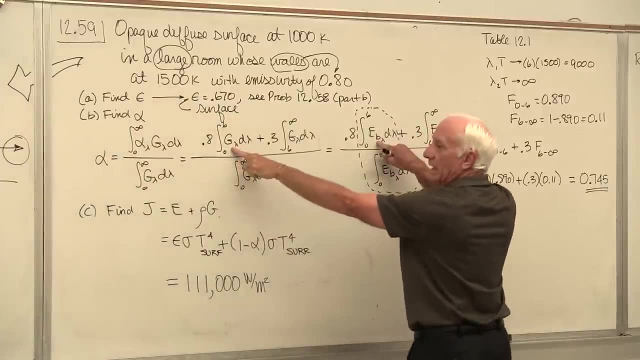 the words either a small object or a large room and tell you what the temperature of the walls in the room are. That's when you can replace the g lambda with the eb lambda. Did we get the term? Yeah, Okay, Yeah, Yep. 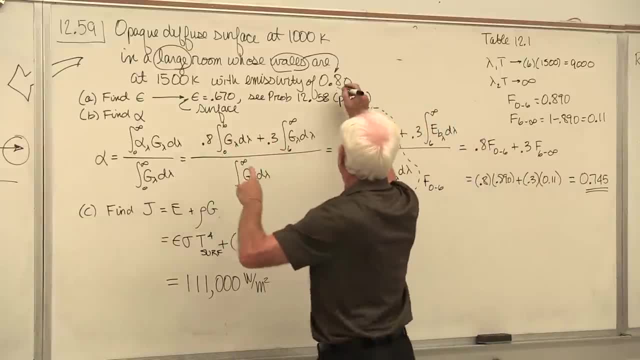 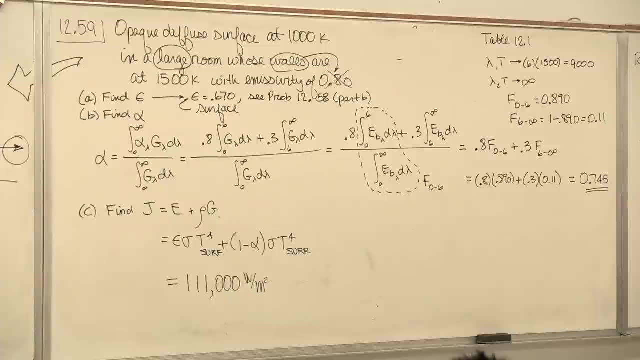 Okay, Okay, Yeah, Right, Okay, Okay, Okay, Okay. Now it's the results again. It should be a little different, Okay, Okay, Okay, ever use this Nowhere. It's not needed, It's just flag. You don't use that. 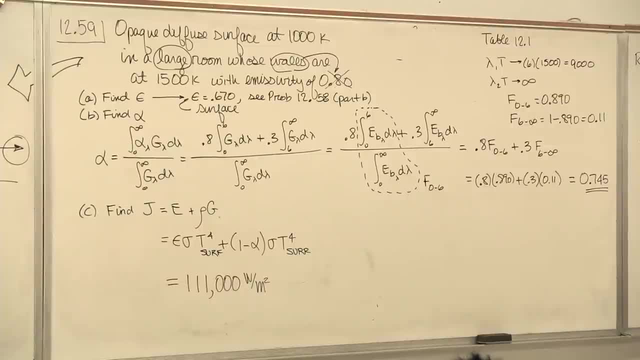 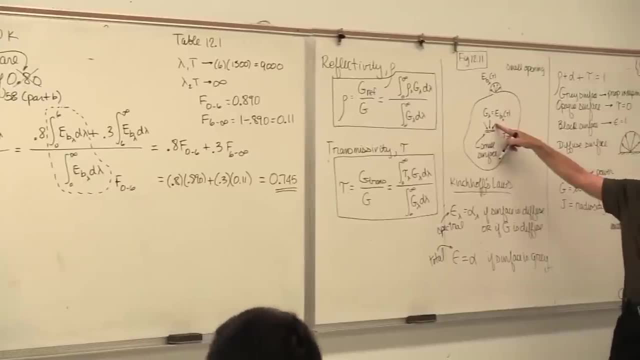 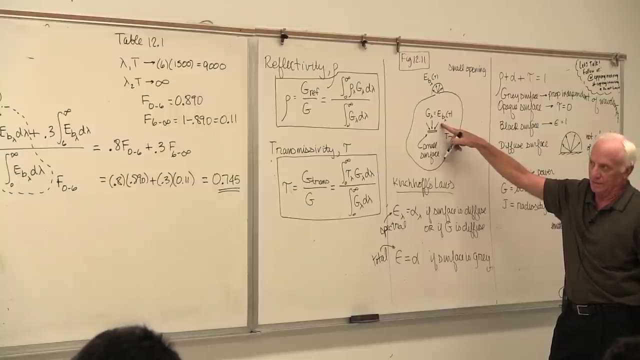 Because if you read the words below Figure 1211, it'll say that this is true irregardless of the emissivity of the walls in the room. This is true irregardless of the emissivity of the walls of the room. It doesn't matter. Change that. 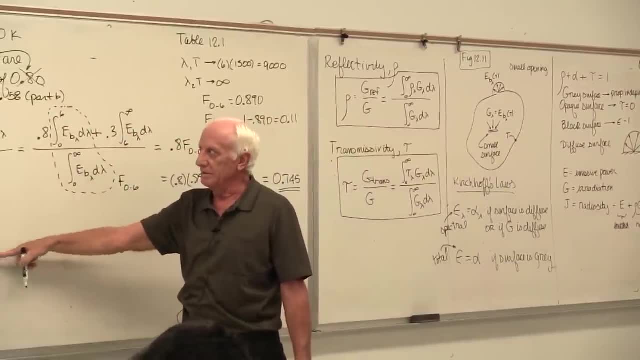 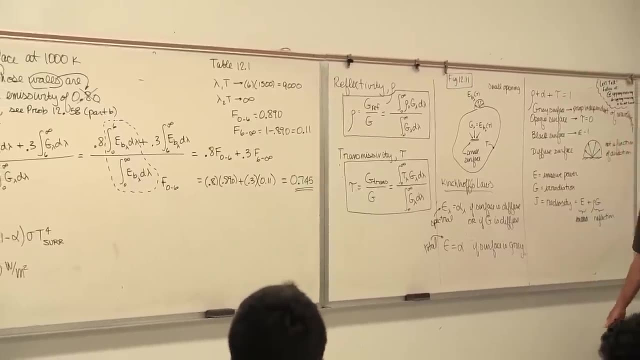 to point one, These answers are still okay. Oh yeah, Chapter 12 is not straightforward. Oh yeah, that's really clear. I see that. No, that's not the way it is. Chapter 12 is the toughest chapter in the whole book to read and understand. 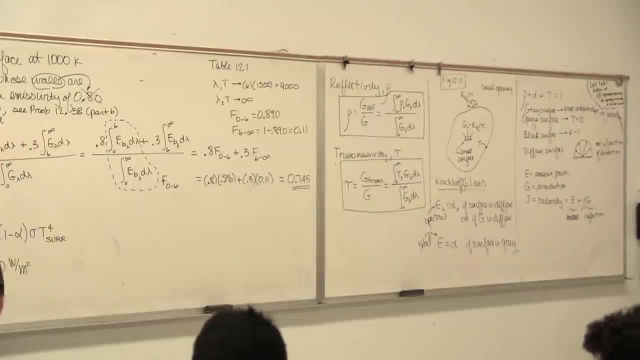 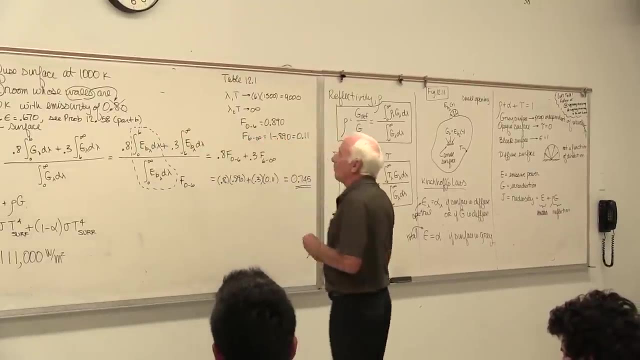 That's why you want to go by the notes here and then fill in what you want to fill in from the notes with the textbook. But start with a good set of notes. That's the key. Okay, homework is very similar to that. 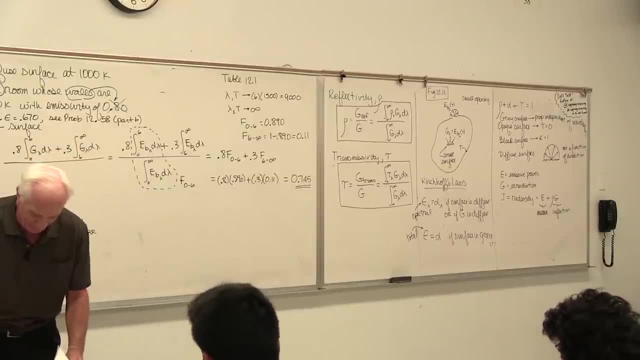 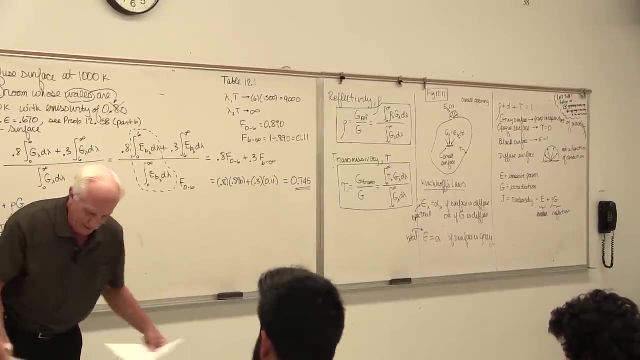 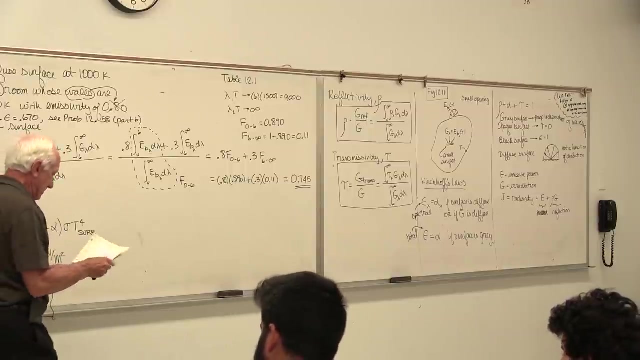 Alright, so that pretty much ends Chapter 12.. And we're going to start Chapter 13 on Friday, But I want to go over the homework problem that I passed back and graded, So let me go ahead and put this up on the board here. 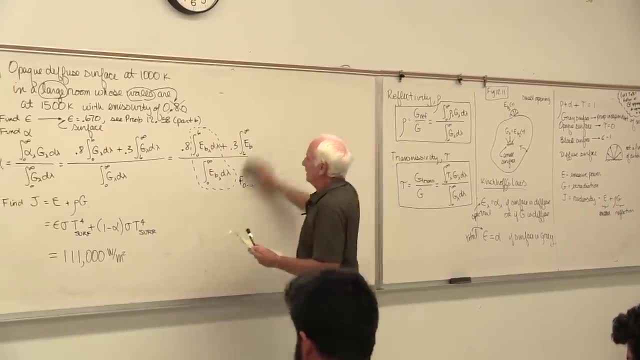 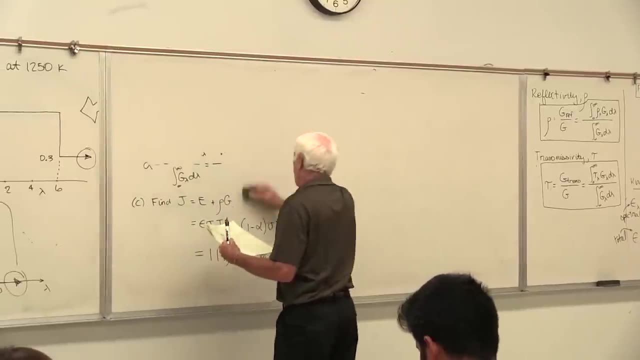 Okay, I graded the first problem because it was a combination problem of a little bit of analytical work and a little bit of graphical work, So I wanted to see both on a problem. So that problem had both. I'm not going to go over. 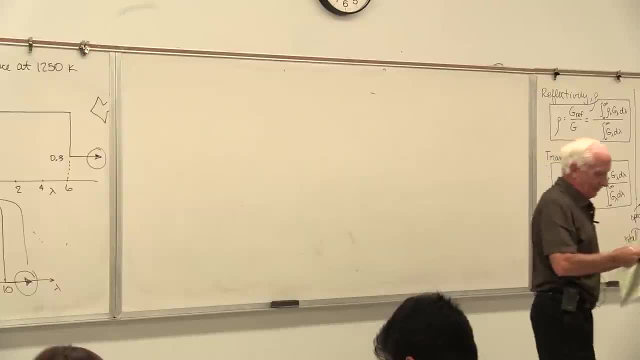 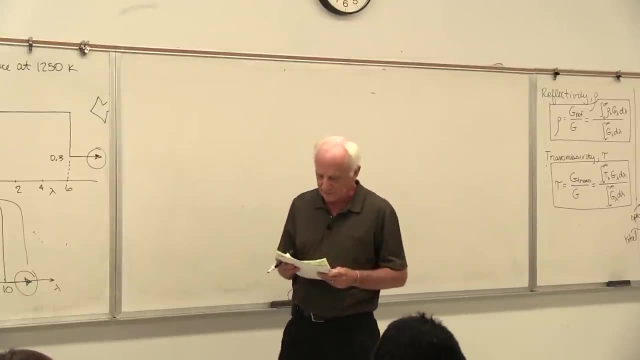 the analytical part. Most people got that right. Find the shape factor from the table, Put it in the equation for Q, S, K, delta, T, Bam, that's the answer. But I do want to go through the graphical part because 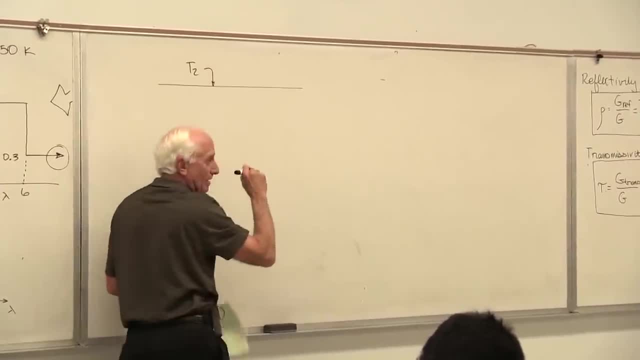 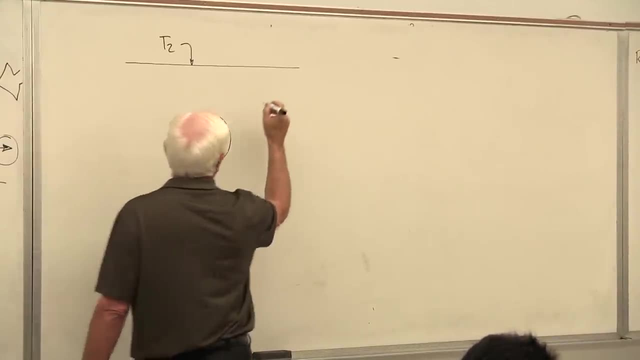 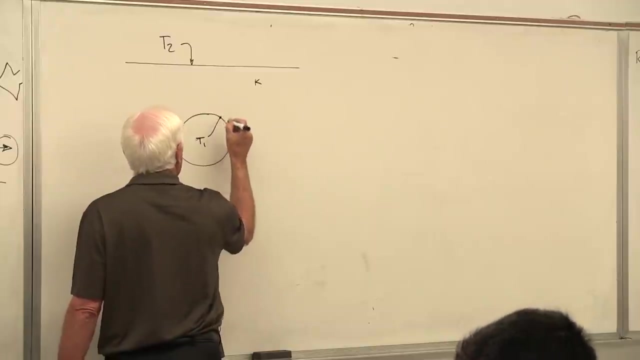 some people had a problem with that. So this is a sphere that's buried in soil And the temperature of the sphere, we'll assume, is T1 on the inside surface of the sphere. I'm going to do a two-dimensional drawing of this 3D picture. 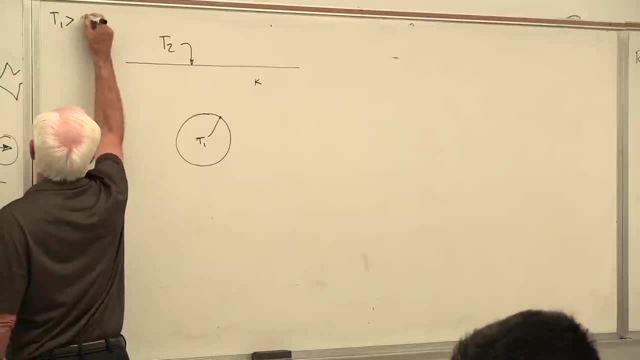 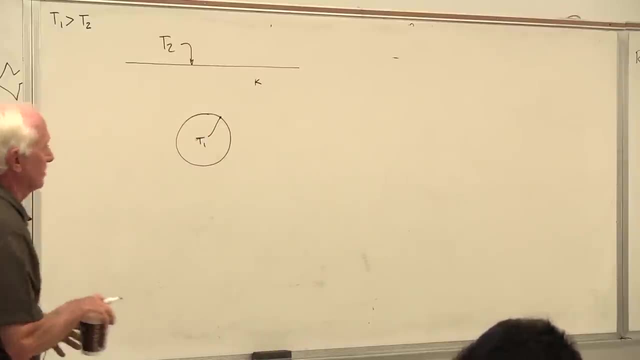 I'm just going to assume that T1, just to talk about something- T1 is greater than T2.. It would make no difference if I said T2 is greater than T1, but I'm going to say I'll assume the sphere is hot. It probably is. It's radioactive. 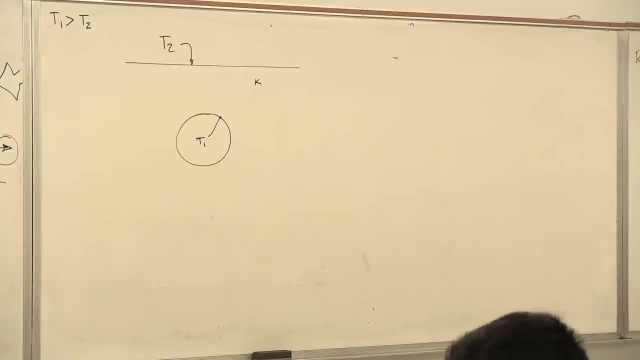 material, And the soil surface too, is cooler. T2 is cooler. Okay, Draw a heat flux plot. You don't need to draw curvilinear squares. I'm not going to do an analysis for that, Just draw the heat flux plot. 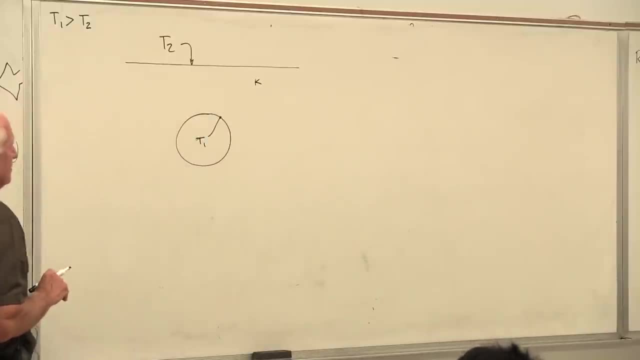 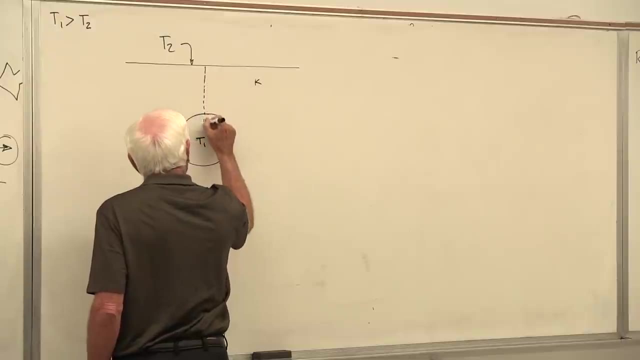 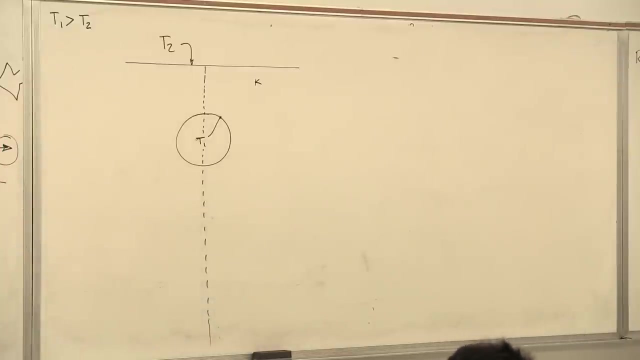 Okay. Number one rule: Look for lines of both geometric and thermal symmetry. Okay, Only one you got is one that goes right through the center of the sphere. There it is A line of symmetry: Geometric, Yes, Thermal Yes. 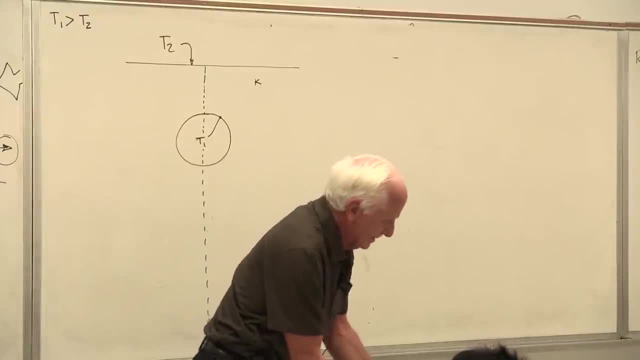 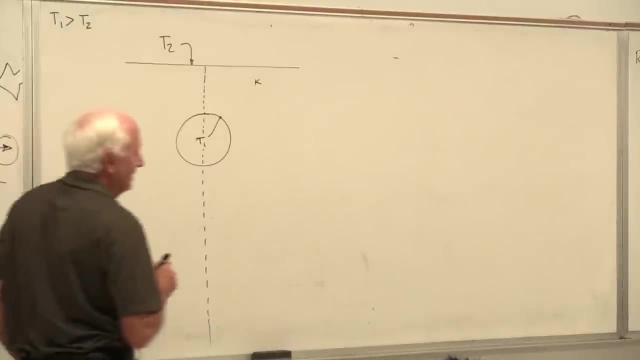 Okay, Got it That line. Rule number two. Rule two: That line is automatically an adiabat, A heat flow line. Yeah, that makes sense. Of course Heat leaves here and goes straight out the top of the soil surface there. 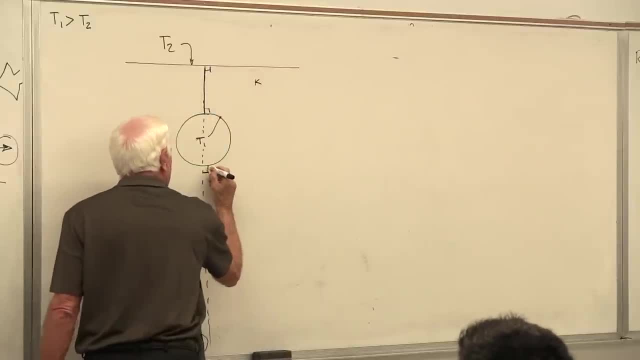 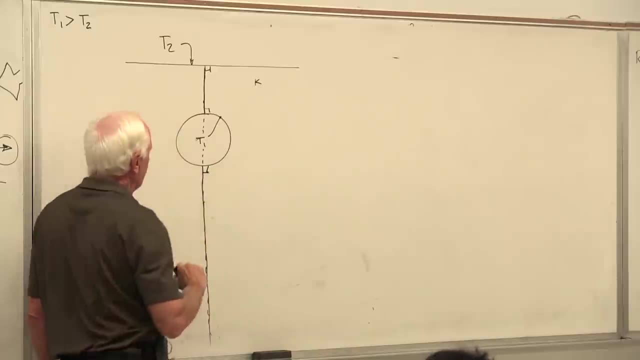 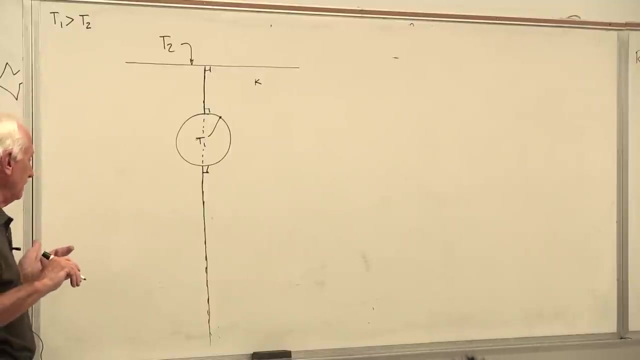 Right angle, Right angle Here This is a heat flow line Going straight down. Right angle. The rule says, no, I'm going to draw the heat flow because that makes I have some intuitive feel for that, But the heat that. 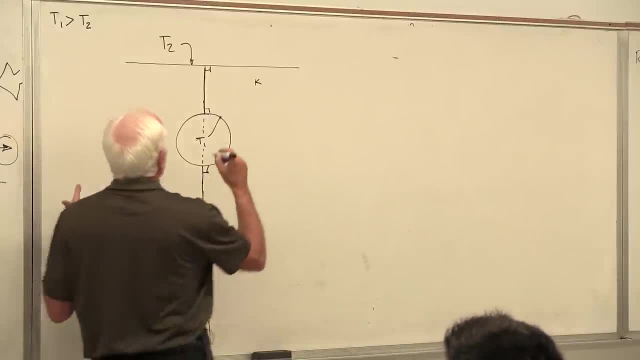 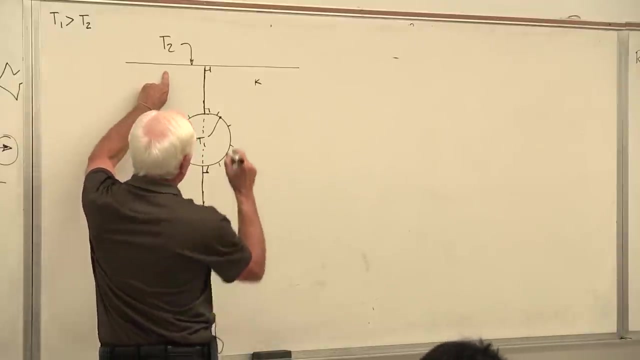 goes from T1 to T2, I know rule three or four- It leaves an isothermal surface at right angles. That's a rule. It leaves an isothermal boundary at right angles And when it gets to the other isothermal boundary it enters that boundary at. 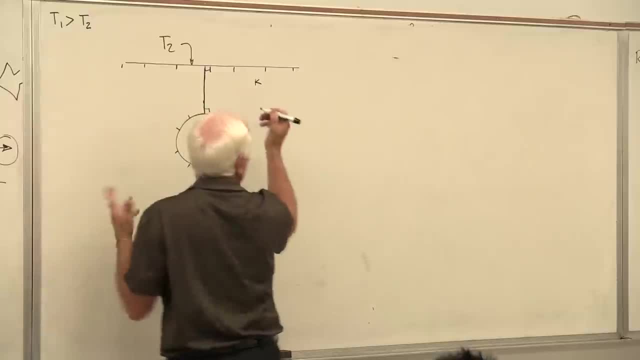 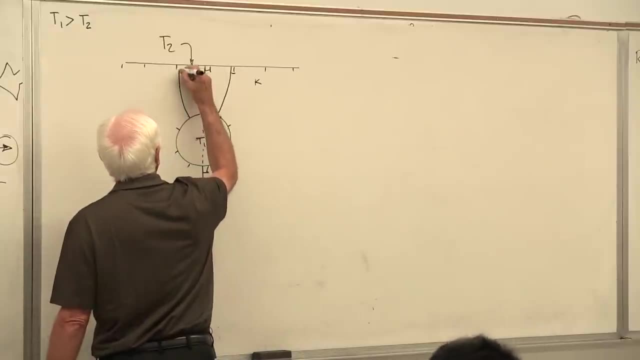 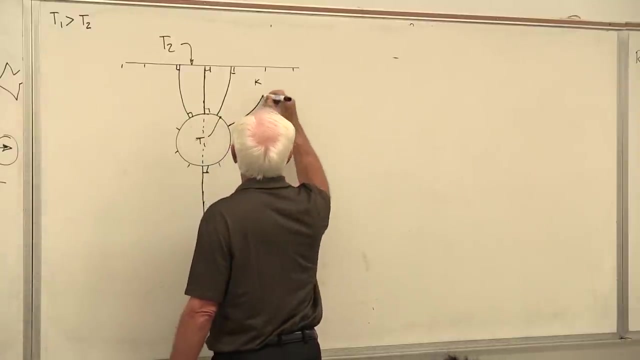 right angles. Okay, Take the easy one. I think heat leaves here and goes out here. Of course, Leaves here and goes out here. Yeah, Sure There. Okay, Keep going. Do the easy one first, though. Okay, It comes out here, Probably goes out there. Yeah, You got it. 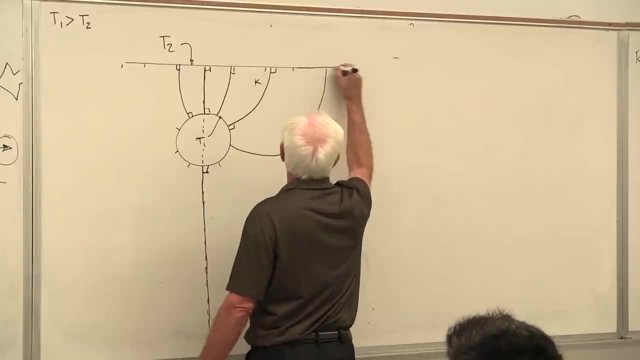 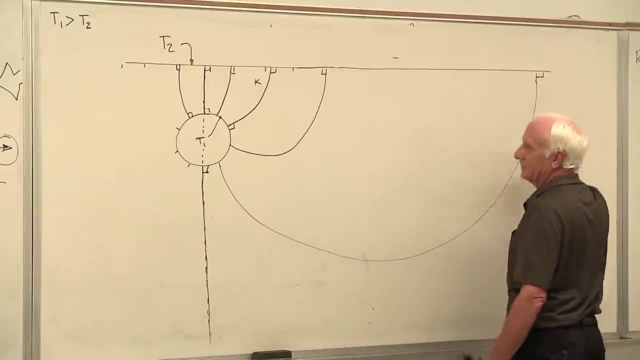 It leaves here and it probably comes out there. Yeah, You got it, And it leaves here and it might come out over here. Yeah, You're getting it now. Alright, There they are. You want to do the whole thing? Don't forget, It's symmetrical. You wouldn't have to, But I'll. 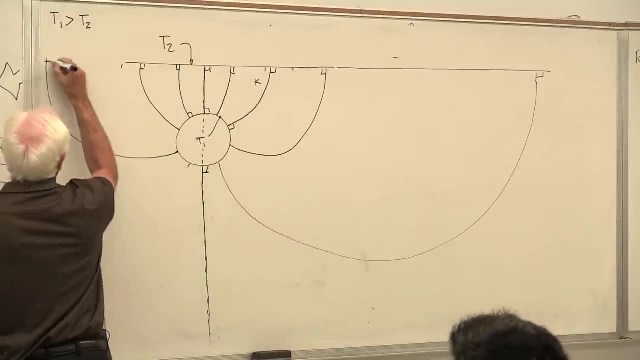 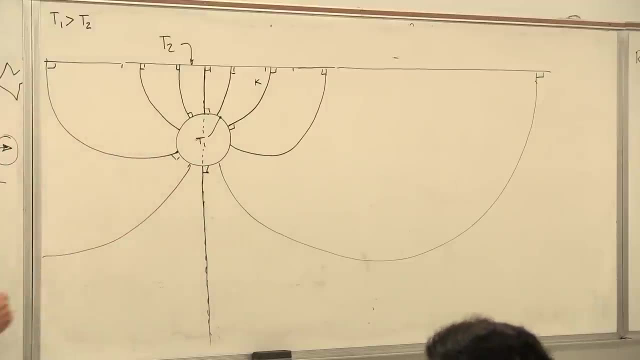 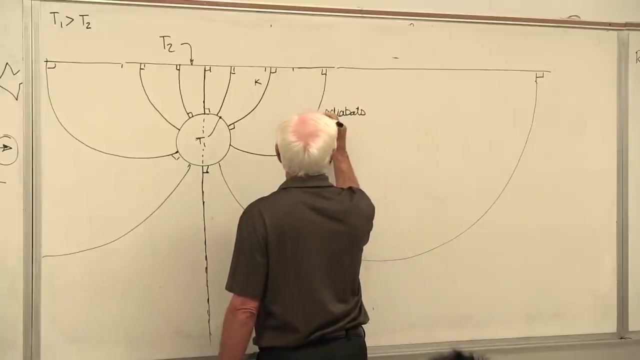 do the whole thing for you here. Comes out here, Goes over here. Okay, There they are. Comes out here, Goes way over there. Those are the easy ones. Label them. You see, if you don't label them, I don't want to guess which one's the adiabat. 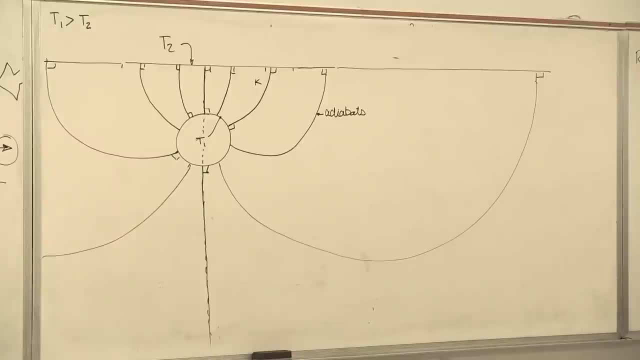 and which one's the isotherm. And I've given them something like this on an exam previously And some people they didn't label the lines And I got to know. I got to know which ones are the heat flow lines. 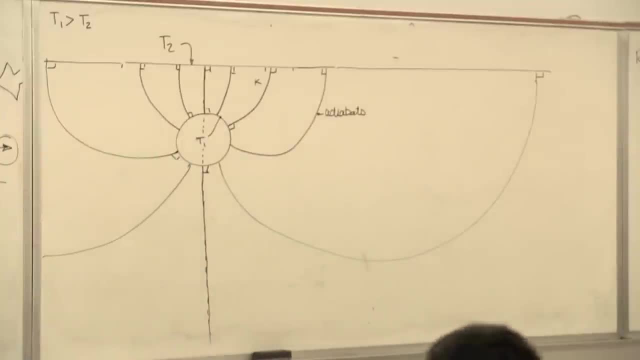 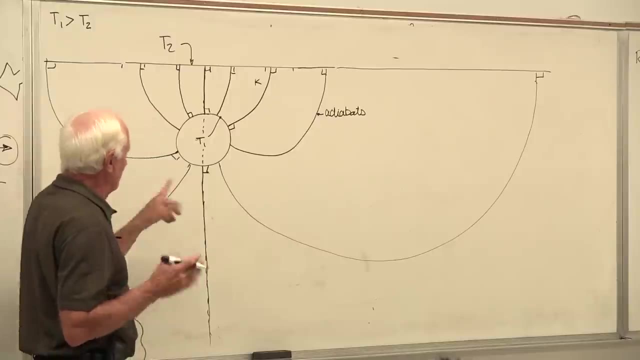 Which ones are the isotherms. So on a problem like this, label the lines for me. Okay, Now we're going to draw the isotherms. Take the easy one first. The first isotherm in this 2D diagram is a circle There. it is Guess what the next one is It's. 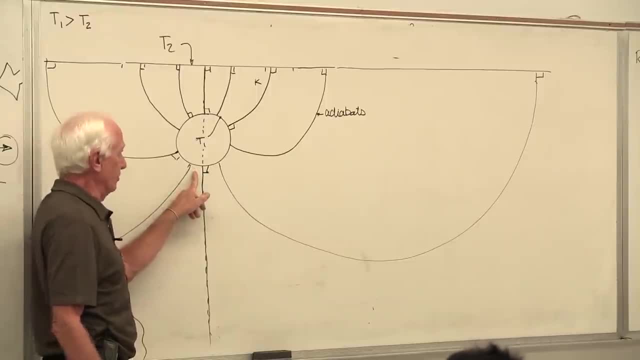 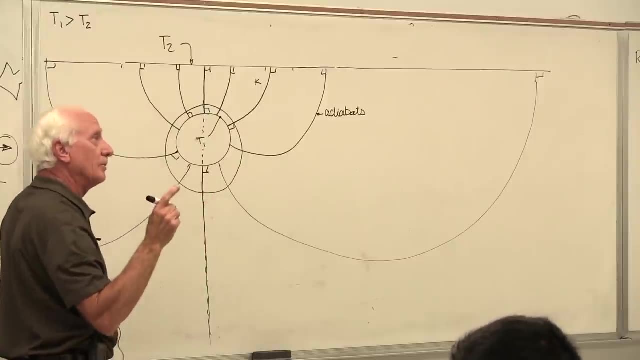 almost a circle. It's not a circle, It's almost a circle. I'll draw one And don't forget rule whatever it is: One, two, three, four, Three or four, Wherever the isotherms cross the adiabats. 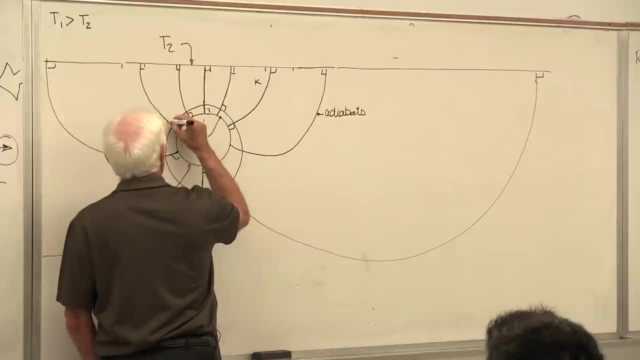 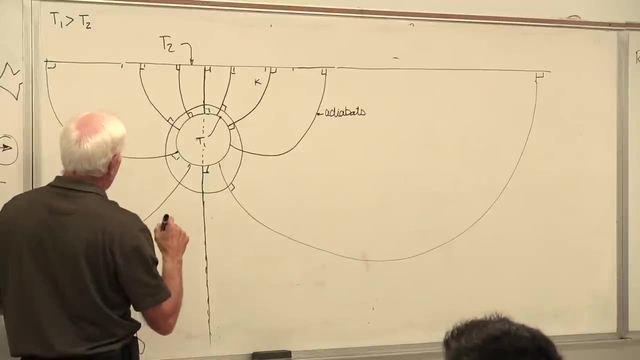 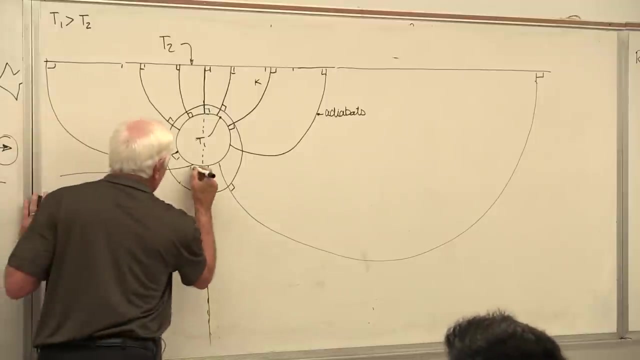 in the interior. they must always cross at right angles. Now, if you don't draw good, and maybe you said, this line here leaves here and goes out like that And I say, gee, that's not a right angle, I'll believe you if you do this. 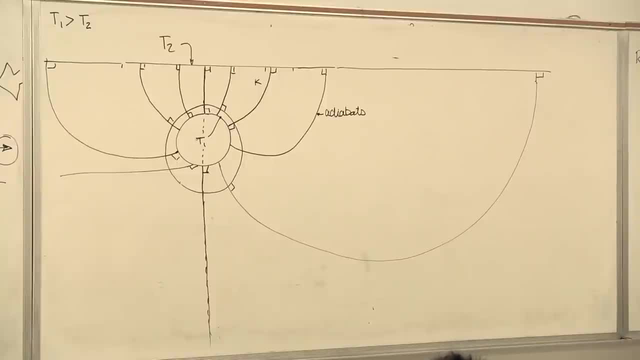 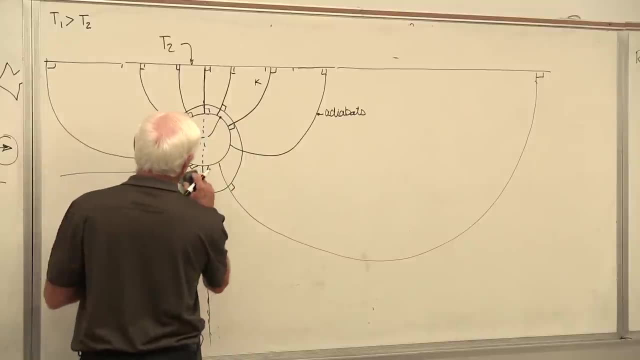 So help me give you partial credit by doing things like that. I know people aren't the best sketchers in the world, But at least show me you should be at a right angle, so I know what your thought is there, Okay, And then I'll believe you. Okay. So here we go again.